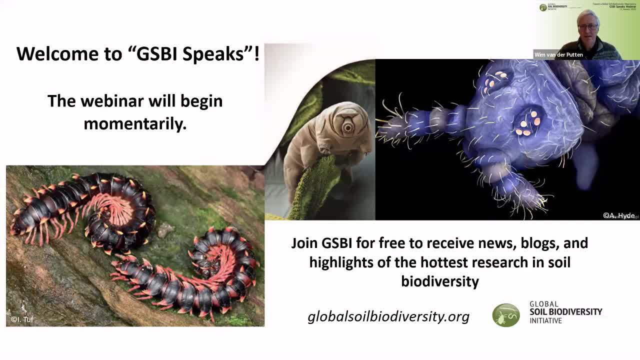 website of GSBI and there you can see all the meetings and the presentations. That also means that these presentations are being recorded, so you're warned for that. If you have questions, you can ask these questions in the Q&A and then they will be picked up and addressed. 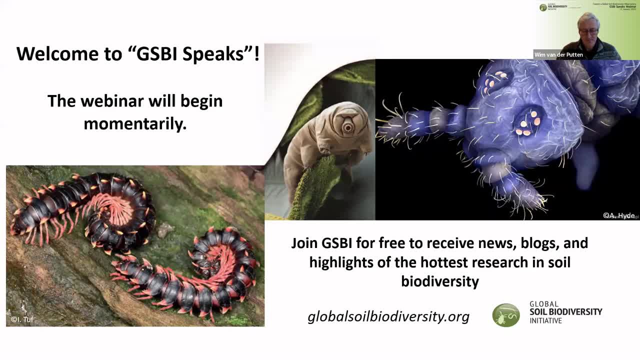 at the end of the introductions. First, I would like to show the speakers that we have gathered today. The first is Ronald Vargas, from FAO. Maybe you can show yourself, Ronald. Hello, Hi, William. Thank you, Hi, Ronald, Good to see you. The second speaker of today. 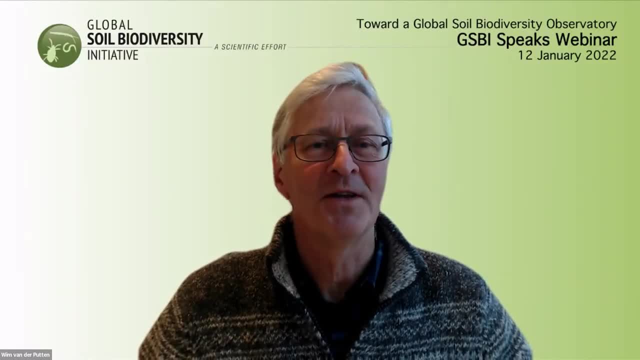 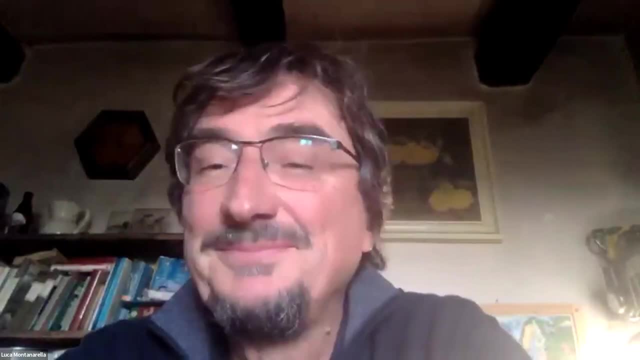 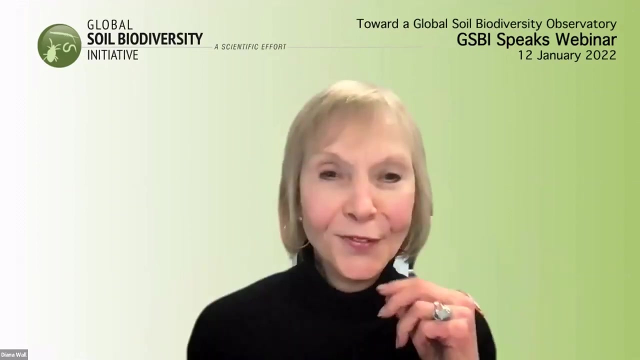 actually is the first speaker. Sorry, it is Luca Montanarella. He's from the European Commission. Hello, Good morning, Good afternoon, Hello Luca. Hello, Then the third speaker is Diana Wall of GSBI. Hi everyone, Hello Diana. 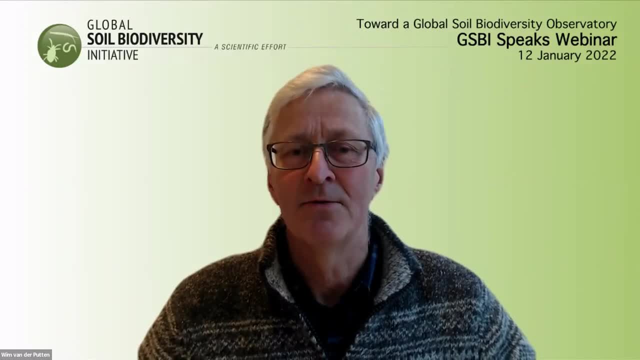 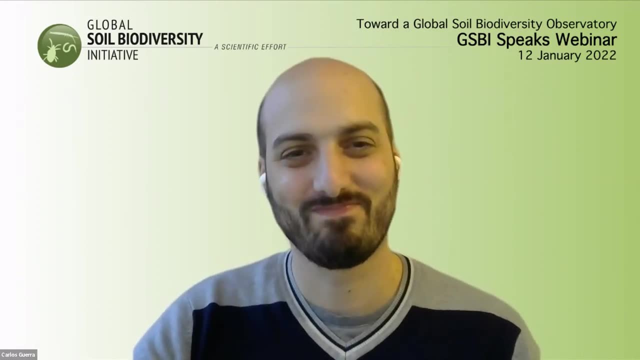 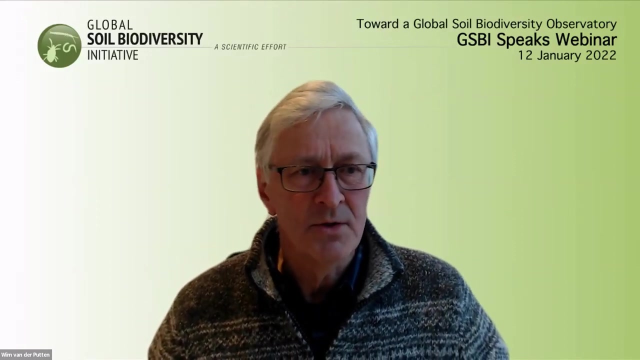 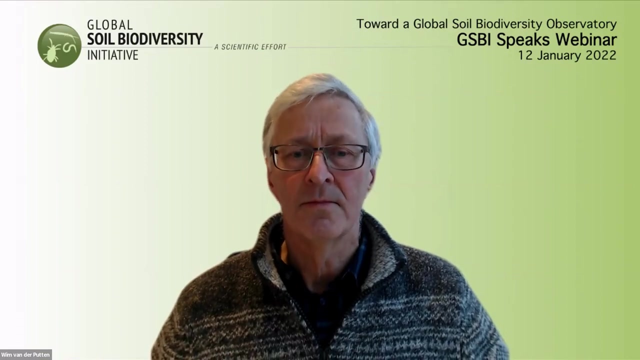 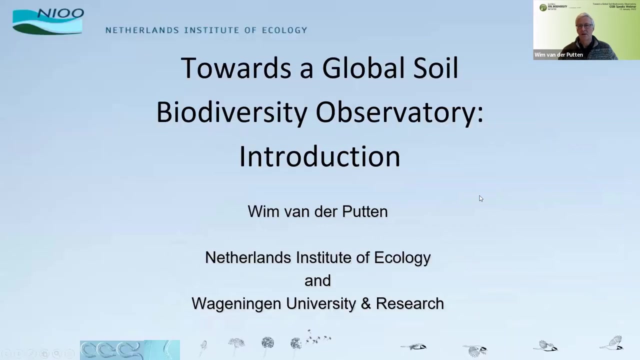 And the fourth speaker will be Carlos Guerra from Soilbomb iDiv in Germany. Hello, Hello. So I will start with an introduction to the theme And so you can switch off the camera, please. Okay, So if everything is fine, you can see my screen. If I don't get something, 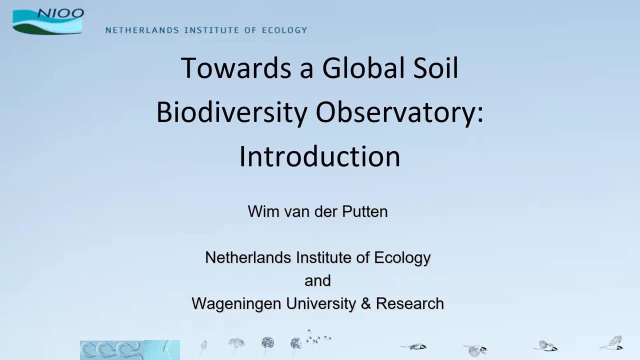 from Monica, then I'm starting: Looks good, Yep, Okay, Thank you. So today it's about Towards- a Global Soil Biodiversity Observatory, And I will introduce the theme to you briefly. All the introductions will be about 10 minutes and then we will just have ample time for. 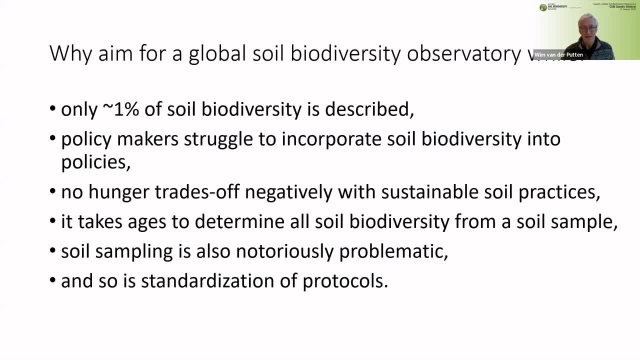 discussions and questions and answers. So the first thing actually to the first question to ask is: what do we aim for? And what we are aiming for, Is that not too early? So we aim for a Global Soil Biodiversity Observatory And we do. 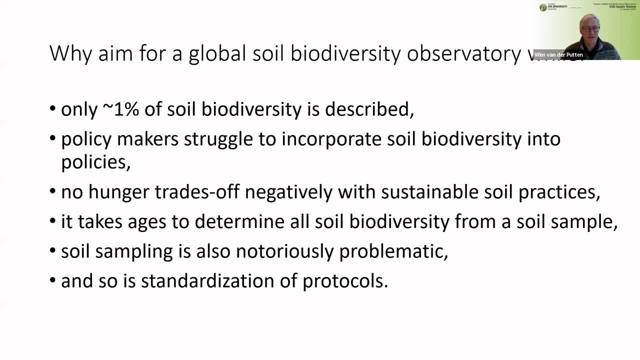 this, while only 1% of the soil biodiversity is described as we, as we can estimate. We also do this while only some of the soil biodiversity is described, as we know that no hunger trades off negatively with sustainable soil practices. We also do this while we know it takes ages to 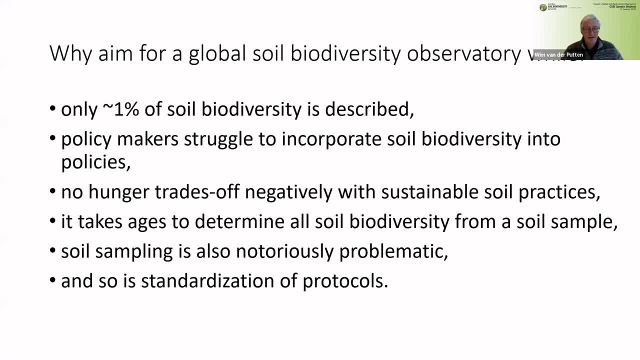 determine all soil biodiversity from a soil sample, And we know that soil sampling is also notoriously problematic, And so is the standardization of protocols. Well, you should have a lot of courage, while we have so much uncertainties, to start with the Global Soil Biodiversity Observatory. 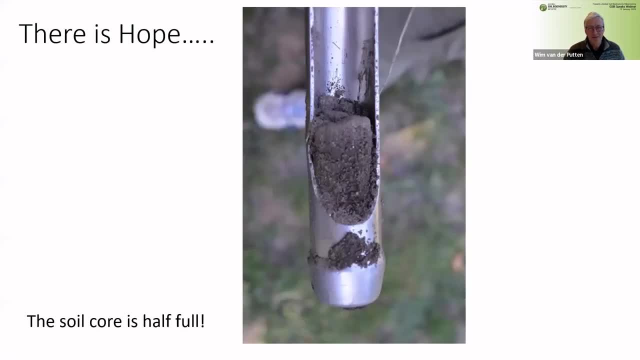 However, there's also hope, And I would like to make the comparison with a glass of water, which can be half full or half empty. We can also say the soil core is half full And actually, if we don't speak out as a soil and soil biodiversity community, then we will. 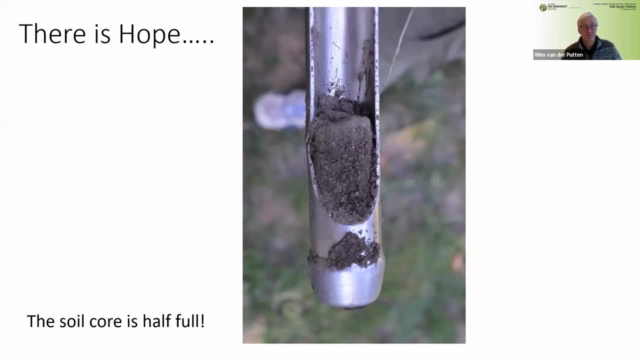 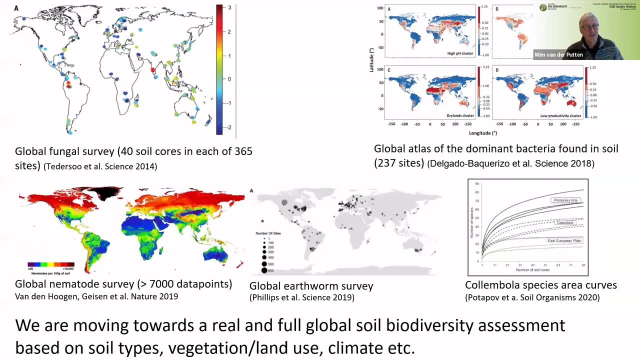 never be heard by the ones who make policy. So this is really important to tell the world what we know, And we know a lot. And if you have taken track of the literature, you have seen many papers coming or becoming published on global fungal diversity: atlas of the dominant bacteria. 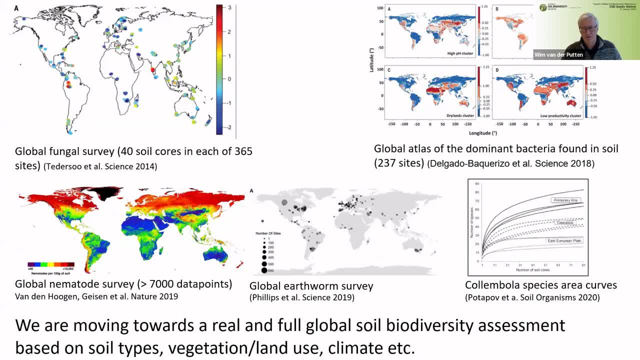 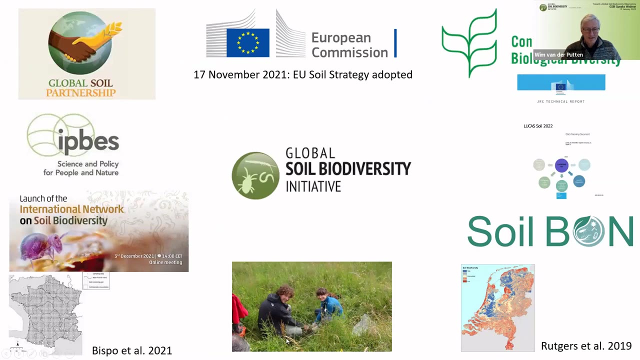 Global nematode diversity, earthworm surveys, columbulant species worldwide, And there are many other papers like this. So ecologists have started to try to publish information on soil biodiversity worldwide. So when you're just like here in the middle, you're a soil ecologist. 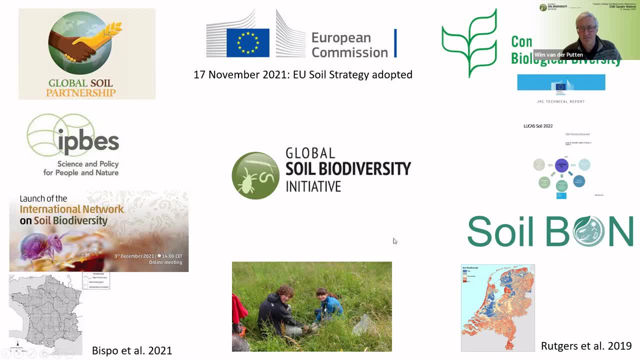 One other thing to be mentioned. I'm sorry. I'm sorry, But one of the things we've made very obviously aware of also is that there is a lot of activities going around. So we have national activities like the soil grid sampling in France or the Dutch soil. 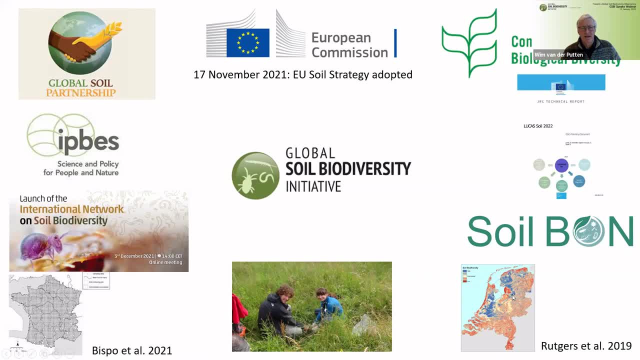 survey data. But there's not only that. there is also a soil bond sort of biodiversity observatory network. we have the Lucas soil sampling. Now it was an international network on soil biodiversity, on soil biodiversity assessment, which has been launched. but we also have IPBES. we have the 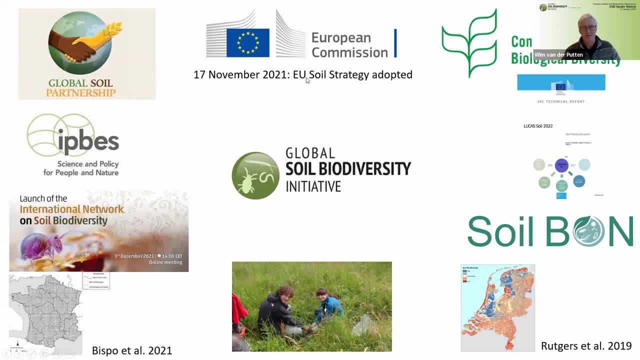 Global Soil Partnership. we have the European Commission that has adopted or started to adopt the EU soil strategy. we have the Convention on Biological Diversity. So just around us there is a lot of activities going on that helps and makes our data, or youth data, trickle up into strategies. 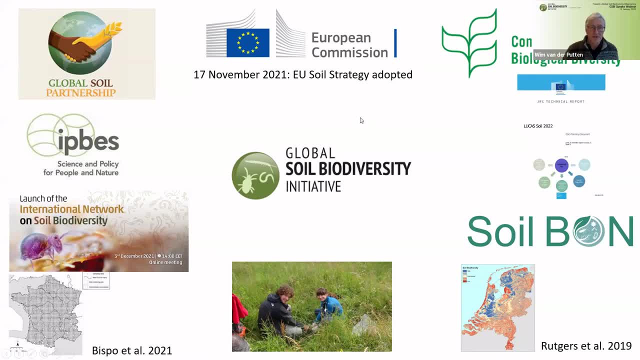 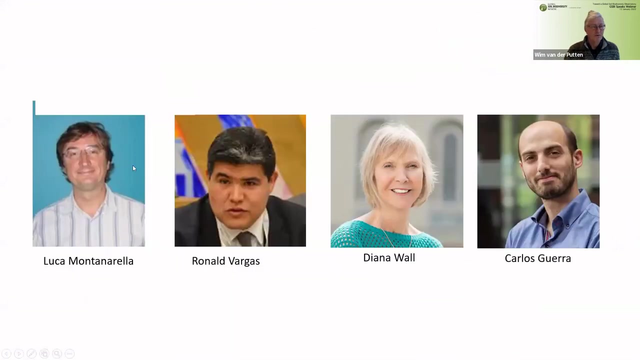 into policy- national, regional, global- And so today we are going to get some presentations from the various colleagues that have shown themselves already, which also can help you to know how your data are going to be taken up by policymakers. So the first speaker of today will be Luca Montanella. 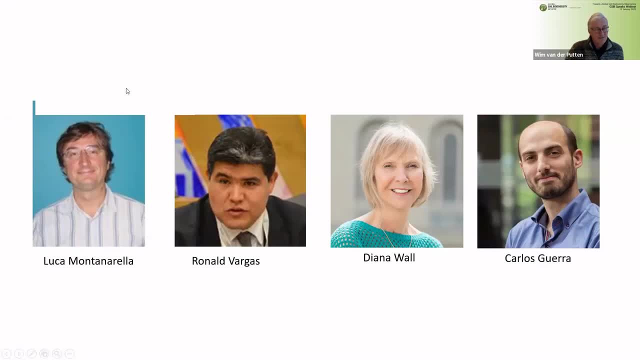 and he will speak about policies, EU policies, global policies. The second speaker: Ronald Farkas. he will bring us towards the global network of soil biodiversity observatories, Then Diana Wall will give the perspective from GSBI and what role GSBI plays, and Carlos Guerra. 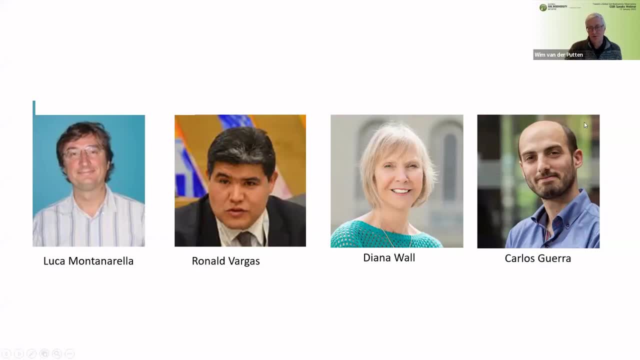 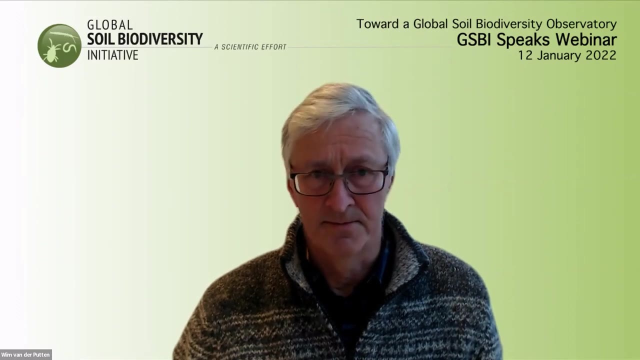 will bring us also to developing countries, and from a soil-borne perspective. So this is my introduction. Let's quickly move on to the speakers of today. Carlos Guerra, So, Luca, can I invite you to start sharing your screen? Sure, and thanks for the introduction, Wim. 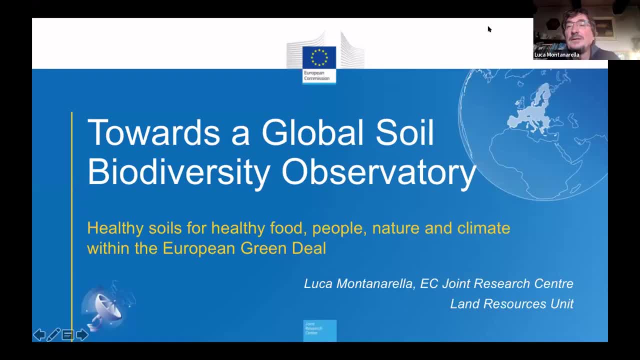 I hope everybody can hear me and can listen to me and can see my screen. So welcome again to this session, Welcome again to this seminar, As was introduced by Wim, very briefly introducing um from the european commission point of view, perspectives and from 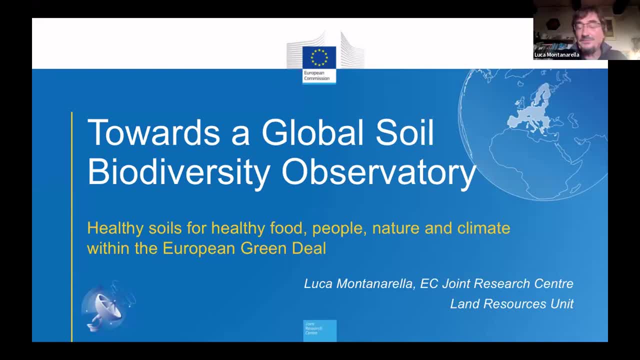 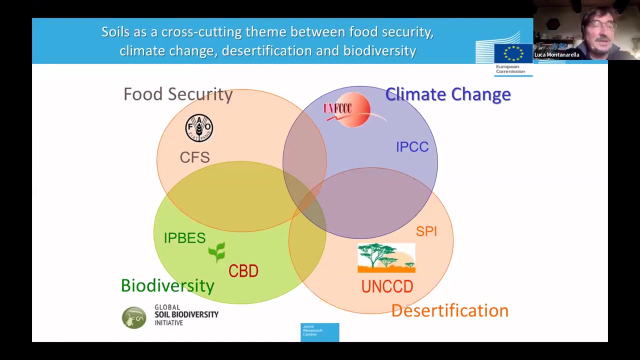 the work i'm doing at the joint research center, which is the science policy interface of the commission, where we are working within a team on some issues, how we have been getting to the stage of contributing to the establishment of such a global soil biodiversity observatory. so, um, let me uh move, uh, first to briefly introduce the context. uh, soils are very much cross-cutting. 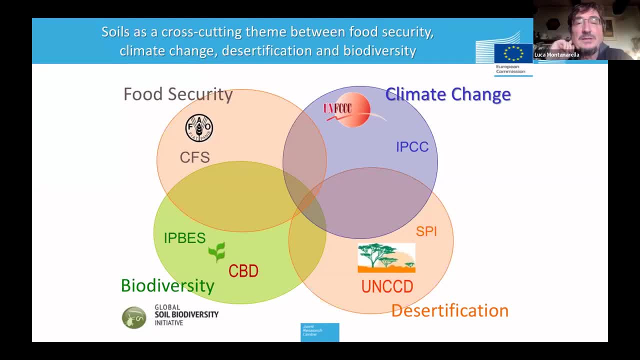 issue and being a cross-cutting issue means that there are many different policy areas that are relevant to soils. uh, that's why, actually, you uh quite have quite a difficulty in having a coherent policy approach, because different policy perspectives differ in policy context. addressing soilakis, a different angle. Certainly, food security is at the core of our concerns concerning soils. 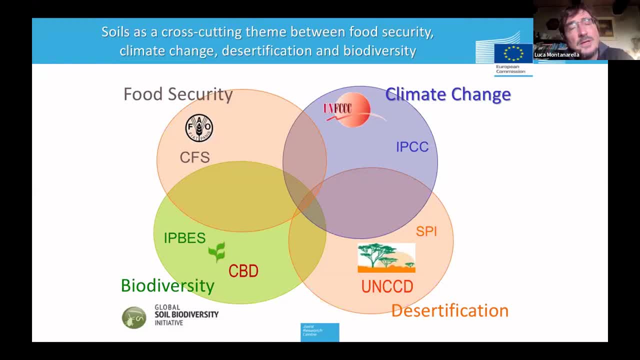 because soils are the basis of our food production. You may know that roughly 95 percent, according to FAO, of all our food is coming from soil-related production systems, mainly agricultural systems, But of course, soils are emerging at a very important topic, also within. 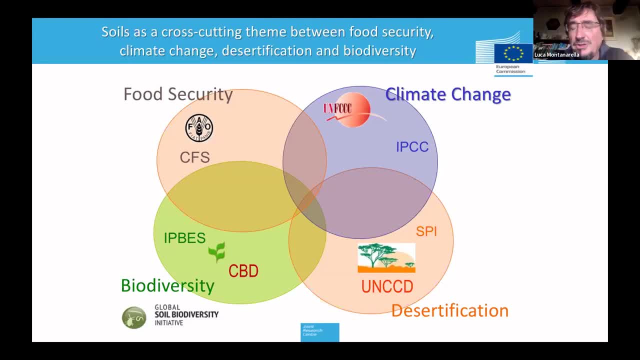 other contexts like, for example, climate change. You may know that soils are a major carbon sink and therefore soils are very relevant to the discussions around how to mitigate and to adapt to climate change. Soils are obviously very relevant also to desertification and to 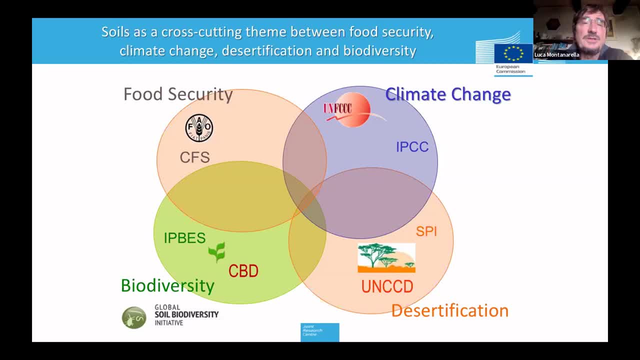 desertification and land degradation-related issues, and that's why soils at the very end are a cross-cutting issue across the various global and multilateral environmental agreements, like the climate change convention, the desertification convention and certainly also – and this is the 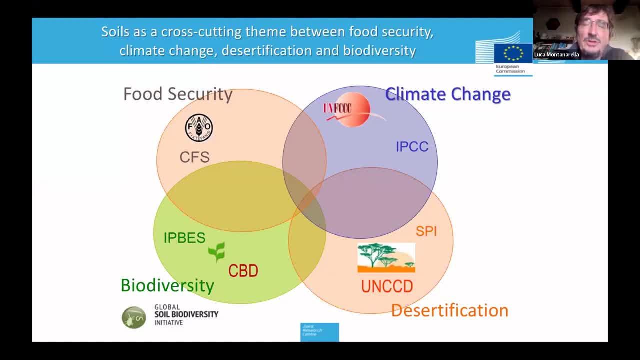 topic of today's presentation – the agreements with partner-states interested inwszy-seizzy via the the Biodiversity Convention. This is because soils are holding a very large pool of biodiversity. Much of the biodiversity, by the way, is little known and, as was just mentioned by Wim, still 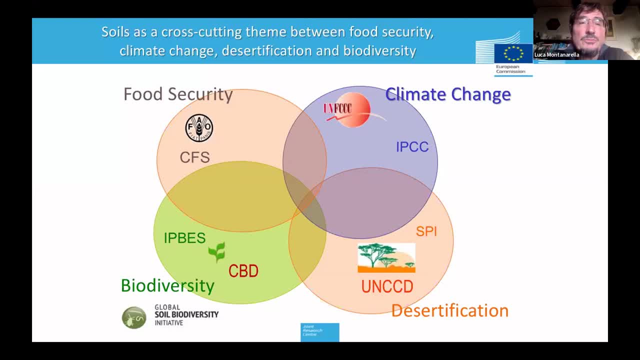 needs to be fully documented and fully described, also in taxonomic terms. Let me move on. sorry, Some years ago actually, and there certainly my colleague Ronald Vargas will tell you more. some years ago, in 2011,, we supported very much the establishment of a common framework that would put 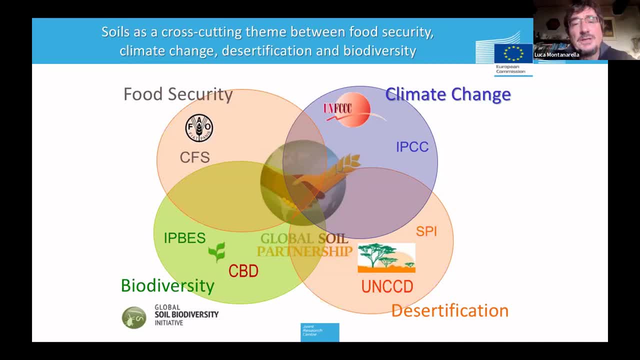 all this together into a common approach. This is the Global Soil Partnership that is very much also at the core of what we are trying to do now concerning the establishment of a Global Soil Biodiversity Observatory. The Global Soil Partnership had and has still the ambition. 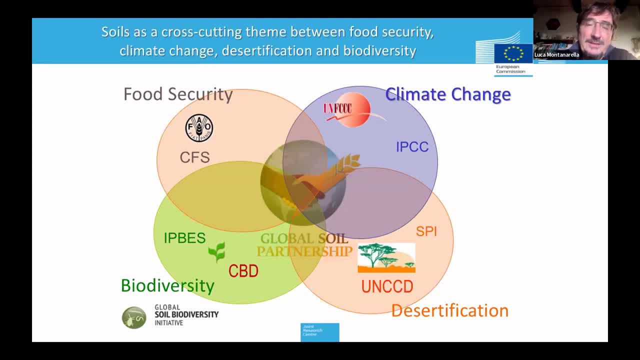 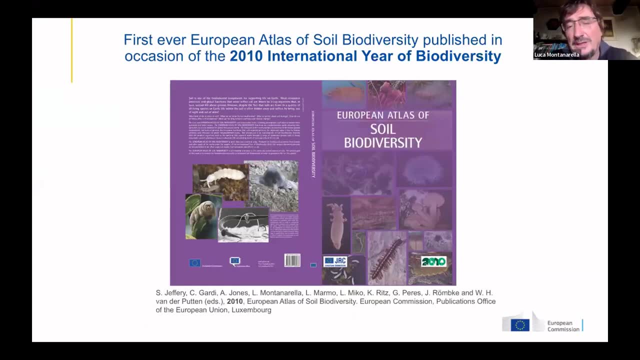 to be the connecting platform for addressing soils in a coherent way across the various policy areas that are relevant to soils. Now let me talk also a little bit about what we as commissioners have been doing on this topic. We started dealing with soil biodiversity actually in the early years. 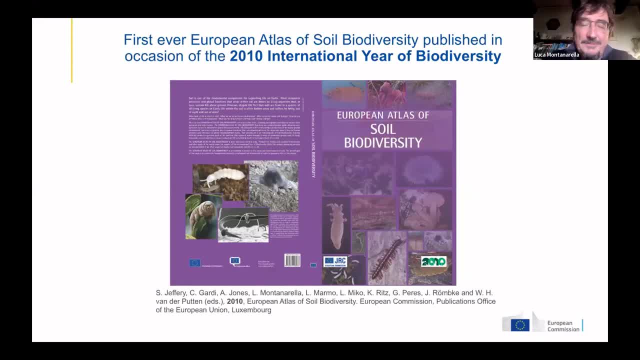 of this century. We started dealing with it particularly in preparation of the International Year of Biodiversity, 2010.. Where we compiled the first European Atlas of Soil Biodiversity that was presented as a contribution of the commission to the International Year and also was presented to the common conference of 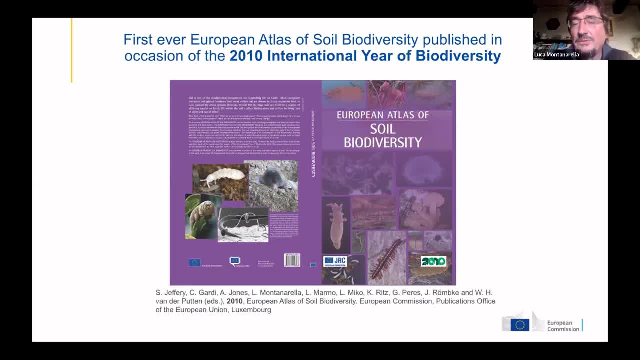 the parties of the CBD, of the Convention for Biodiversity in Nagoya. That was the starting point, actually, of understanding the biodiversity existing in European soils and but was also triggering a number of other initiatives that have been then leading to many of the things that we are discussing today in this webinar. One of the 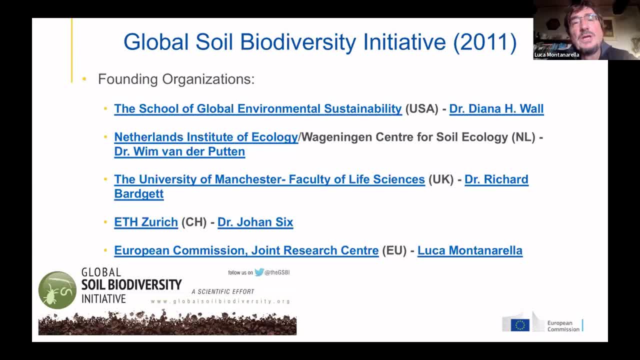 things that came after the publication of that Atlas was the founding of the Global Soil Biodiversity Initiative. I'm sure that later on Diana will tell you all the details about that. The commission was one of the founding organizations of that initiative that we think. 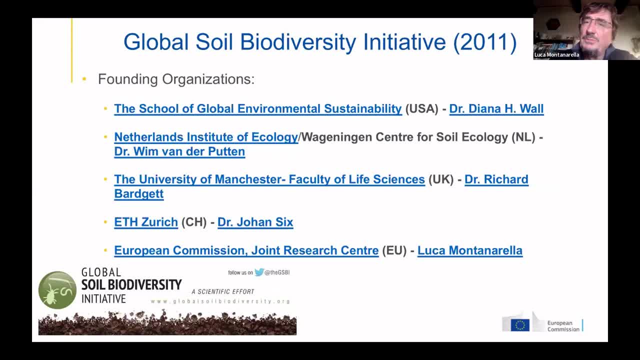 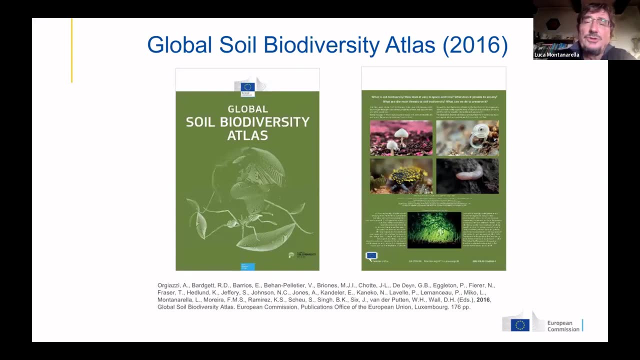 should be at the core of what we are doing concerning global soil biodiversity, and particularly should and is contributing quite importantly to this new idea of a Global Soil Biodiversity Observatory. Out of that also, then, we developed a global approach to assessing soil biodiversity at global scale, and actually that was the work that 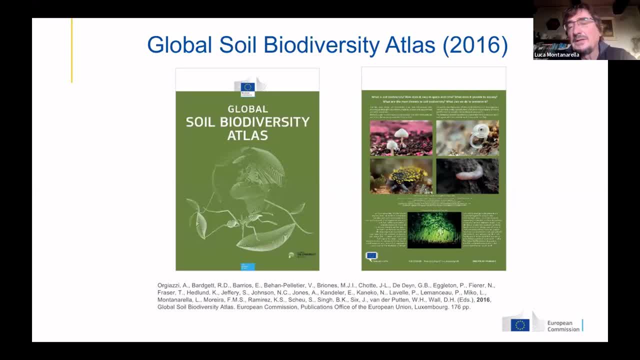 with the help of the Global Soil Biodiversity Initiative and many, many colleagues across all the continents in the world, has been leading to the publication in 2000, in 2016, of the first Global Soil Biodiversity Atlas as a publication of the European Commission. but 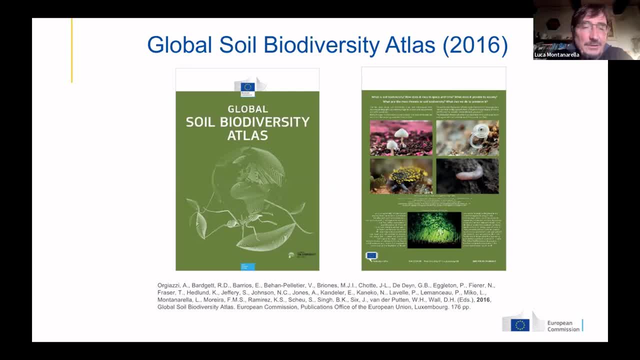 with the contribution of many of you- also many of you that are currently online and following this webinar- It was a huge collaborative effort all over the world in order to have a common understanding of the Global Soil Biodiversity Pool and also an understanding of what needs. 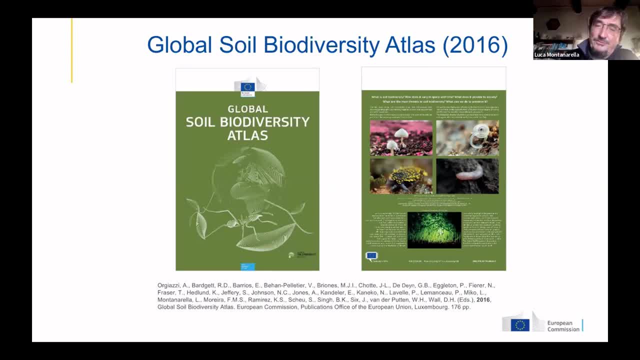 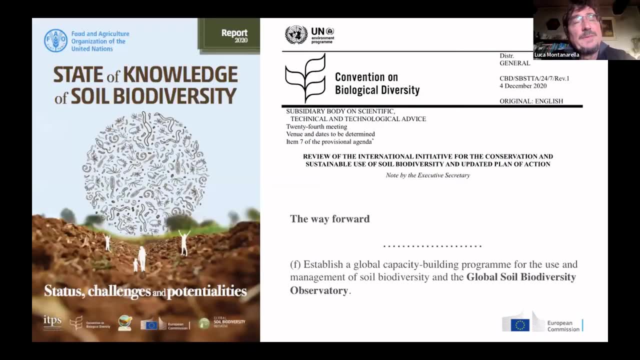 to be done in order to protect it and to further understand it. Now that has triggered a number of initiatives, including the need to have a higher level assessment of the state of knowledge on soil biodiversity. To that assessment, led by FAO, has been contributing many people, and 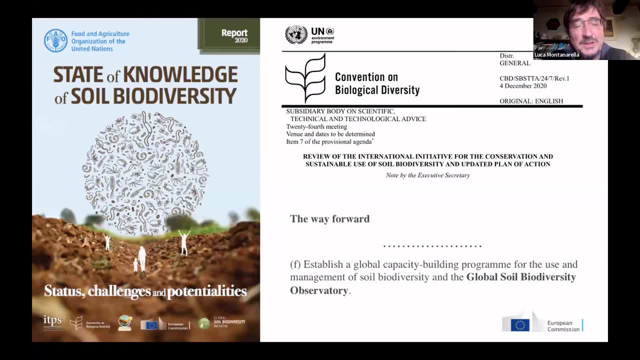 was released then in 2020, the report that you can download from the website of FAO, which is actually a reference for what we are trying to do now establishing the Global Soil Biodiversity Observatory. It's a reference because that report triggered a report by the Scientific Committee of the Biodiversity Convention. 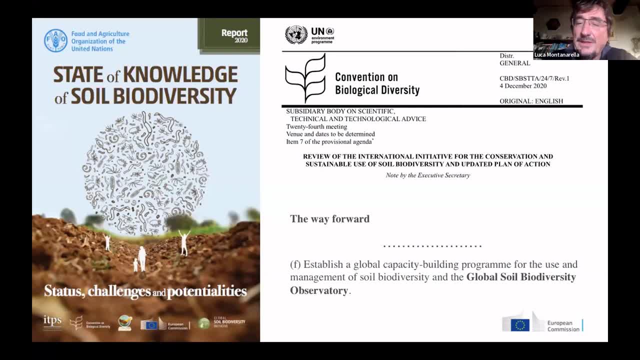 that has been recommending to establish a global capacity building program for the use and management of soil biodiversity and, particularly, has been recommending the establishment of a Global Soil Biodiversity Observatory, because that's an important type of recommendation. that's, of course, is building the basis, then, for further action from the side of the various stakeholders Following that. 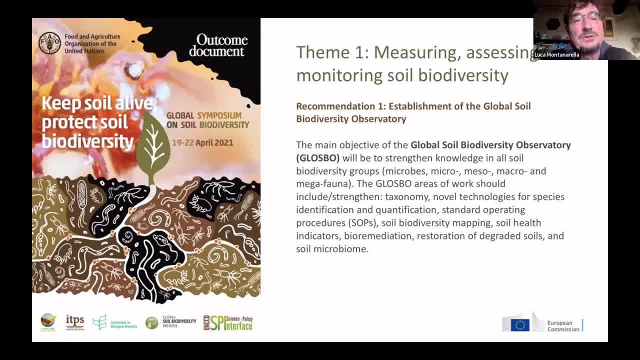 we had a quite important year last year, 2021, because FAO hosted in Rome- actually online as a virtual event due to the current pandemic situation- the first Global Symposium on Soil Biodiversity. That was a really turning point because out of that symposium, which 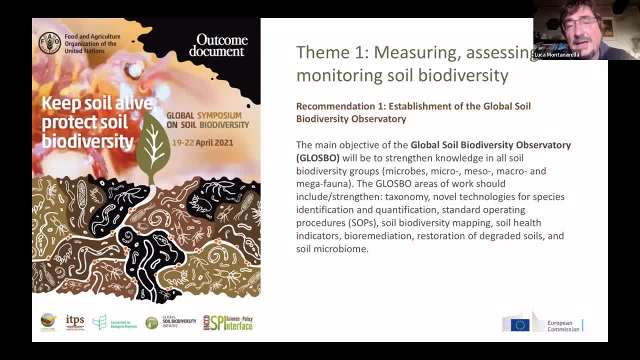 was open to everybody and where all the various stakeholders have been very actively participating, came out an outcome document that includes several quite important recommendations to policy makers, but also, in general, to all the various stakeholders, and one of the recommendations, actually the first one, is to establish a Global Soil Biodiversity Observatory. That recommendation is, of course, 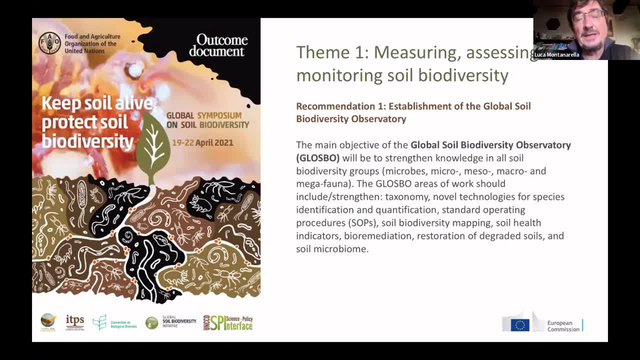 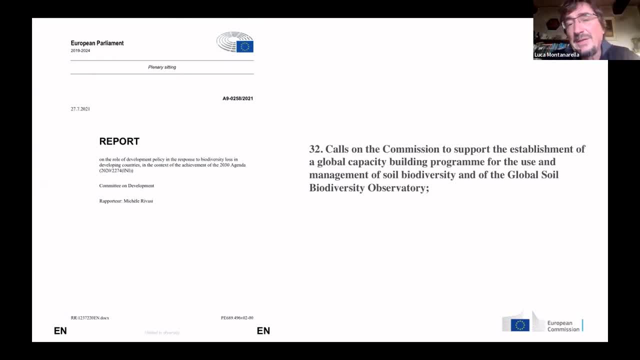 quite relevant and it was immediately taken up by several stakeholders and policy makers. particularly in the same year, in July, the European Parliament has been releasing a report, adopted a report in which it was calling on the Commission to support the establishment of a Global Capacity Building Program for the Use and Management of Soil Biodiversity and of the Global Soil Biodiversity. 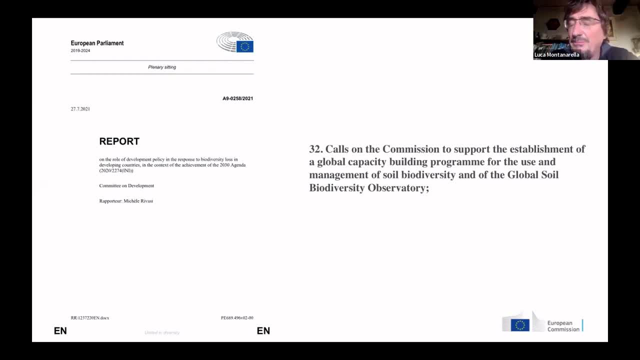 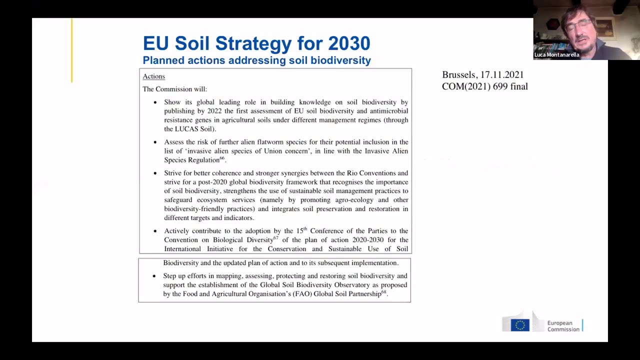 Observatory. So, having the European Parliament recommending us to do something, the Global Soil Biodiversity Observatory was further elaborated and inserted also in the more recent document from the side of the European Commission, which is and has been just mentioned also by Wim in the introduction, which is our new EU Soil Strategy for 2030.. As you know, as you may know, the European 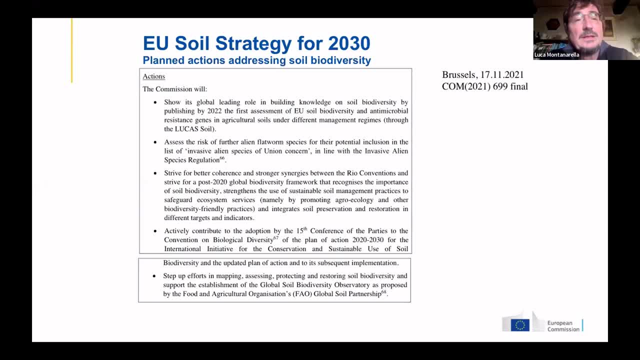 Commission has presented, on the 17th of November this last year, a new strategy. we already had one, which was a little bit outdated, presented in 2006.. In this new strategy, which has a target for 2030, we have outlined the various actions that the Commission is planning to do in the next. 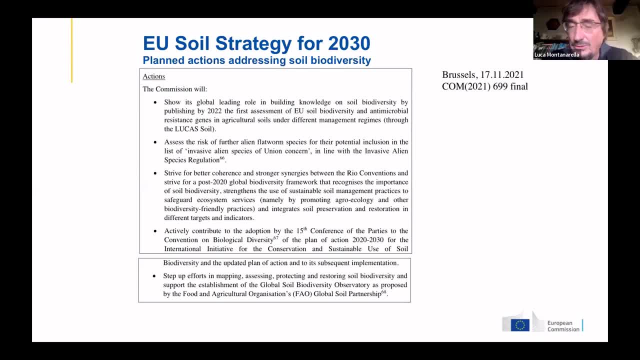 years in order to achieve sustainable soil management in the European Union, but also taking responsibility for what we do at global scale as well. I will not go through all the actions, of course, but just concerning the planned actions addressing soil biodiversity. the Commission is planning to demonstrate its global leading role in building 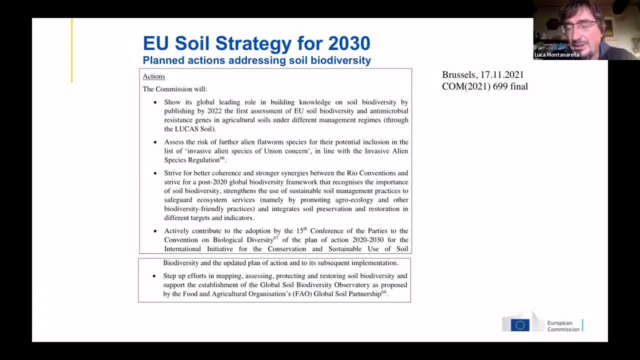 knowledge on soil biodiversity and that's by publishing in this year first assessment of EU soil biodiversity and several other activities that are related to that. but most importantly, I would like to mention that in the official final document of the soil strategy we have expressively mentioned that we intend to step up efforts in mapping, assessing, protecting 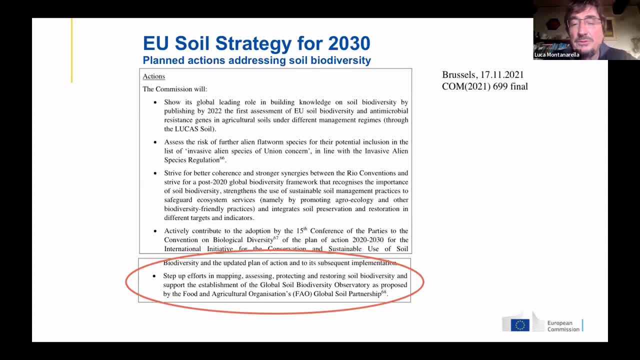 and restoring soil biodiversity and support the establishment of a global Soil Biodiversity Observatory, as proposed by the European Commission. information about the Global Soil Biodiversity Observatory State City日本 Now, but from Suomen University to Aso, get to and manage it. belangrijk to talk with you. our annual meeting of the European Commission, taking turn 104, is our official final document of the household strategy. We have expressively mentioned that we intent to step up efforts in mapping, assessing, processing, protecting and restoring soil biodiversity and support the establishment of a global soil biodiversity observatory, as proposed by the European Commission. 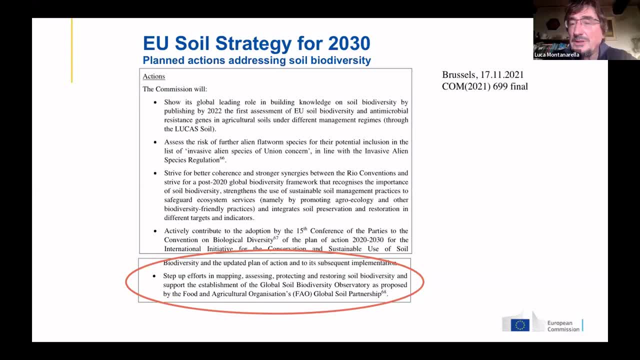 proposed by the food and agriculture organization within the global soil partnership. so that's the, let's say, the policy, the recommendation and the basis for further action, because out of this recommendation we would like now to make a move forward and see how we can concretely contribute. 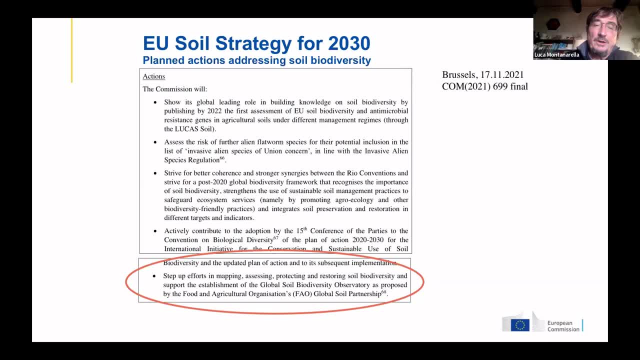 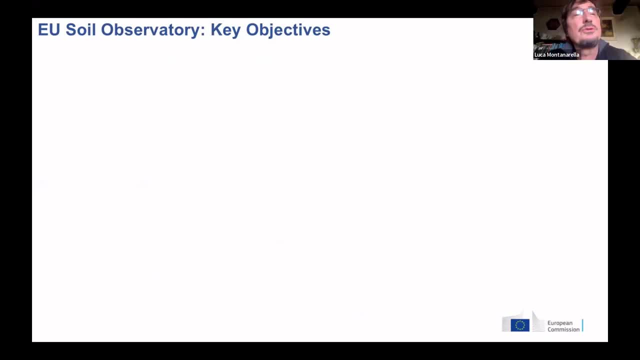 and help in establishing such an observatory. of course, we offer what we, what we know, and so you may know that last year we also introduced and established the eu soil observatory, or the european union soil observatory, and actually we offer that as a model, as a potential model. 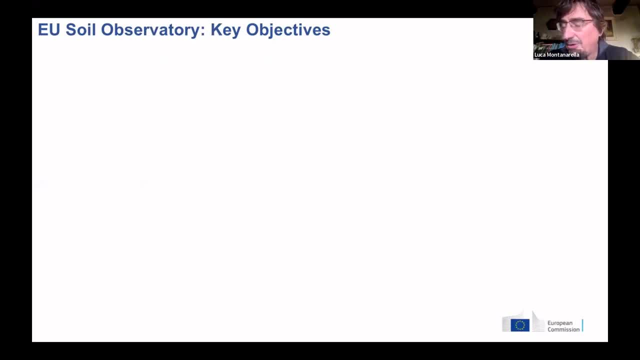 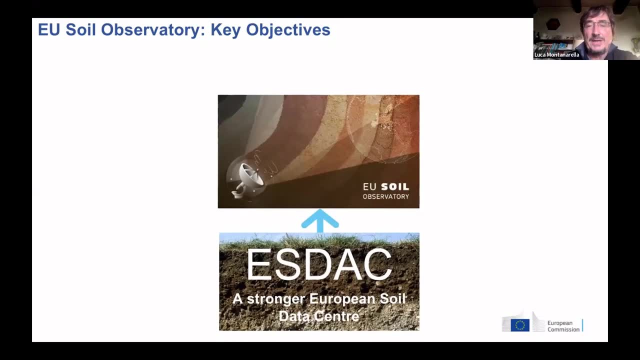 for how such an observatory may function and look like. for us and a soil observatory in the eu is essentially strengthening what we were already doing over the last 20 years, which is the collection of data in a harmonized way across the European Union has available already. 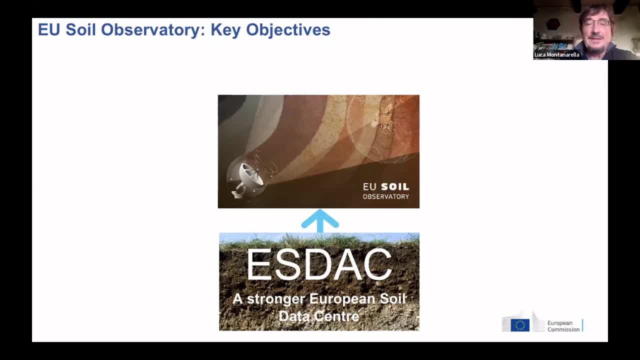 since a long time from the European Soil Data Center To strengthen that data flow. of course, the first crucial element is to have a stronger and more structured EU-wide soil monitoring system, And so a soil monitoring system is the basis for any observatory. 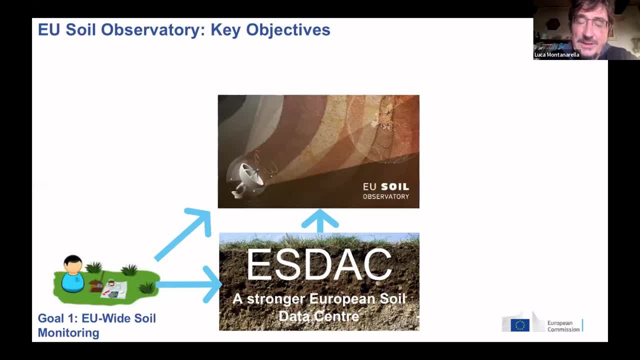 And this, in our view, should be also the basis for our discussions on how to organize a global soil biodiversity observatory. The second element is, of course, that data are not sufficient to help and to steer what is happening on soils from the policymaking side. 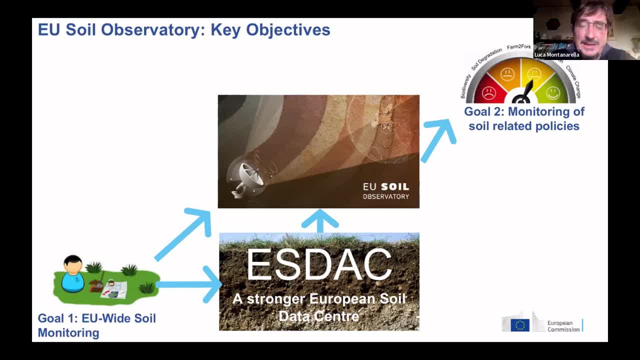 You need to translate this data into indicators that are relevant for the various decisions to be taken on the land management and on the soil management practices. So you need a dashboard of indicators that is monitoring how we are doing the soil management practices Concerning soil-related policies. 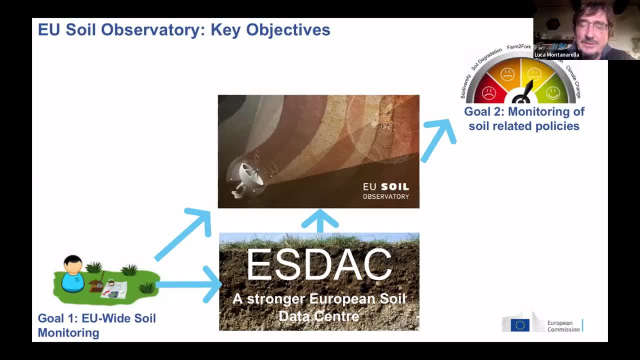 how are we doing in implementing what we are planning to do and how this is really reflected then in a positive outcome concerning the properties and the condition of soils in Europe And, of course, in the case of the global observatory, at global scale. We also think an observatory should keep a window open. 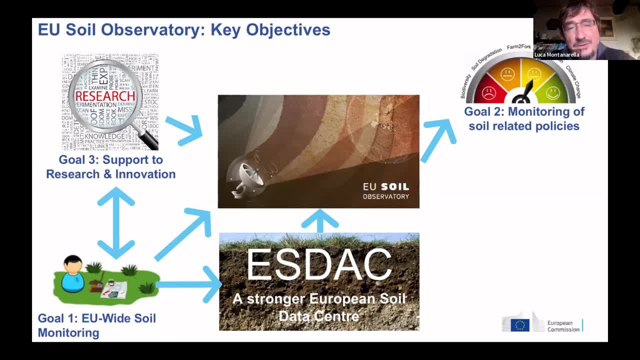 and should continue to support top-level research. I think And we think that research and innovation in an observatory has a role to play, because we need to be at the forefront of the scientific knowledge. An observatory must be based on the most updated scientific knowledge. 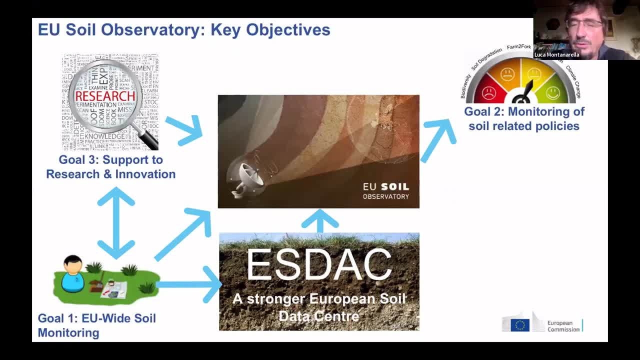 And that's why support to research and innovation is an important goal of the European Soil Observatory. And finally, let me mention something that we consider quite crucial: We cannot do monitoring. We cannot have monitoring of the soil, We cannot have an observatory. 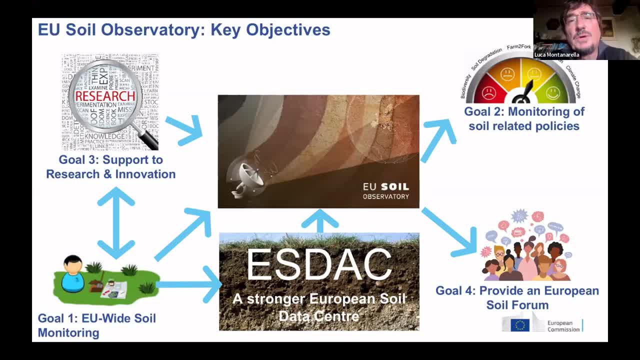 if we don't have an open platform for discussing what we monitor and what we measure with all stakeholders, And that's why an open stakeholder forum that we call the European Soil Forum is crucial to us in order to assure that everybody is on board. 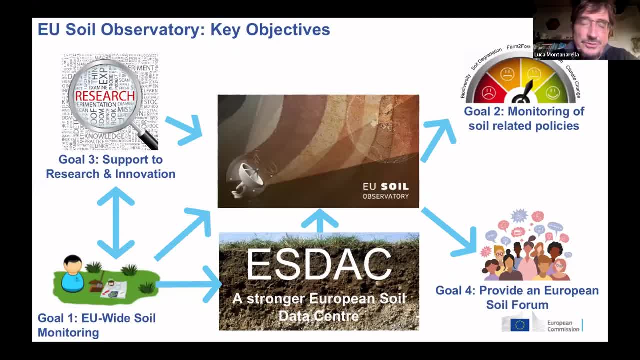 that everybody has the possibility to express his vision concerning how we should operate such an observatory at EU scale, And we think that that could be a successful model also to be replicated at global scale, But this, of course, needs to be further discussed. 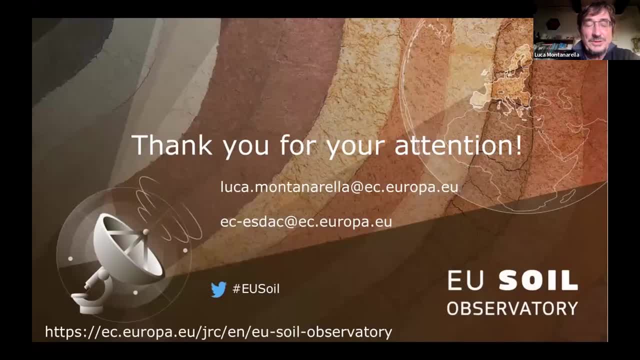 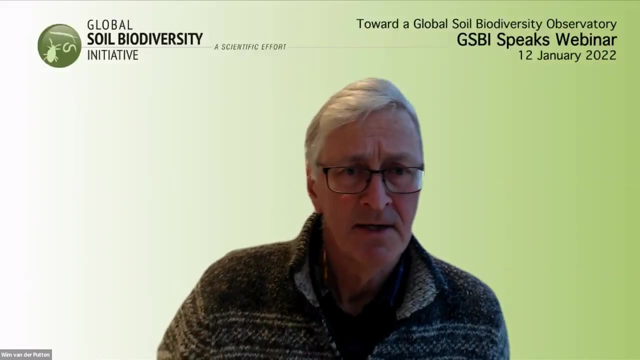 And hopefully also this webinar will allow such a discussion. So thanks again for your attention And I'm more than happy to reply to any questions later on or to further discuss all this. Thank you very much. Thank you, Luca. In the Netherlands we have a saying. 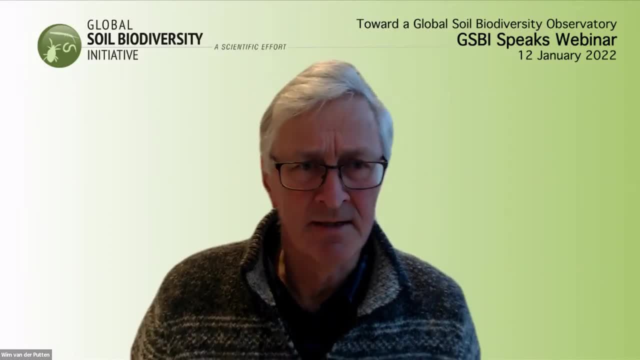 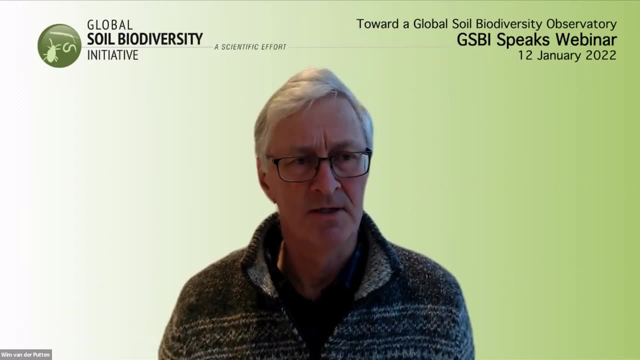 that Aachen and Cologne have not been built on the same day, And I think that you have nicely explained how much time it takes to get everything in place, to have a good soil strategy and then to roll it out. So you mentioned two decades. 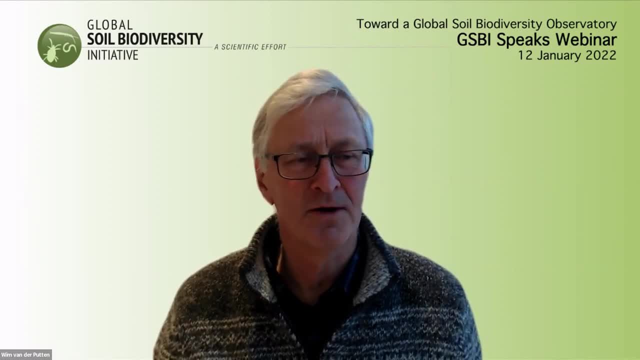 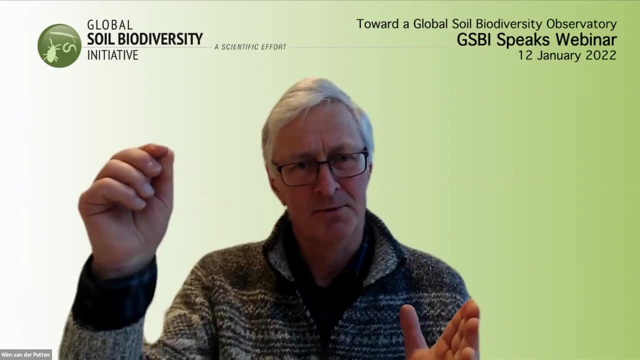 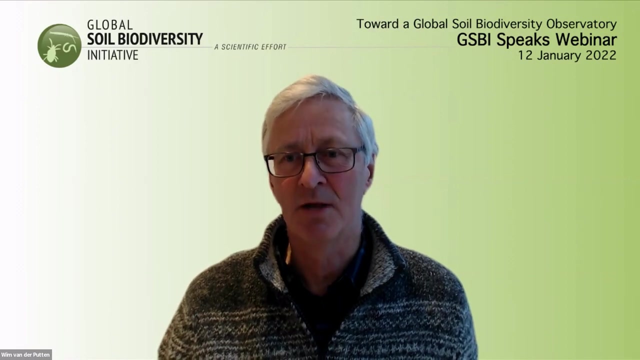 It's very enlightening for everybody, I think, to see how policy works, So how much it takes time to go from your soil core up to Brussels or Washington or Rome or wherever. Thank you. So the next speaker is Ronald Bargas. 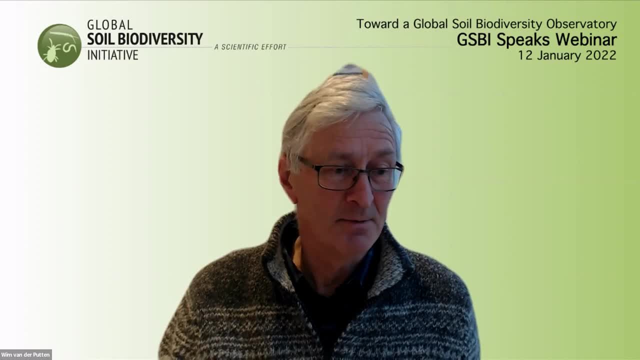 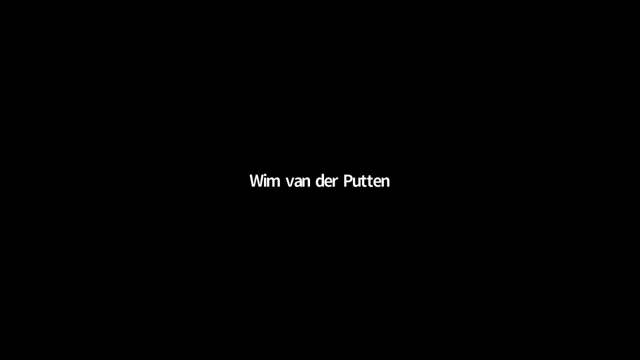 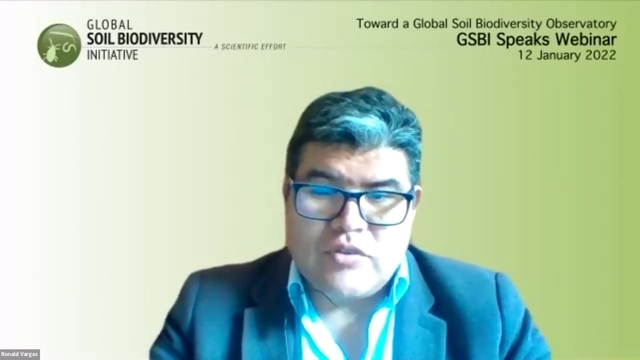 And he is from Rome, from FAO, And he will bring us into the conversation And he's going to tell us a little bit about this global observatory. Thank you very much, Wim. I will well. Luca basically explained most of the things. 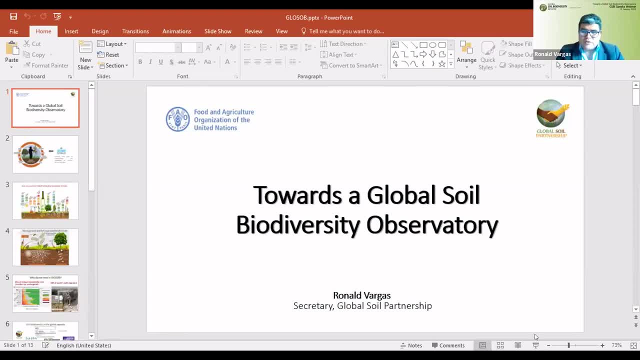 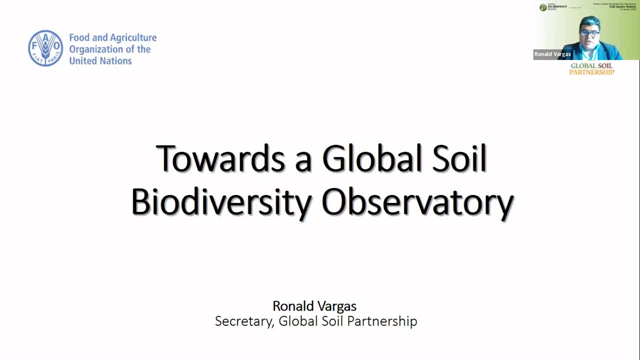 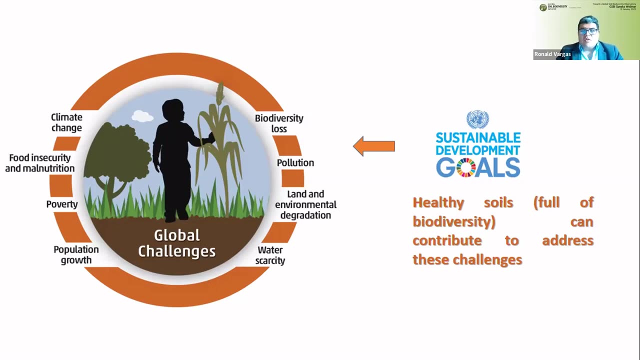 that I was going to say, So it's easier. now I will try to focus on some details about what we are trying to do together. So, basically, we are aiming to establish a new biodiversity observatory in order to contribute to address the global challenges. 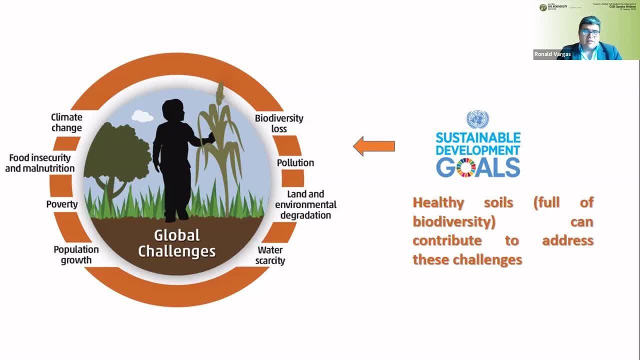 that we are facing. I know that here we are in the community with soil biodiversity experts, And biodiversity loss is one of those great challenges we are currently facing. However, there are many others And all of them are interconnected, And they are interconnected through one interface. 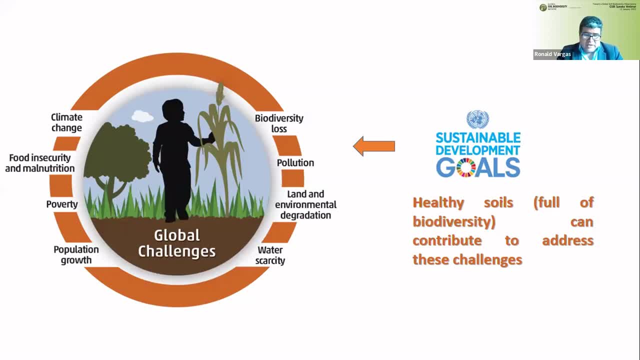 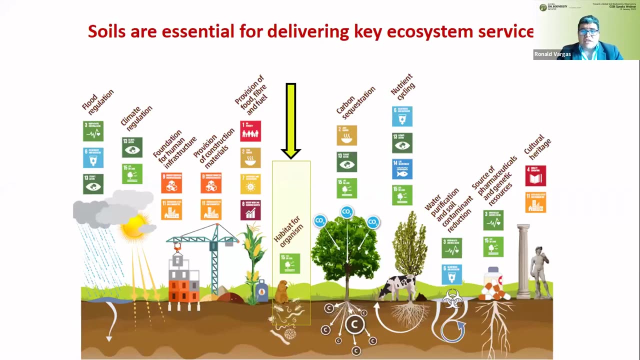 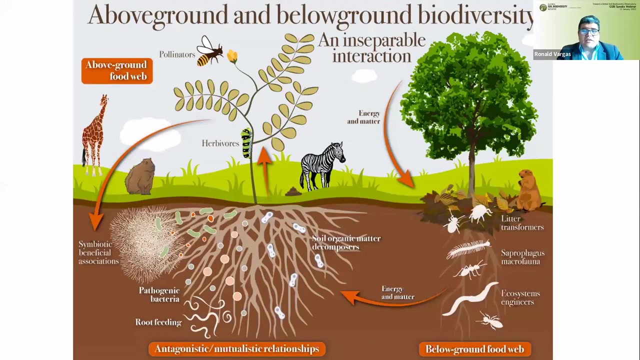 which is soils, And we are firmly Sure that healthy soils, of course, with a lot of biodiversity, can contribute to address these challenges, so that we keep ensuring the provision of key ecosystem services that are fundamental for life on Earth. That is really what it motivates us all. 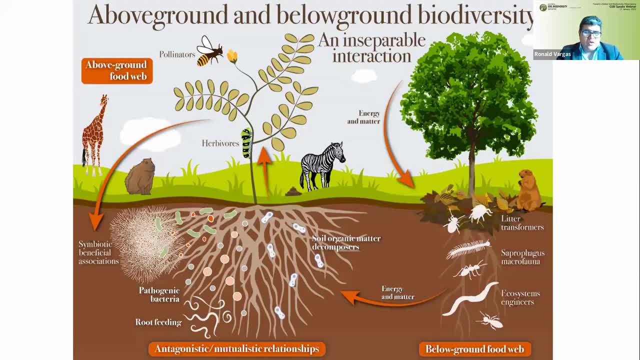 But something very important, that we are trying to inform the different And Venues, And particularly the decision makers, Because when talking about the biodiversity loss, we tend- and especially general public tend- to talk about what we can see, But we fundamentally forget about what is below our feet. 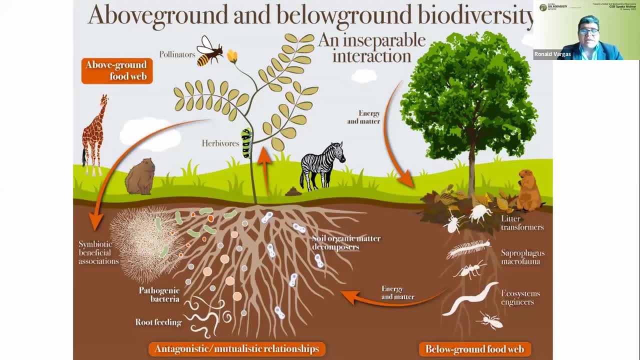 And that's the biodiversity in our soil. So we are trying to make it very clear that the two cannot separated, cannot be separated and should be addressed together. Otherwise, we are really not addressing the biodiversity loss. So that is something that we want to highlight. 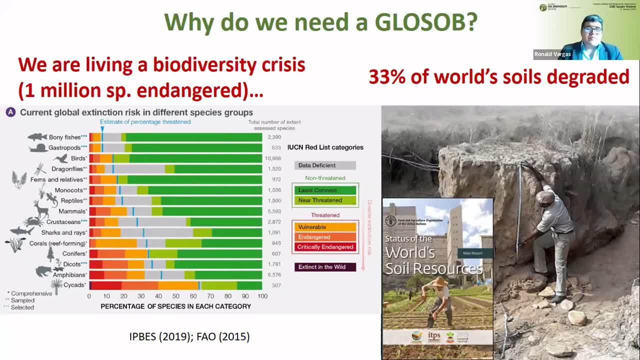 Because there is a lot of, let's say, concern about the biodiversity loss, But we are forgetting a fundamental piece, that is, soils, soil, biodiversity, And currently we are facing one big challenge in our sector, which is that soils Are getting degraded. 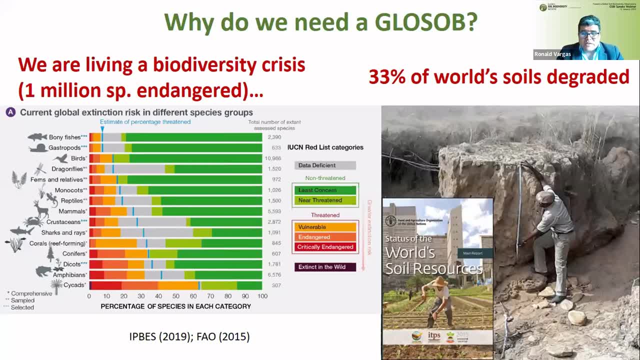 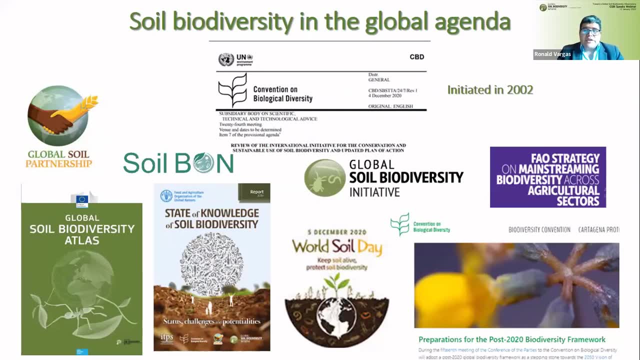 And that of course, has an impact not only on soil biodiversity but on the overall soil health. A lot of, let's say, work has been done already in soil biodiversity, And we have been trying to position soil biodiversity in the global agenda. 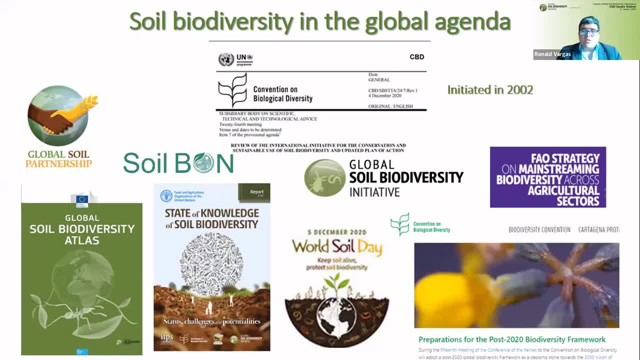 And we were not the first ones to do this. In 2002,, the International Initiative for the Conservation and Sustainable Use of Soil Biodiversity was Established under the Convention on Biological Biodiversity, And some work has been done. However, it didn't reach the level in which soil biodiversity 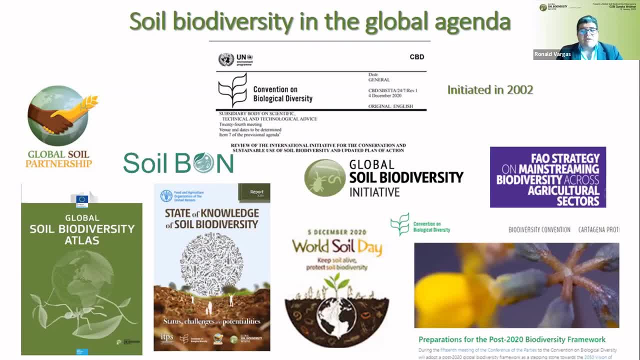 could be considered. Luckily, there has been a number of initiatives coming up- And Luke already mentioned most of them- that brought soil biodiversity again and give it an impulse, that now soil biodiversity is considered an important, important piece. But we didn't reach the limit because there 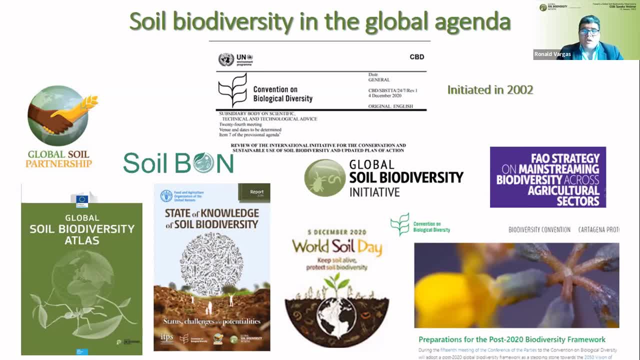 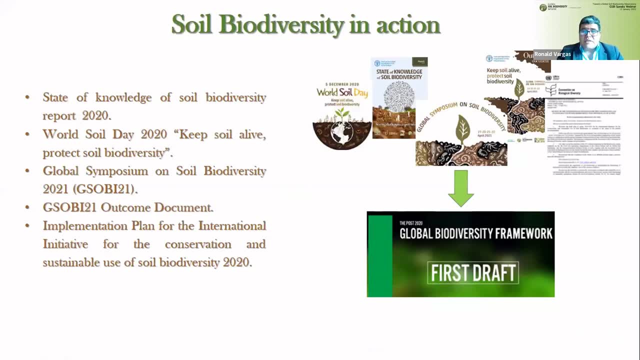 is still a lot of work to be done in order to really make soil biodiversity a very important piece of all the policy developments and actions globally. We have been doing some work. Luca mentioned most of it, And I believe that now we have the basis for moving forward. 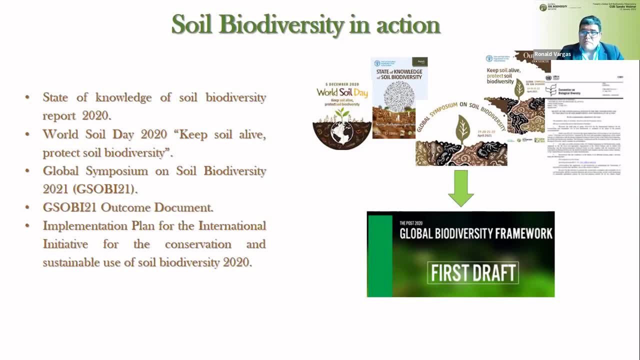 So that research And I believe that now we have the basis for moving forward, So that research, And I believe that now we have the basis for moving forward, So that research Is a strength, More investment is there, but also that all countries around the world. 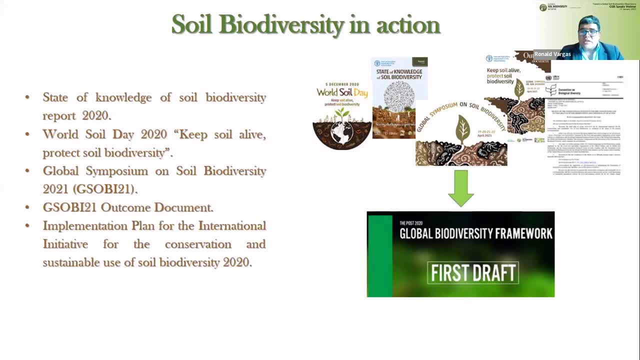 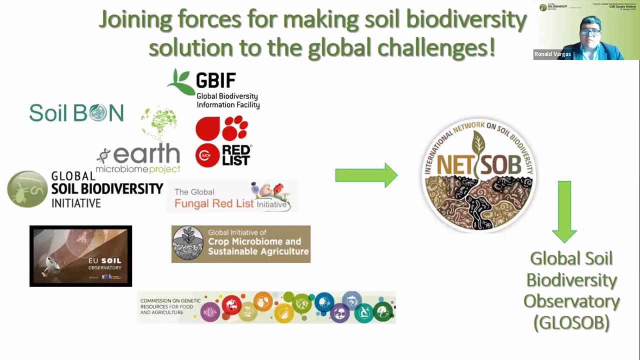 can be working on soil biodiversity, not only to understand what they have in terms of biodiversity there, but in using soil biodiversity as a nature-based solution for all the challenges that we are all facing. Joining forces is crucial for making soil biodiversity a very important aspect to 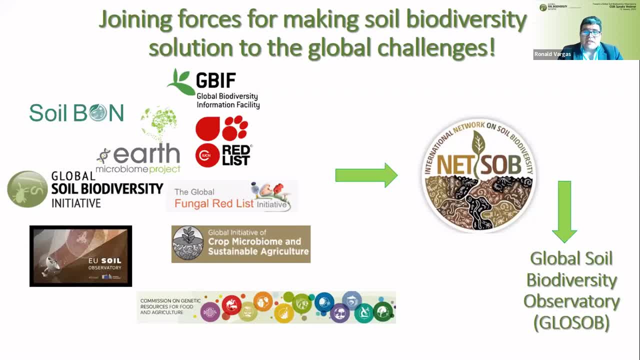 be a solution for the global challenges that I mentioned before, And for this we have established this international network on soil biodiversity, bringing along and together all the ongoing initiatives and experts that are working in this important field. They become the technical forum, the human talent. 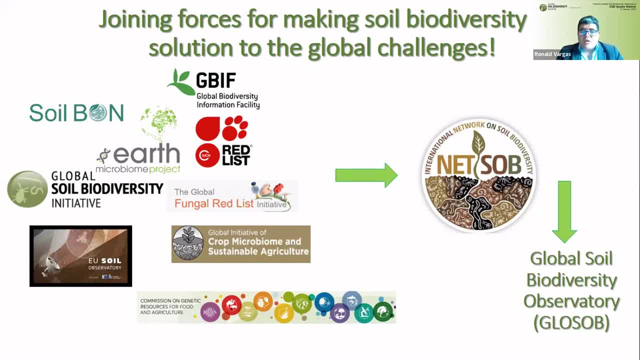 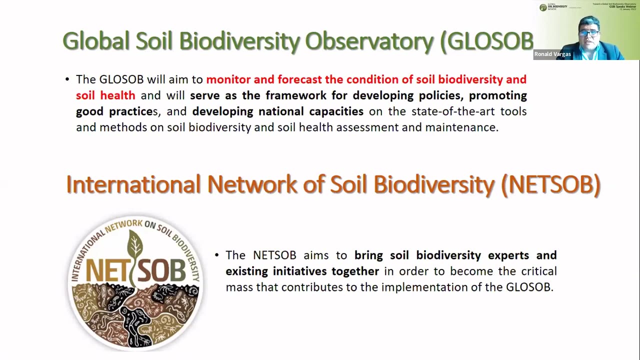 that will make possible the establishment and running of the global soil biodiversity. Otherwise, without you, without all these people and initiative, this will not be possible, Because what we are aiming to do is to monitor and forecast the condition of our soil biodiversity and soil health. 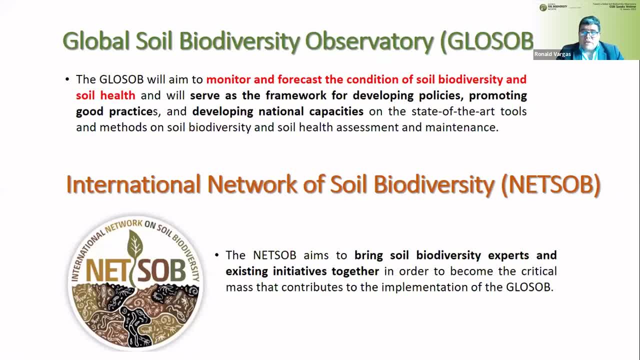 globally, And for doing that, of course, we need to measure. We cannot just rely on proxies or on all data. We need to start measuring. That's an observatory, And for this We need to involve everyone, not only the research community. 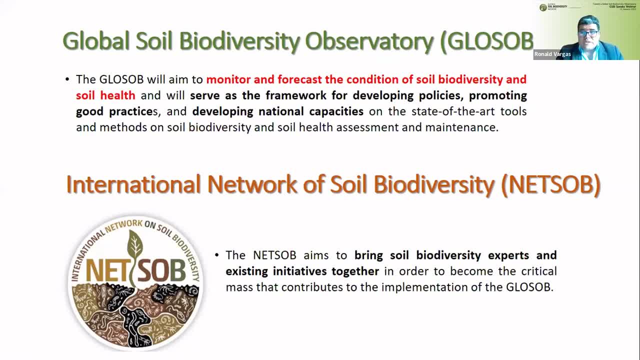 but we need to bring along also countries, because they have to understand that measuring and trying to understand the condition of soils and soil biodiversity is fundamental for the decision making, for developing policies, actions, et cetera. And this is all about. 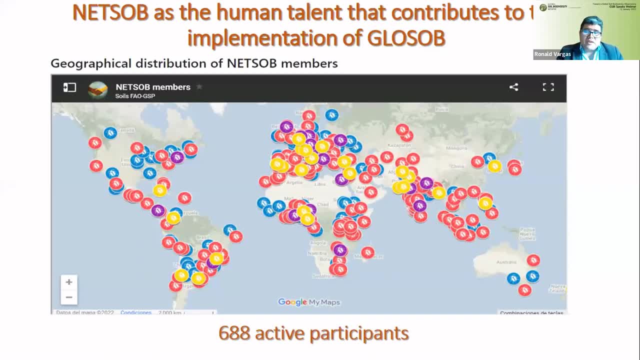 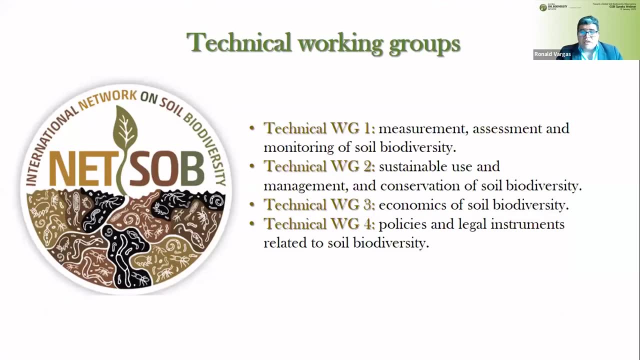 Now the network of soil biodiversity. this is really growing And we have many active participants in terms of institutions and people. We have working groups for different aspects that are fundamental in order to address soil biodiversity, from measuring, monitoring, but also to the time. 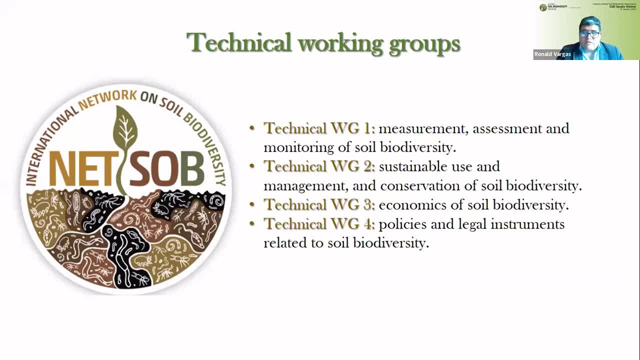 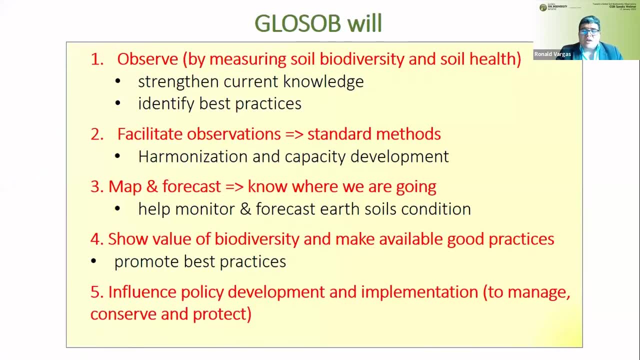 we reach policies in the time, we can use soil biodiversity in terms of good practices to address the challenges. We are currently in the design on how the Global Soil Biodiversity Observatory should look like, what they should be doing, how the governance, the components. 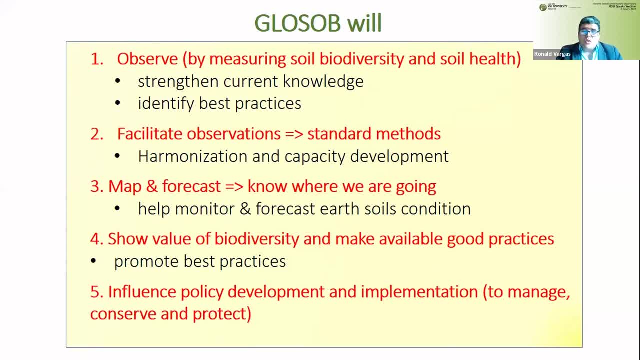 et cetera. And for doing this we of course need you all Because, as I said, we are really facilitating this process And we want to bring all these initiatives and experts to contribute to this very important observatory, Because we will be focusing on the observation. 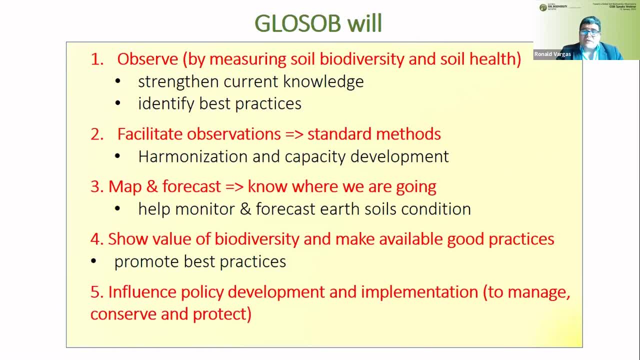 We need to measure, As I said, we need to have common methodology so that everything that we do is harmonized, and we have protocols, et cetera, So that while we the data and information that we will be giving to the decision makers. 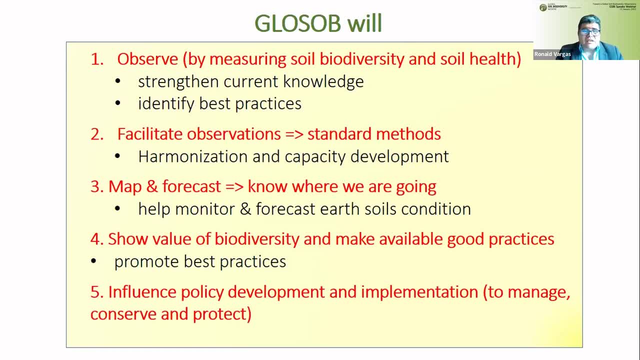 is really harmonized, compatible between regions, countries, et cetera, And that will help us to monitor and forecast the earth's soil condition. We also need to show the value of biodiversity and make available good quality, And we need to have good practices for addressing not only. 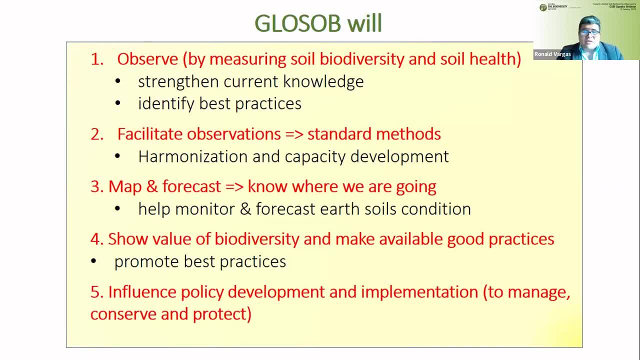 food security, issues related to agriculture, but also bioremediation, et cetera, And we should definitely influence policy development, because that's when we will see results. Otherwise, it will be just we talking to each other without having an impact. 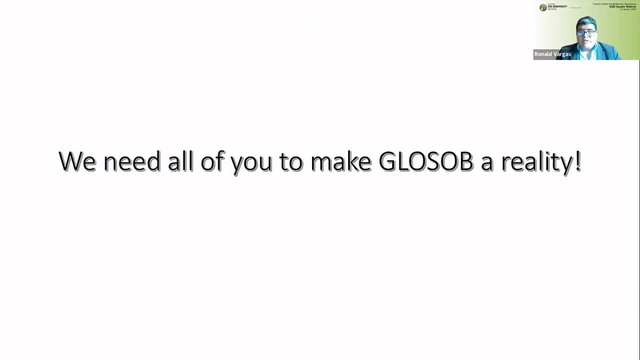 That is why I would like to invite you all to join the International Network of Soil Biodiversity and contribute to the study, And I would also like to invite you all to join us for the next session of the Global Soil Biodiversity Observatory. 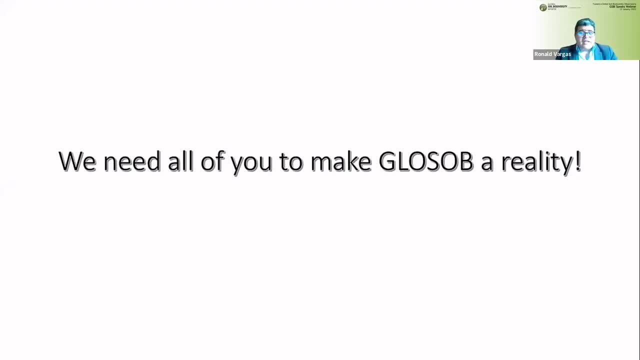 I want to thank the Global Soil Biodiversity Initiative, Diana Wim and all colleagues who made this possible- this webinar- And I really want to invite all of you to join us so that we can make a difference when it comes to soil biodiversity. 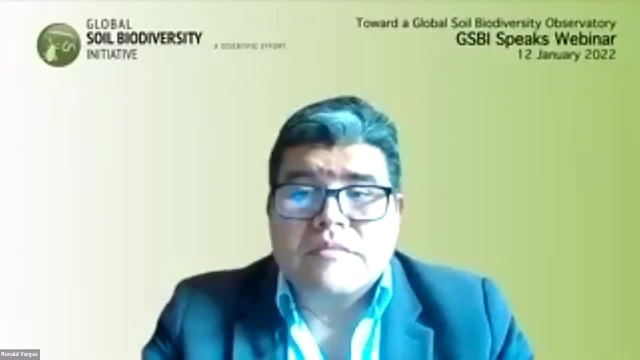 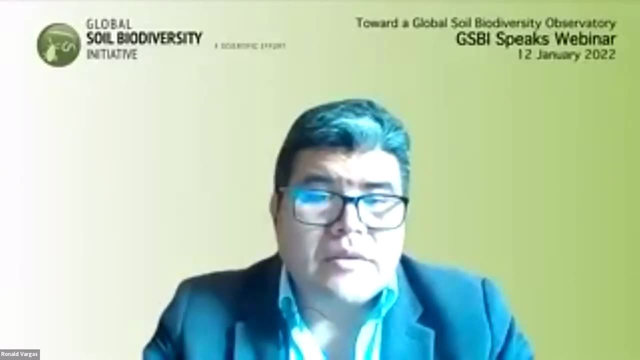 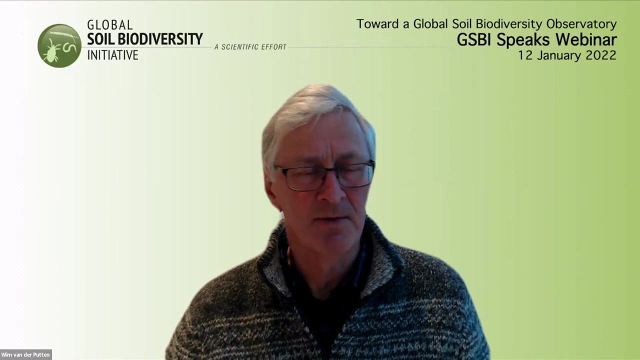 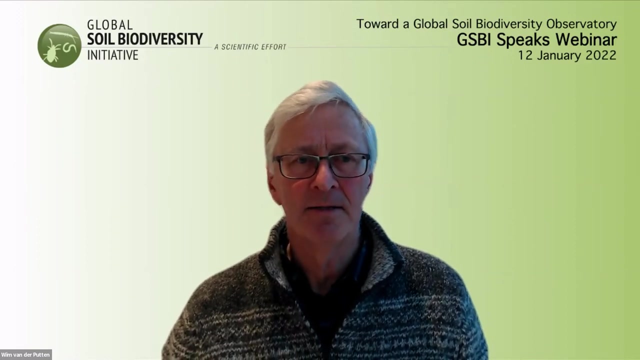 Thank you very much. Thank you very much, Ronald, for this very nice introduction to this ambitious program. We are getting questions ready in the Q&A, so don't hesitate to put your questions in, And the next speaker will be Diana Wall from the Global Soil Biodiversity Initiative. 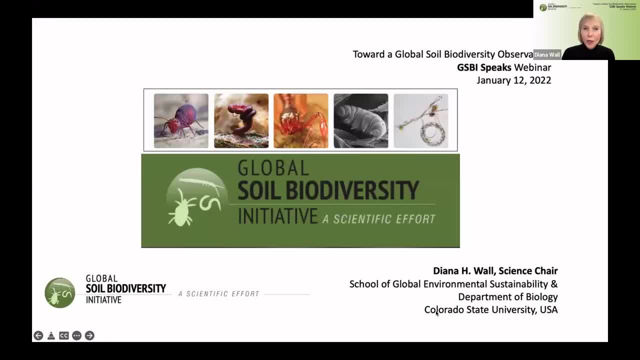 Diana, the floor is yours. Hi everyone, And thanks so much, Ronald- I always enjoy your presentations- and Luca, to help set the stage, I want to explain why we have the GSBI and how. I hope that we can contribute A little bit of knowledge right now. 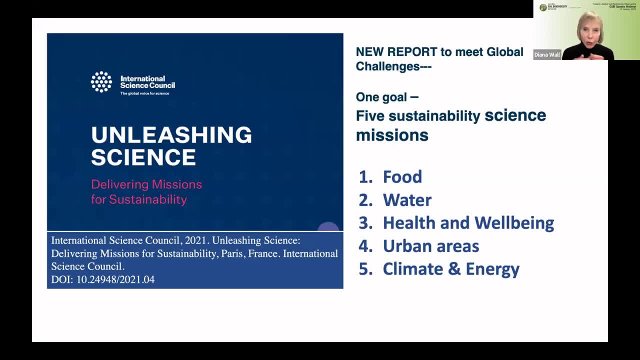 is that we are facing so many challenges, And I saw this report that just came out by the International Science Council And they were looking at the same thing. we're looking. How do we get the information to address what is happening in food, water, our human health? 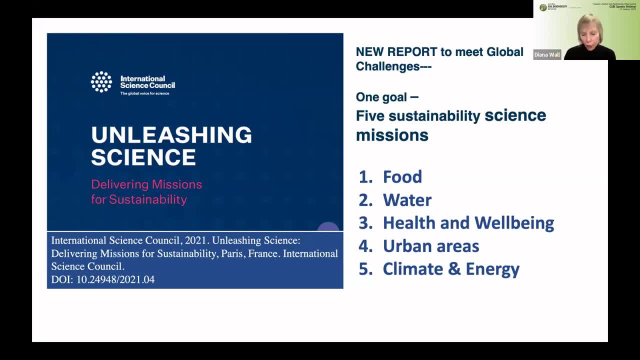 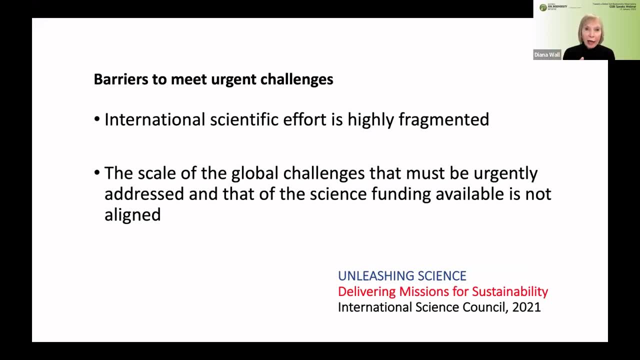 urban areas and natural areas, and climate and energy, And they have come up with those five targets and said that there are barriers now that are existing that are stopping science from really coming together to address these issues. And I think soil's been in there, in soil biodiversity. 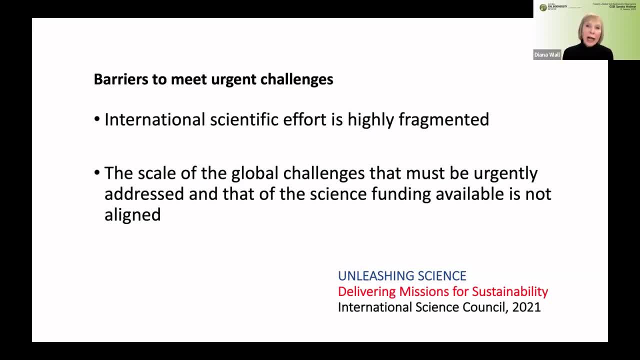 Soils are also, And soil biodiversity in particular is highly fragmented. We have scientists who study a single organism for their whole career and an interaction with what it feeds on in soil, And there are many different types of predator-prey interactions, trophic interactions, many species. 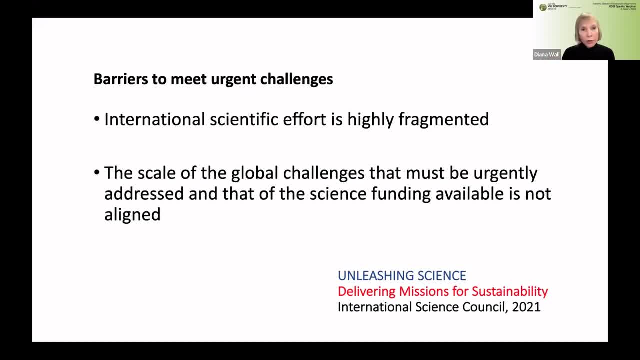 But we also have biogeochemists who look at nutrients to connect the whole ecosystem above and below ground And it's getting those people who are already interested in soil biodiversity and how it connects above ground, below ground and what it does. that is really going to be important to meet. 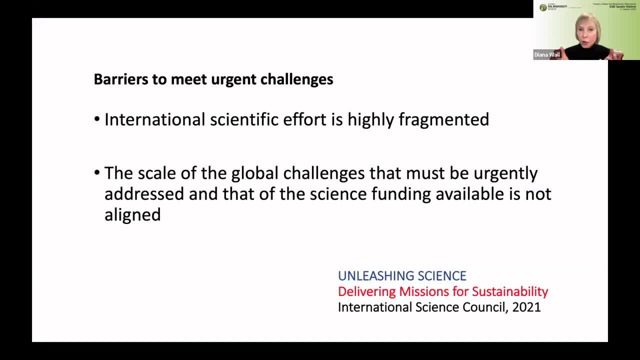 these urgent challenges, So all of our science is from many disciplines and we're really lucky to have it. But the second thing is they pointed out- and this is a number of challenges that they listed- that the scale of global change issues the challenges. 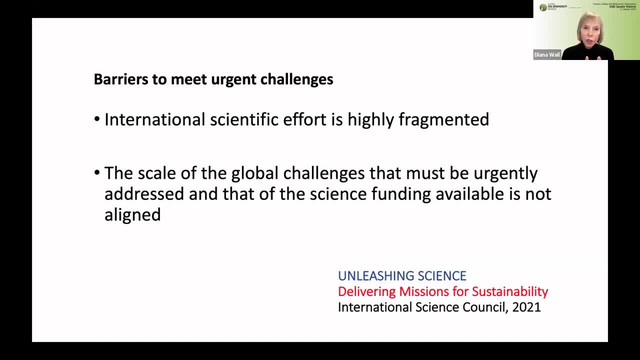 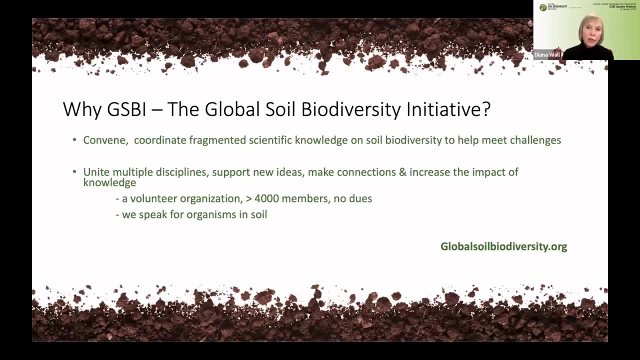 particularly biodiversity and climate change, has to have more scientific funding and infrastructure, And I think we've seen some of the ways this happens from Luca and Ronald's discussions. So why the GSBI? As mentioned, it started in 2011.. A bunch of scientists got together. 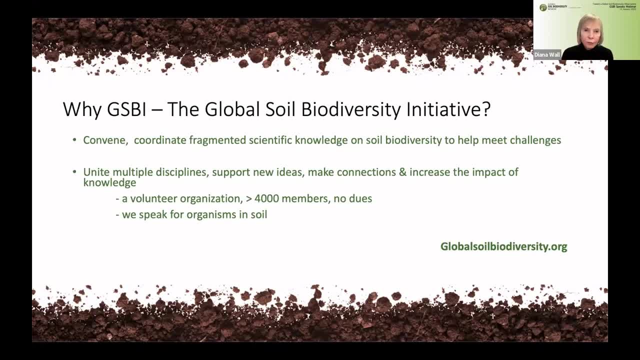 We said we need to pull this information. we know a lot already in 2011.. To help as we're moving forward to address these challenges, And so the GSBI is just kind of a cornerstone, that kind of talks with people. 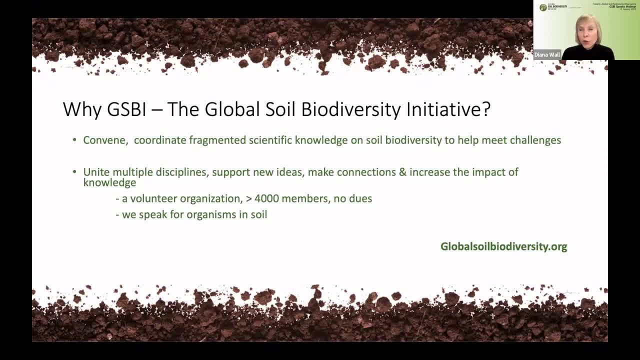 unites different disciplines, supports new ideas, tries to make connections, And we're volunteer scientists. We've got, we think, more than 4,000 members, But with volunteers we don't have a way to count them so far. 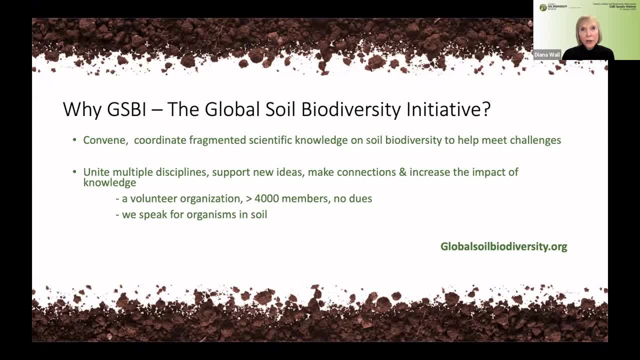 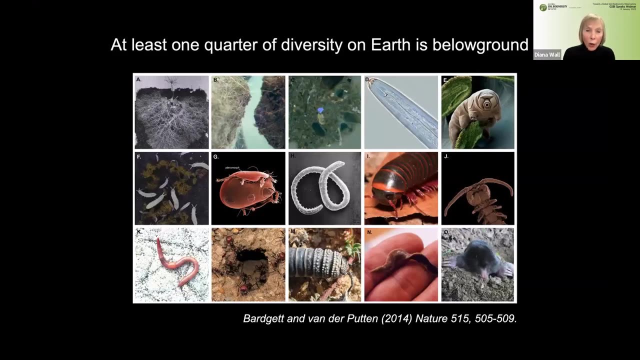 There's no news dues, But we do feel that we need to speak for this interconnecting, complex interaction of all these species below ground. What are we talking about? Many of you have seen this picture We've got, at least the estimates aren't great. 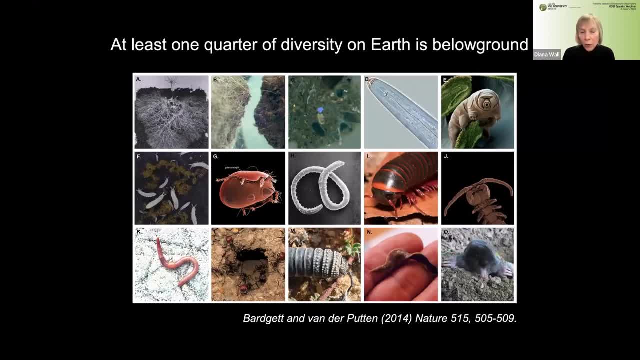 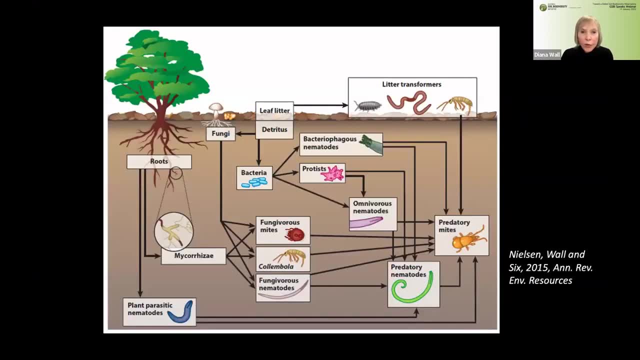 but at least a quarter of diversity is estimated to be below ground, in soils, And, as you can see, it's animals, plants, and behind each one of these boxes, they're doing something in an ecosystem, Whether it's the fungi, the bacteria. 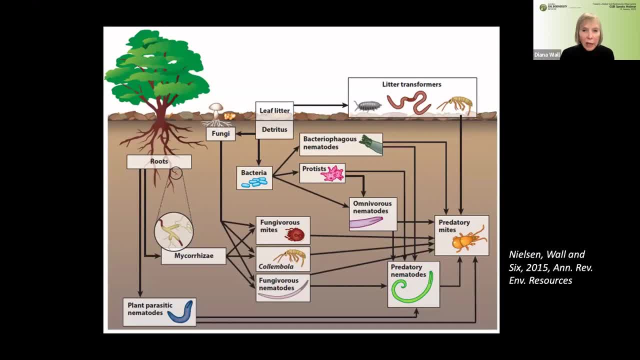 the mycorrhizal networks, the columbula, the mites, and going on up to huge earthworms- and huge to me because I study nematodes- but going up to huge animals. How are they all connected? 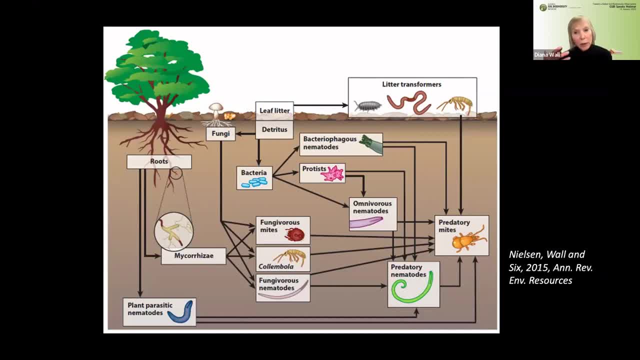 Where are the taxonomists, the species, people? How do we resolve molecular and taxonomic and functional what they do in soils? So these are big issues and there's data on this and we think it can be helpful. So the GSBI. 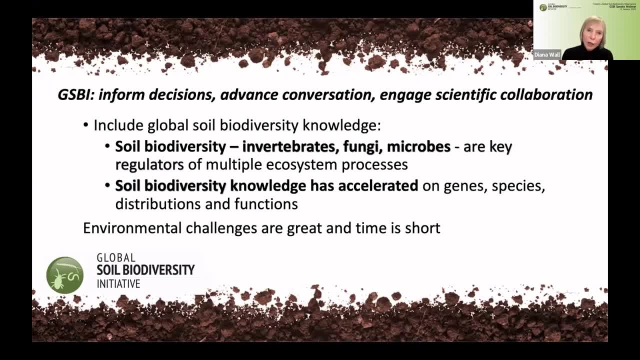 it's trying to be a link between what we know, the knowledge on soil biodiversity as key regulators of ecosystem processes that give us these ecosystem services we're dependent on, And it's just a point here to say that soil biodiversity knowledge has really accelerated. 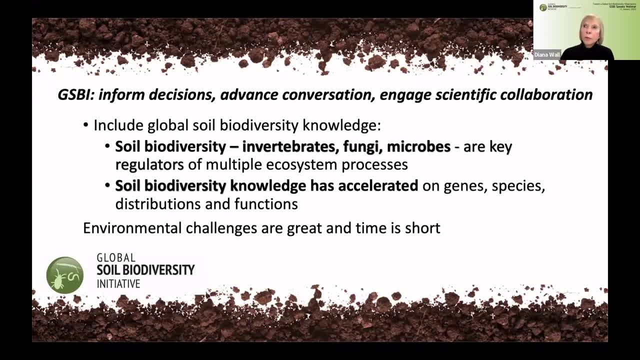 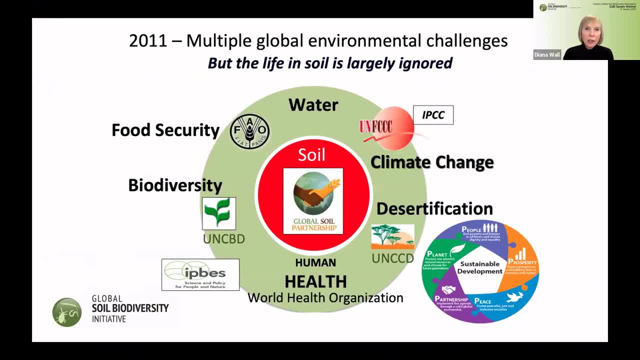 It's just tremendous that both the technologies, the numbers of people, the interest- and it's good because, as I keep mentioning, we've got an urgency Here- have there been many slides so far to show you these challenges And I just want to reiterate that when we started in 2011,. 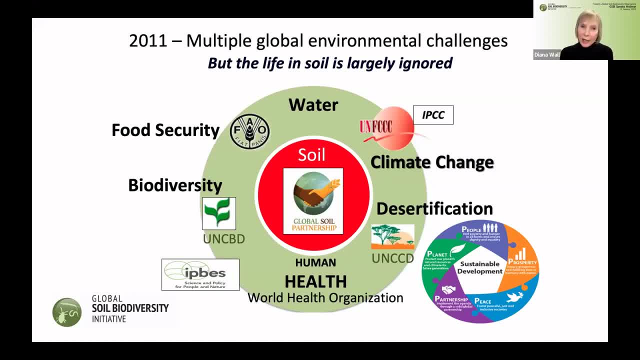 and this is not long ago. And again, we had a kind of a basis from the 2002 group of scientists that were going to be listed in the convention on biological diversity, you know, the international initiative on soil biodiversity- but we really kind of wanted to move faster and really 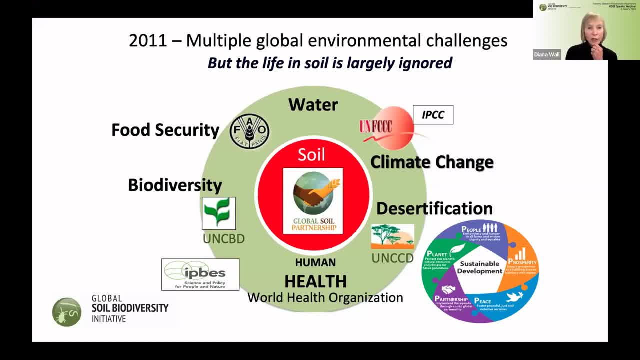 really address these urgent challenges. And now it's nice to see that we're all convening. but here you see, these big issues We could take water, food, biodiversity, human health- All of these have now become missions from, as I showed from this new report from the international science council saying: 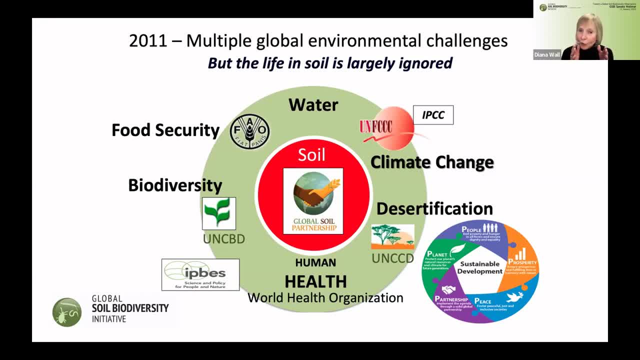 that research must be looked at like a mission to make our planet better, and soil and soil biodiversity is part. right in the center where we see the impact of soil biodiversity, We see the global soil partnership. It's really integral to getting all of these issues addressed. 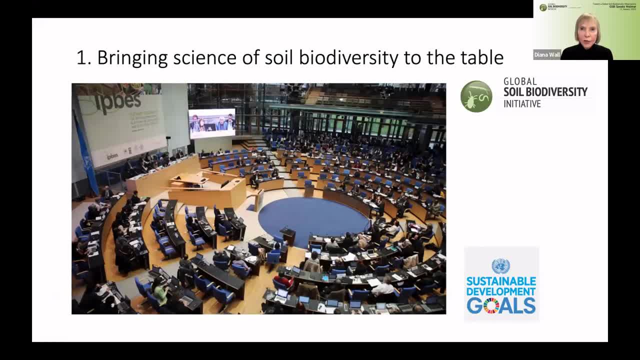 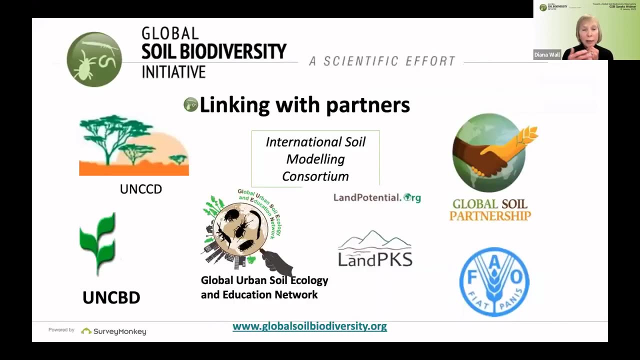 So, young scientist, here's your chance. What we wanted to do, basically, is just bring science of soil biodiversity the table, whether it is biogeochemistry, whether it is above ground looking at below ground- all the interactions we wanted to bring to the table. 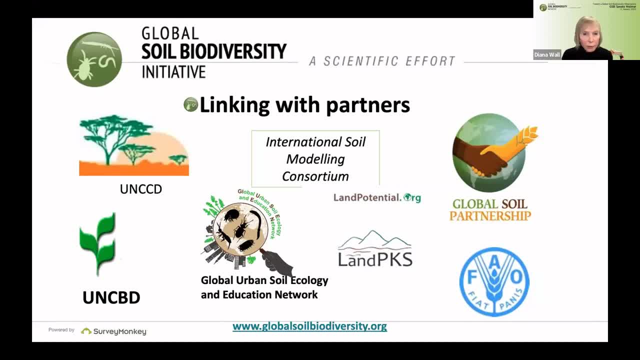 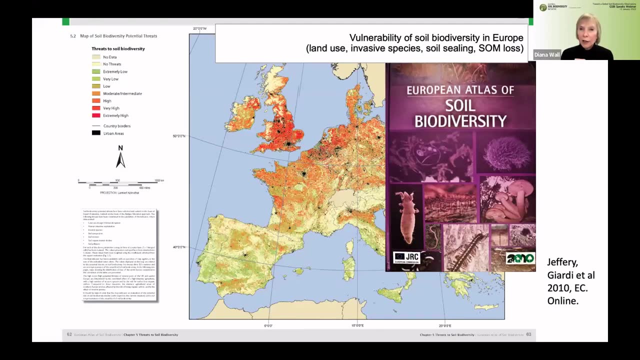 We do this by linking with partners. It's already been mentioned How many partners are now available and interested in soil biodiversity and we can do more together. It was mentioned by Luca about this early Atlas, which was just fascinating to me. It wasn't a GSBI project per se. 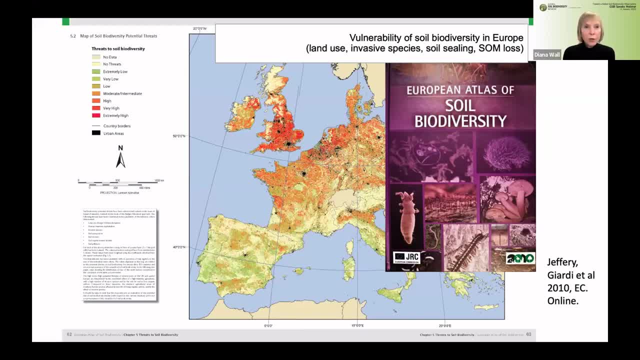 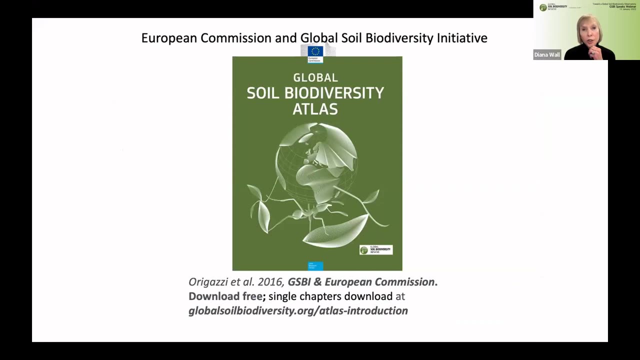 There were people involved in it, obviously, that knew different organisms, but this is a map of threats to soil biodiversity And that is based on knowledge at that time And it's pretty, pretty effective And from that we had partnerships. The GSB idea has already been mentioned. 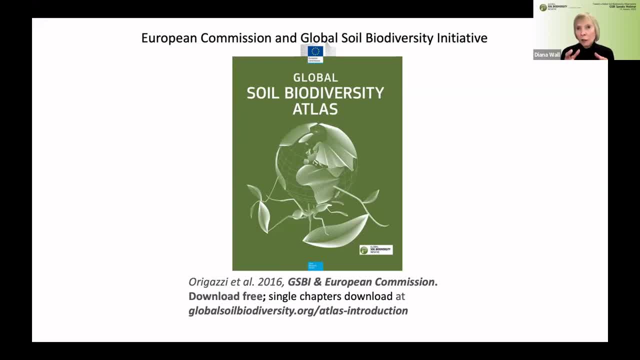 um with this document, which has become both available for teachers. It is being used. It was being looked at by policy makers. It is now being brought up as a reference for talking about what each group of animals. it's got gorgeous pictures of what each group from microbes own up. 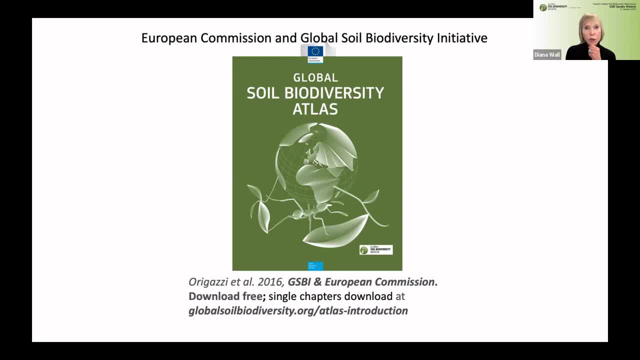 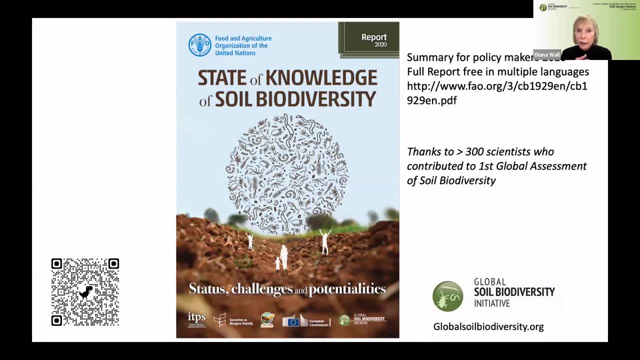 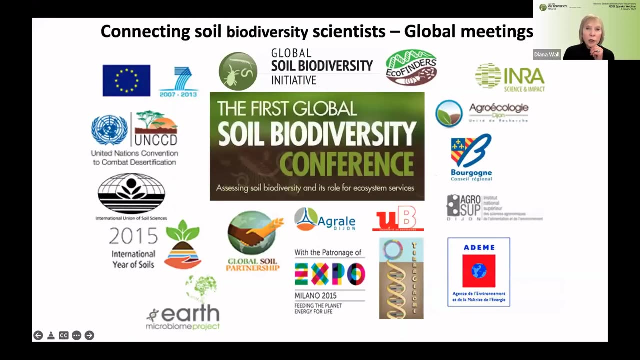 does and what their functions are. what are the ecosystem services? But this scientific assessment that was recently done, in 2020, is probably one of the most important things I'm gonna try to get. I can't get that off. The next was that we also connect soil biodiversities. 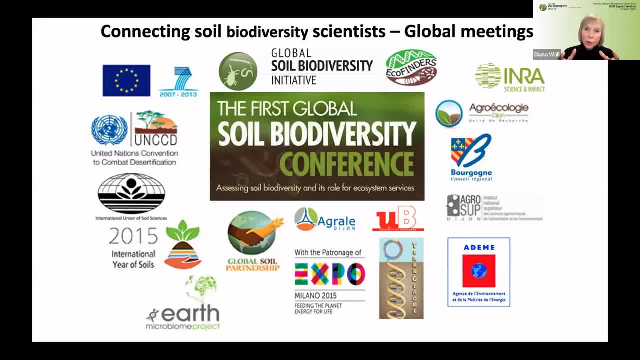 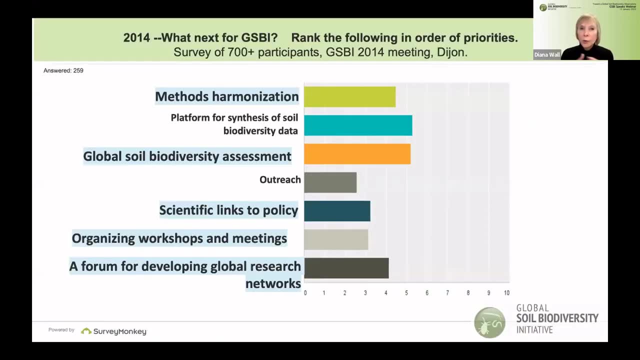 in global meetings. This is just an example of the number of partners that were involved in our first meeting that was held in Dijon, France, in about 2015,, I think, And one of the questions we asked the participants, and you can see there were about 700 participants. 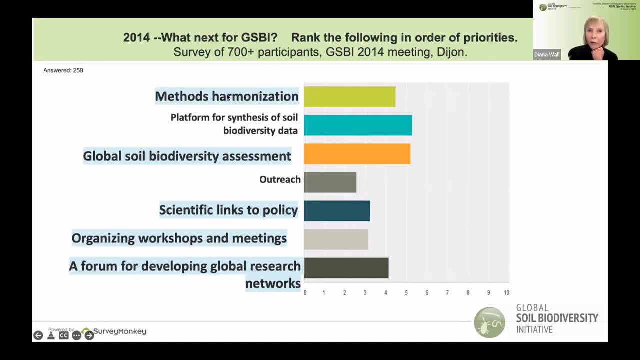 was: what do we need to be doing? And right now? the things that we've just heard that have taken years to get into policy and now we need to do it are methods, harmonization, an assessment, such as the status on soil biodiversity. 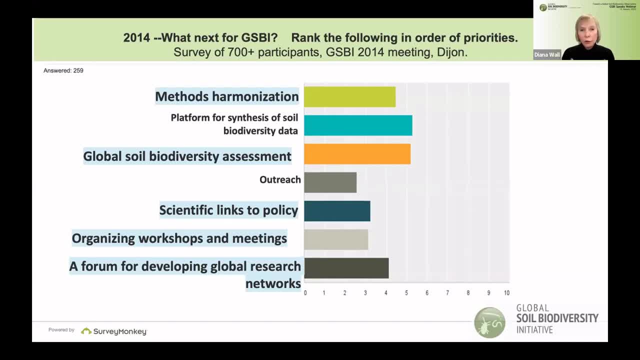 the scientific links to policy, providing that knowledge so they can move forward, credible knowledge, convening with each other so that we can cross these disciplines, and just serving as a forum for new global networks, And there are many of them that are coming up and already running. 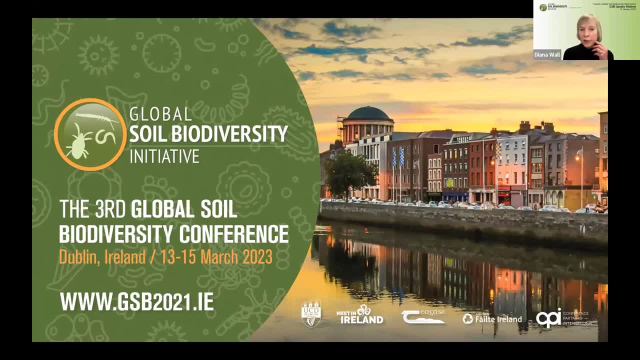 The next meeting we will convene will be in Dublin. It's in March of 2023.. It's in March of 2023.. We're looking forward to seeing many stakeholders there because, as Ronald mentioned, we have to be together on this. 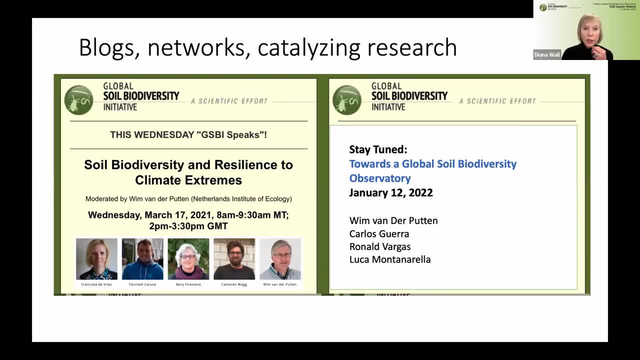 We also connect through this monthly blog And I just want to give you another example of the type of topics that we do talk and we're interested in hearing more topics from you all and people who are interested in talking. I wanted to show that some of the advances here. 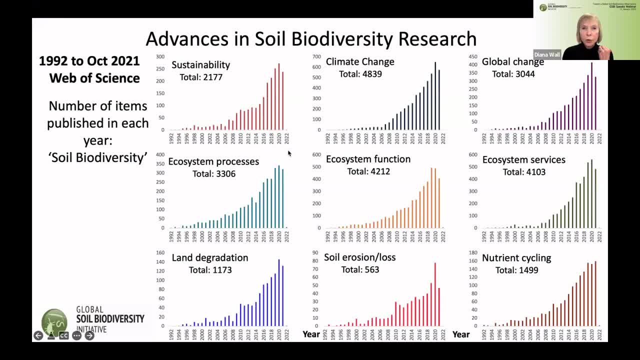 these are graphs from 1992 to 2012.. These are graphs from 1992 to 2012.. These are graphs from 1992 to 2012.. These are graphs from 1990 to October 2021.. And on almost every single item that we have here. 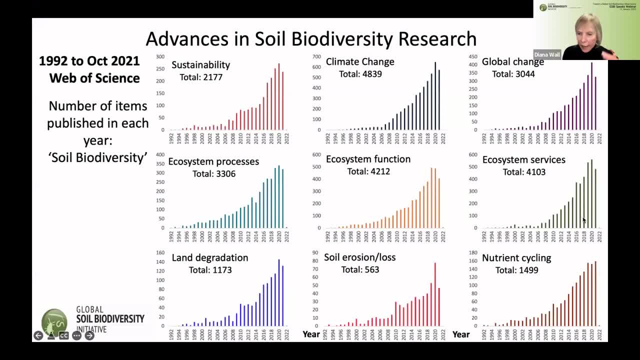 you see the numbers of papers going up. The numbers of items published went up. So we have had an impact here with a broader awareness among the scientific community that there is life in the soil. We need to consider all the soil and its above ground interactions. 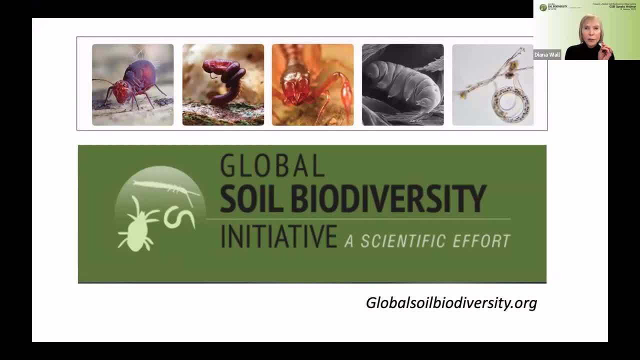 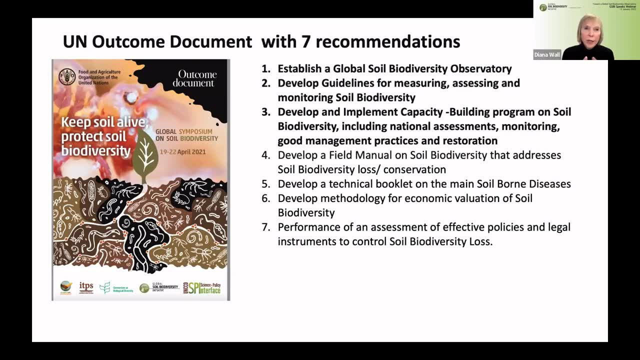 So what's next next? I love this picture of all the organisms. That's from the Atlas, so you all should get one. What's next? Well, this outcome document has been mentioned and it lists seven things that need to be done, And we're concentrating on number one, but many of these are being done, as mentioned. 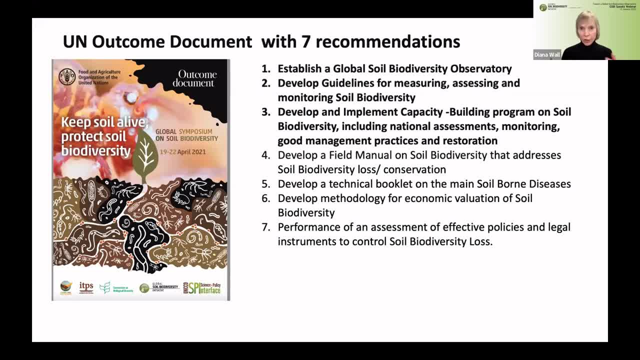 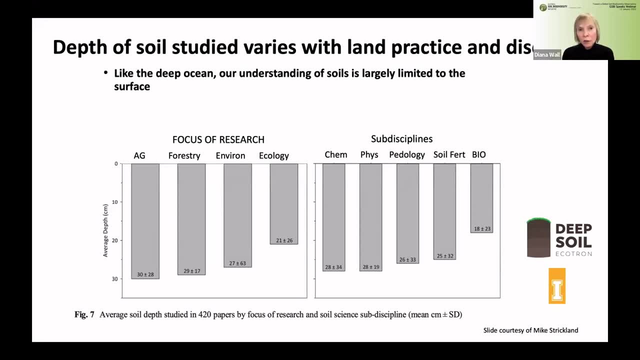 by the International Network, the Netsub, and all of us are involved. And for today, you know we're going to be talking about this Global Soil Biodiversity Observatory, but I want to not limit this discussion in any way. For example, this shows in a number of studies: 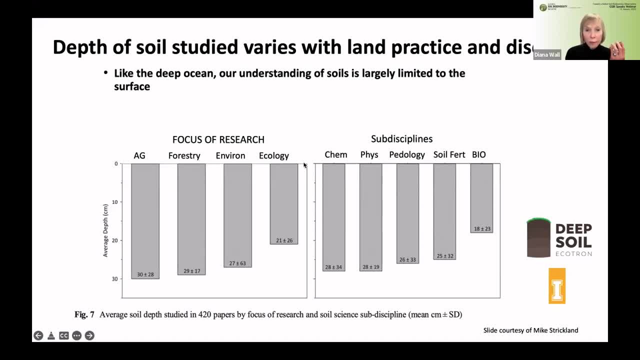 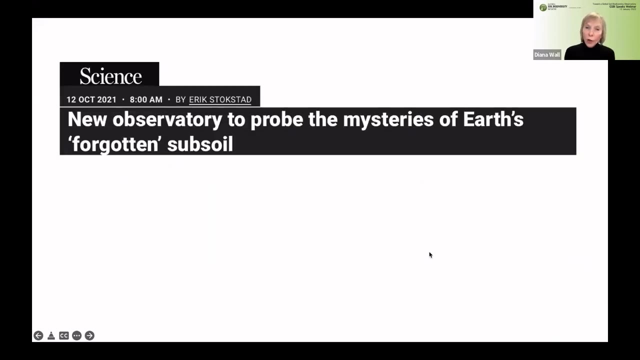 the focus of research for agriculture, forestry, environmental research and ecology and the depth of soil. that has been studied mostly at 30 centimeters only, And for sub-disciplines- and this is from 420 papers- you can see that it's 30 centimeters or less, And so a new type of observatory is going to have to. 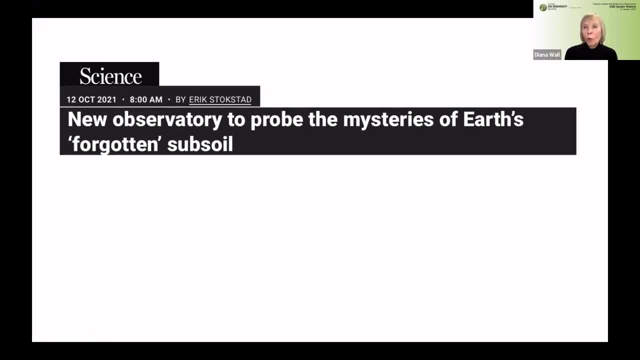 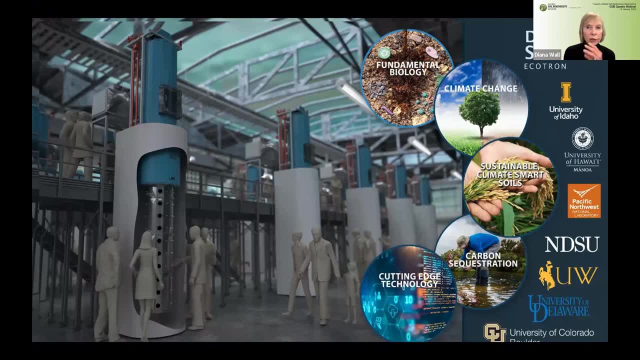 be thought about to probe what's below that- 30 centimeters, And here's an example of one that's going to be at the University of Idaho. It's got lots of partners, but it's three meters deep And they're going to take proposals to look at everything from global change scenarios and 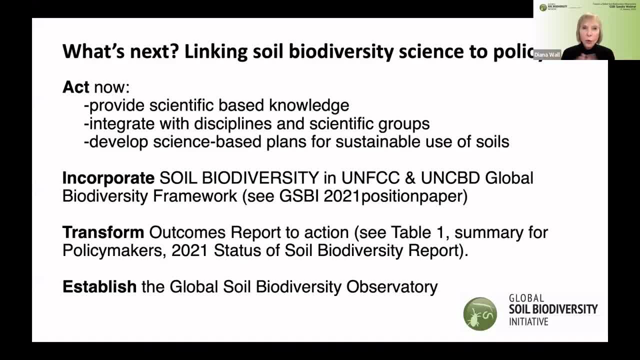 the plants above ground. It's quite fascinating. So we don't want to limit what's going on. We need to link our soil biodiversity science to policy. There's many ways we need to act: by providing science knowledge, or integrating with other disciplines and scientific societies, or 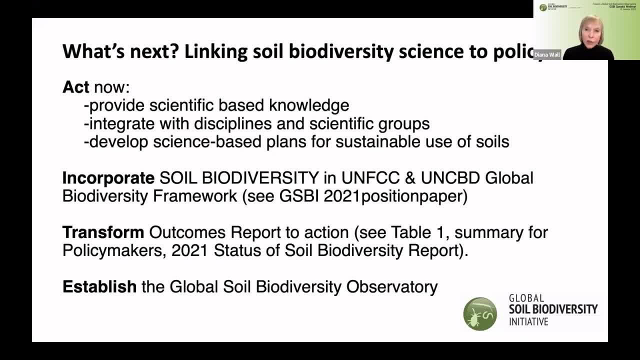 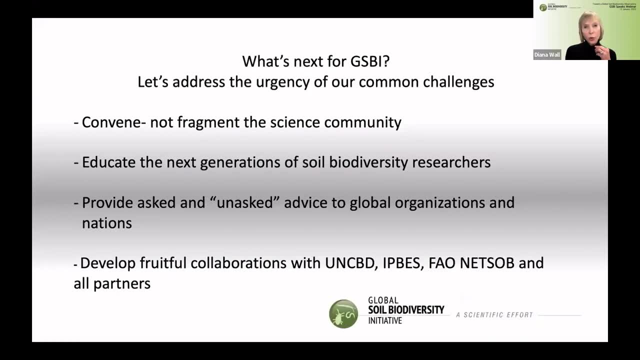 whatever Incorporating it has been mentioned in the policy- the new framework for 2020.. We have a position paper. we wrote to the CBD for that. We need to work on those outcomes that I just mentioned and establish this observatory. But we want to not forget that 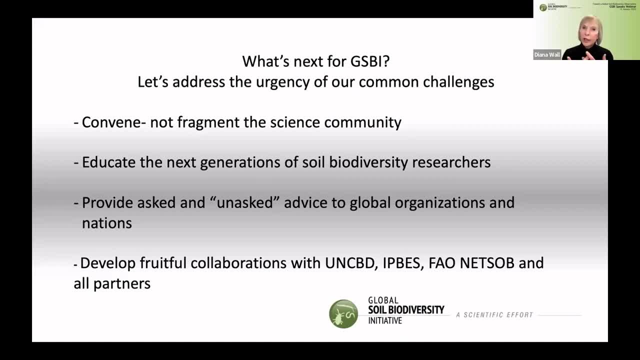 there's an urgency and a reason for scientists to now come together, whether it's through mission based science or just for soil, biodiversity science, to inform other science and then the decisions that are going to be made on our lands. We need to not only think of ourselves, but think. 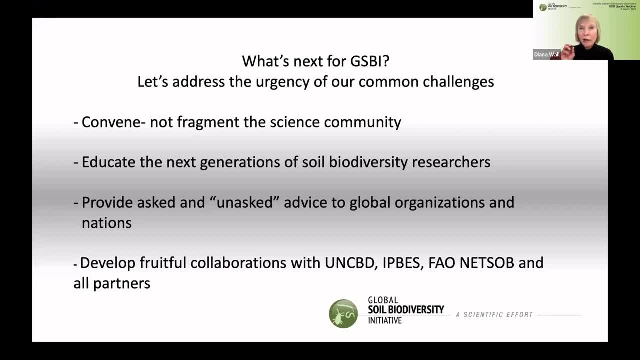 about the next generation of soil biodiversity researchers and how excited they are to be able to be part of this, And I think that's exciting. The technology is now from using artificial intelligence to look at through microscopes to provide the public with a better understanding of. 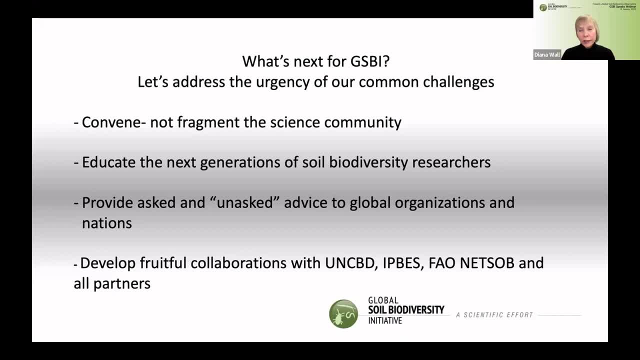 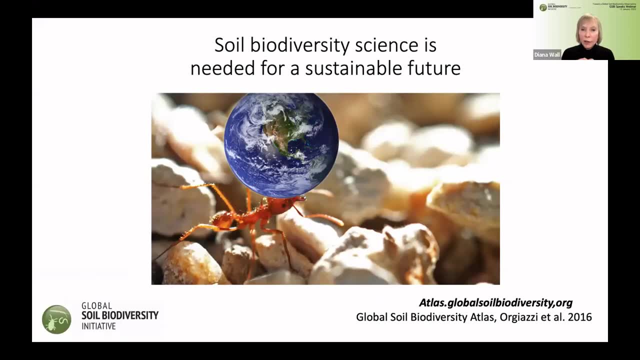 what we're seeing and why we're excited about the science. We're going to continue to partner. I think this is all very important and it keeps GSBI busy. So with that, I'd just like to say that this picture from the Atlas is just one example of how the world is changing, And I think it's a 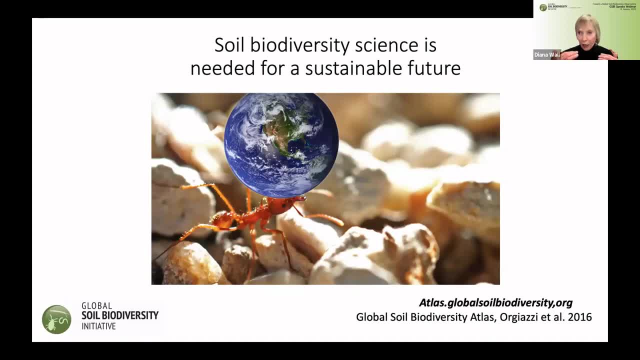 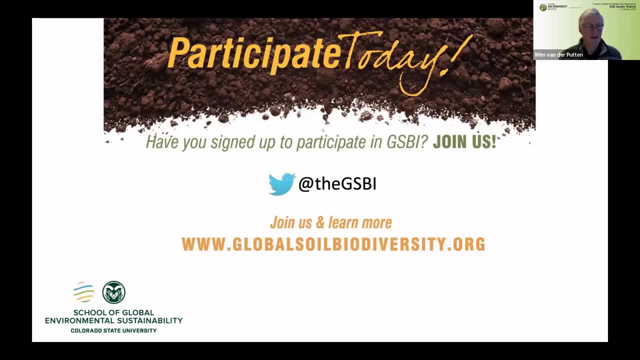 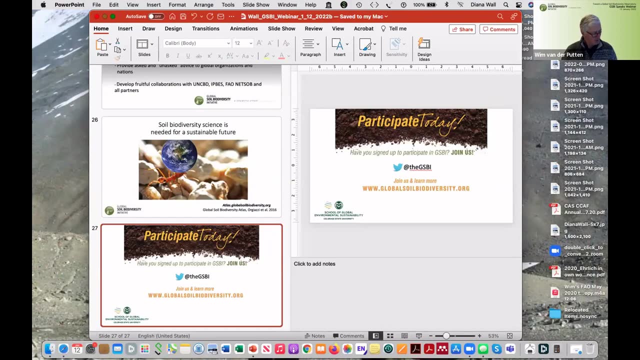 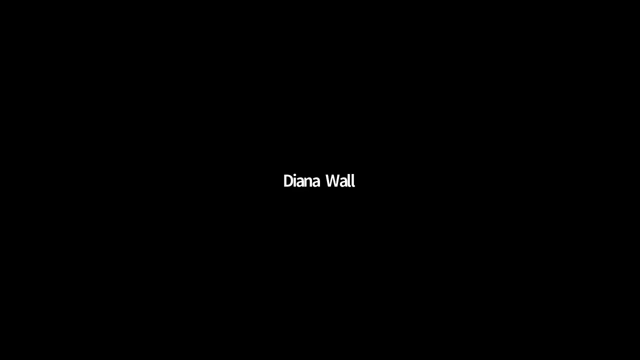 good example of how the world's problems are really sitting at our level. Thank you. Thank you, Diana, for this introduction from the GSBI perspective. It's amazing that we have over 4,000 members already. So the last presentation will be by Carlos Guerra, and he will bring us to. 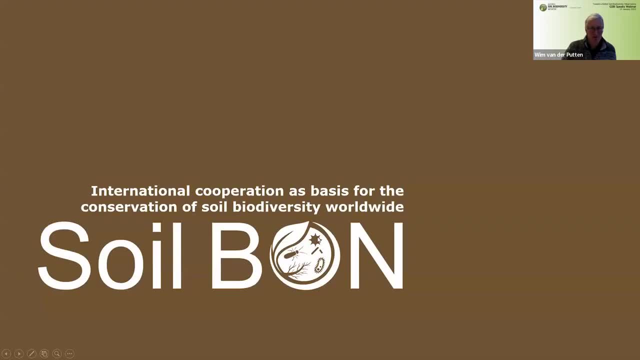 how to analyze soil biodiversity And he's going to talk a little bit more about soil biodiversity. So the last presentation will be by Carlos Guerra and he will bring us to how to analyze soil biodiversity And he's going to talk a little bit more about soil biodiversity. And also he will bring us to Africa. 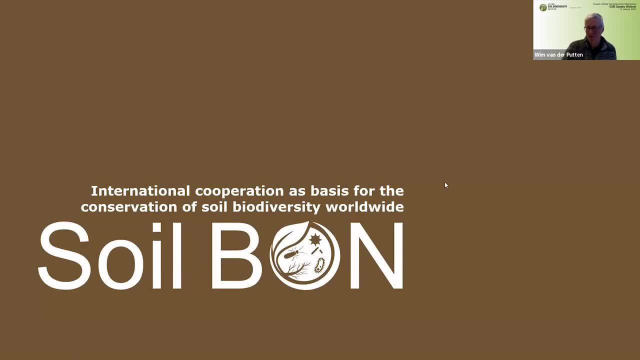 or at least to outside the Northern Hemisphere. Carlos, the floor is yours. Thank you very much, Wim, And thank you all for attending the panel. So it's not that I'm going to take you to outside the Northern Hemisphere, but I will try to focus a lot on some of the 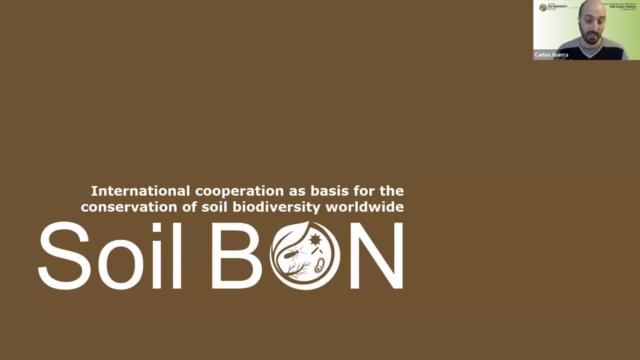 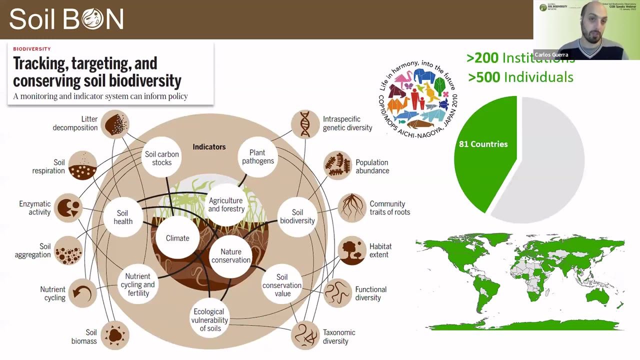 issues that we have been facing when trying to implement an actually global soil monitoring system that tries to be as balanced as possible across the world. First of all, I would like you to know where we come from. So the idea for us of implementing such a system, 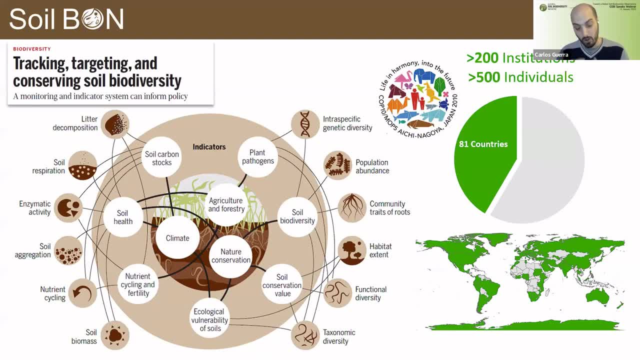 implies that we look at soils not only from one perspective, but we try to understand soils in a multitude of perspectives. This involves including all the diversity inside soils, also the chemistry and physics inside soils, but also the function within soils, But at the same time to build a 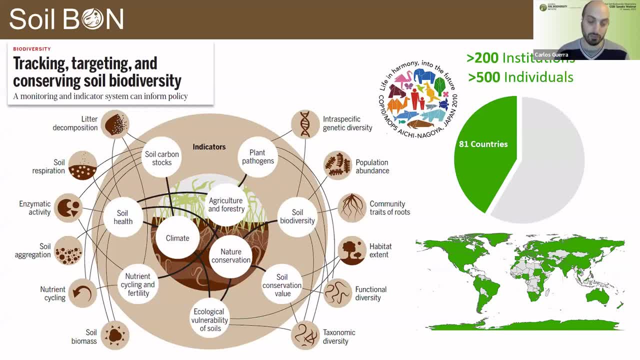 project like this. we need to, or we aim to, create a project that is actually open: open for the participation of people, of researchers, but also opening the way that we want to communicate our science. The idea behind SoilBoil is that you own your data, you own your soil sample, you are 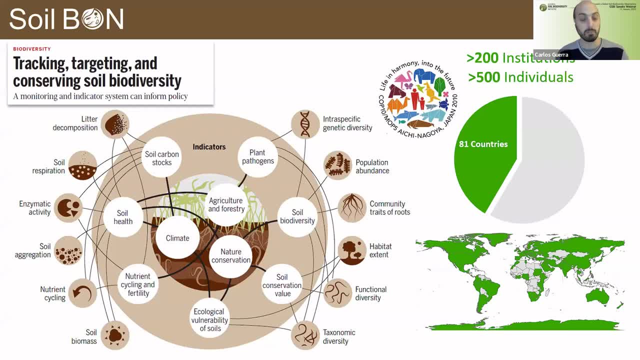 allowing us to use it in a more broader spectrum, but you're also allowing us to use it in a more more broader spectrum, but you're also allowing us to use it in a more broader spectrum, but you're are also allowed to use it yourself. So let's say that you want to develop something in South. 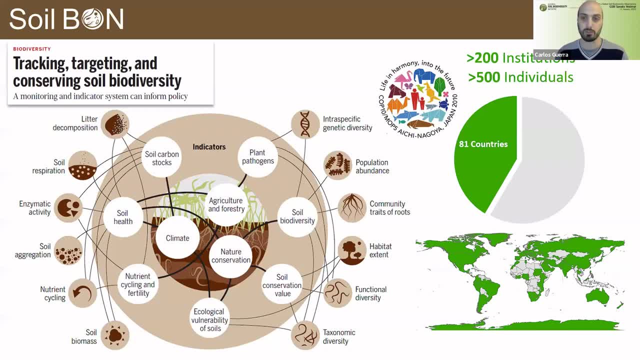 America, for example. all the samples of soil one will be available to you. What this also means, in order for this to be possible, is that we want full standardization. What this means in practice is that what we want people to contribute is actually soil, so soil samples that will be. 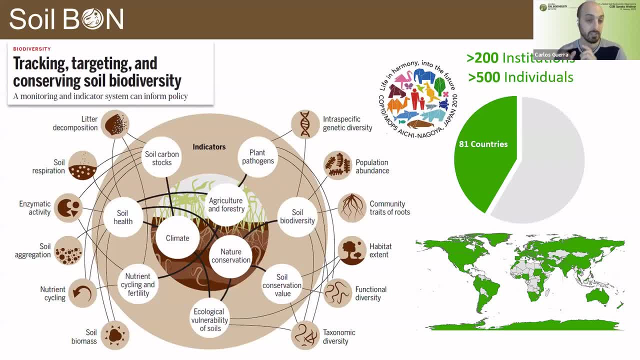 standardized and all pull together in one single macro frequencies that will touch all these aspects. In this scope. what we are now able to do already in during this year, or we will be able to do this year, is that we will be able to sample in about 81 countries that will send the samples of. 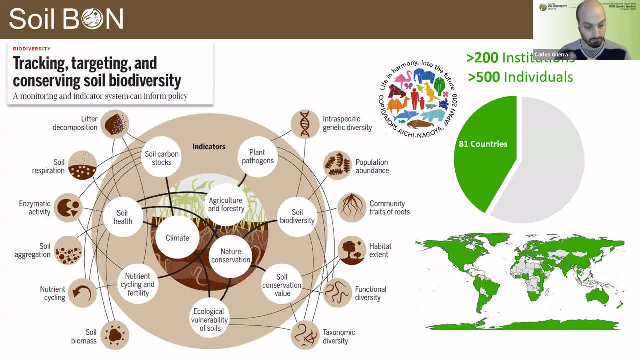 soil, and then we will try to do all this analysis in a standardized way. This implies one thing that is very critical, because when doing this type of sampling, where this level of standardization enters into play, we have to comply with international law, And while for many of us, as researchers, this compliance with law 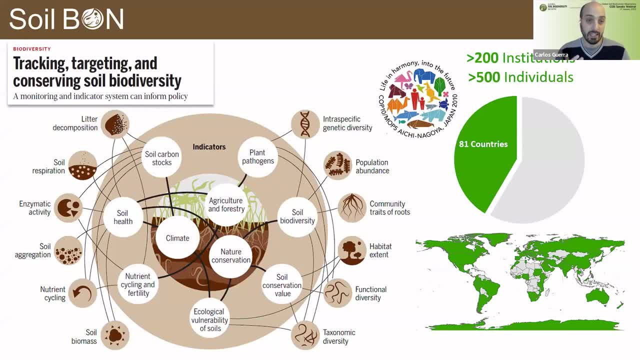 is something that we never touch or never think about. it actually matters, And there are some countries where this matters a lot. You can go to jail, you can have your career damaged if you don't follow the law. So because of that, we want to protect everyone involved here And 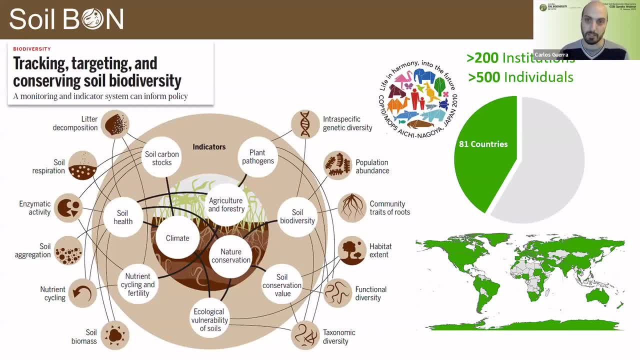 this is a critical aspect for us: to be Nagoya compliant and be compliant with international and local laws. At the same time, this is also a mechanism that stops much of our research, because we focus on nature conservation, nature protection and try to have more sustainable soils. But this type of legal instruments, although probably 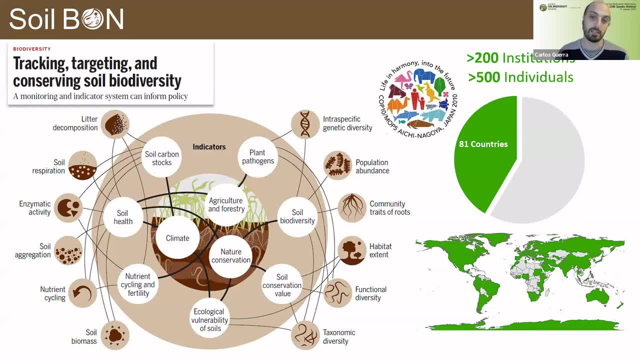 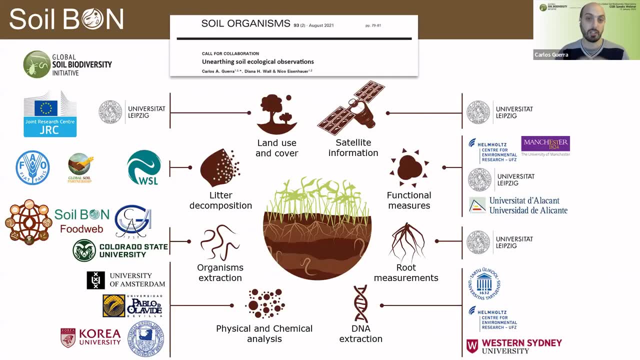 necessary, they in many cases stop our capacity to do more broad research. As I was saying before, we are trying to look at soils from a very complementary point of view, But this implies that this is not a work for one institution only, Contrary to, for example, the first example, that 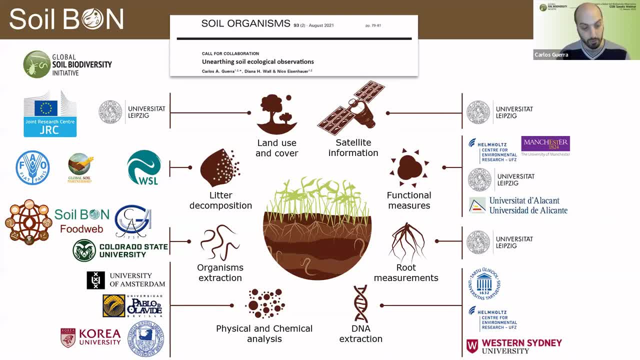 Luca presented, where the GRC is the main force behind the Lucas Program in Europe and the European Soil Observatory, although it has partnerships with our institutions too. In SoilBON we are built based on partnerships because otherwise this would not be a possibility for us. 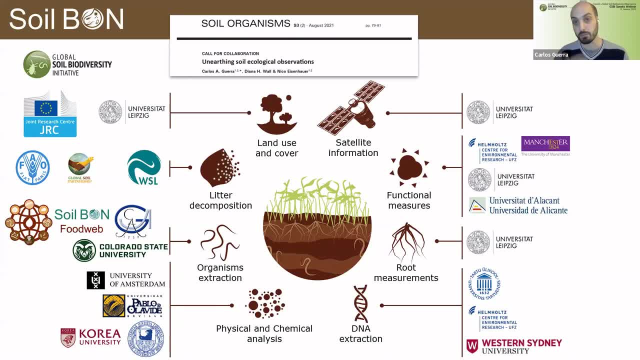 And this implies having partnerships or different partnerships for addressing functional properties of soils, to addressing physical and chemical properties of soils, to addressing the diversity of soils And just touching on one of the questions that I saw in the chat already about taxonomy and the use of taxonomy, these types of things. So, as you can see, here we are also. 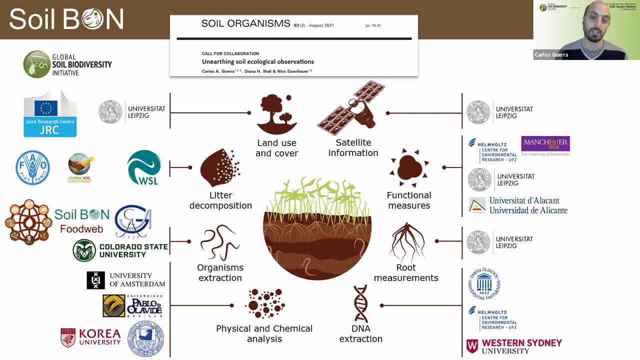 aiming to, for example, do organism extraction within soil samples. And this assumes that we have a network of taxonomists, a local network of taxonomists, Because if it is already hard to ship samples from- I don't know- Berkeley, for example, to other countries, then we have to 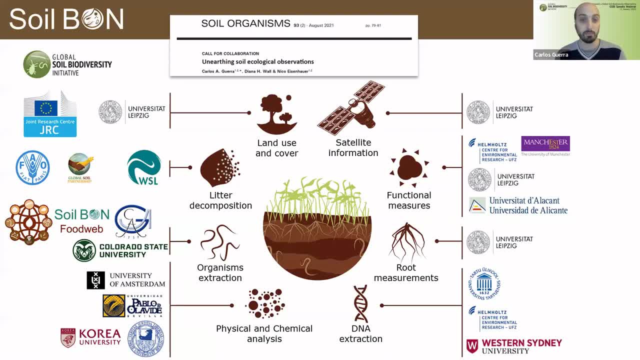 do this on a proper basis. In other words, if we are shipping samples from, let's say, you know, Brazil, or from Angola to Europe and to do this standardization in terms of analysis, imagine what it would be if we were starting to sample or to ship actual animals And for that. so, considering that, 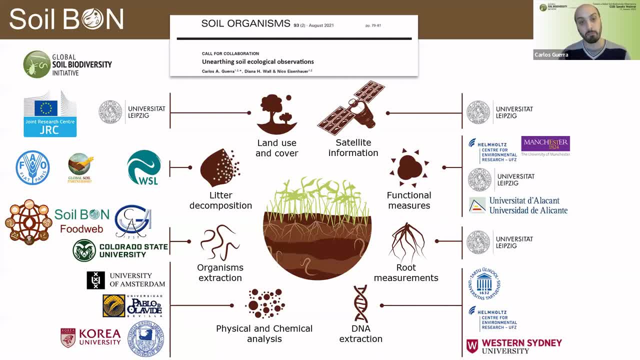 impossibility. we are in the process of building a network of taxonomists, So to have them also participate in this type of global network and global sampling scheme. At the same time, it is very important for us to understand that we are creating this and we are 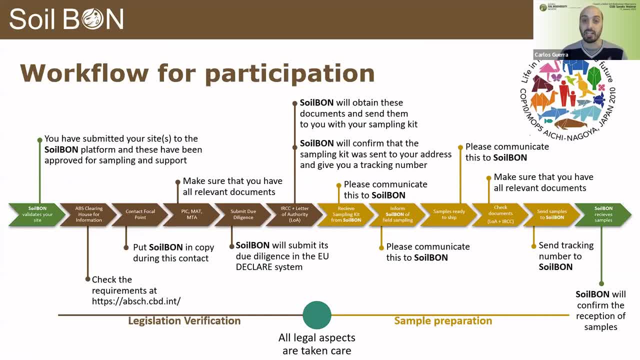 time. as I was saying before, we have to have a very clear way of communicating how you interact with this type of network, Interacting with this type of network. it's not. this is not about citizen science. Although we work as always, volunteers, we are not looking for the average. 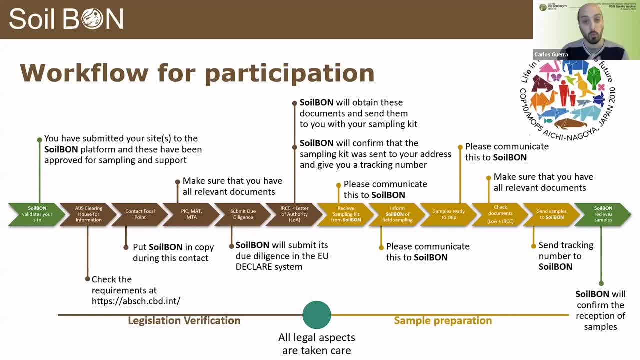 person to directly contribute to this, just because we have to overcome severe in some cases, in some cases very easy legal issues in order to be able to actually sample in all these countries at the same time. So we have a very- we laid out a very structured way of how to overcome all these. 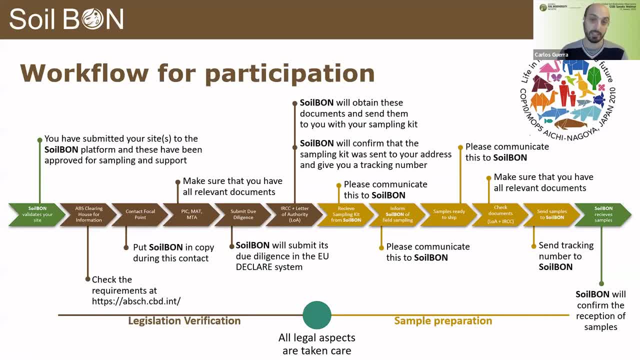 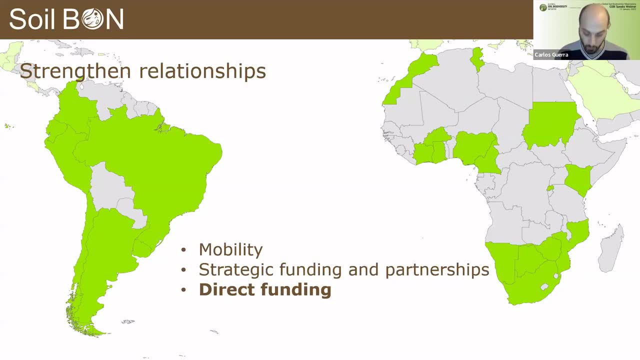 issues And we are, for example, in that way informing directly the efforts of FAO in trying to keep up with the current laws and the different nationalities, The national mechanisms that exist- Talking about what Wim was saying about bringing these questions to the southern hemisphere- 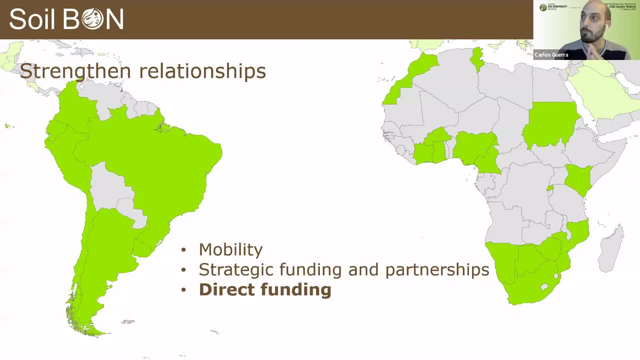 I would like to come to this, not, I would like to come to this because I feel that we are. when we are developing these networks, these global networks, we keep missing the point, And myself included. So when we started all of this, there are several issues. 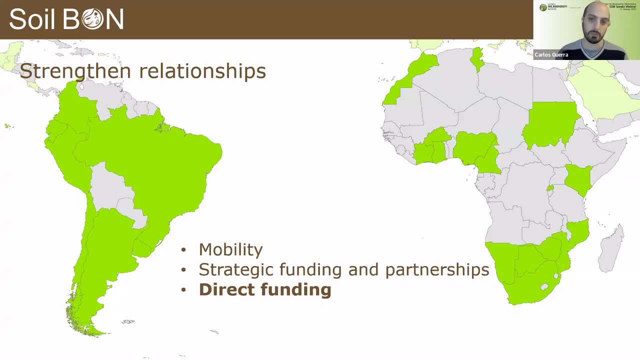 that we did not consider when structuring this network. What you see here in this slide on your left is so: in green you see all the countries that participate already in soil bond And you can see that in South America you have most of South America represented in the case of Africa. 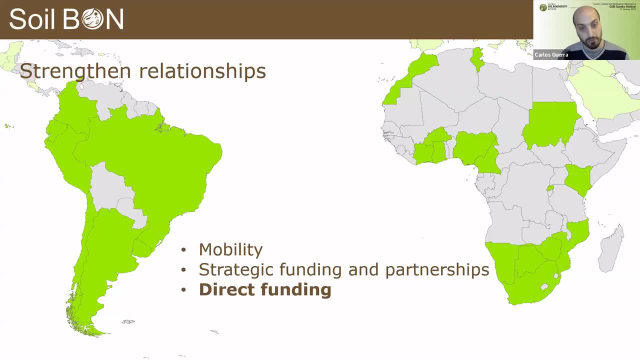 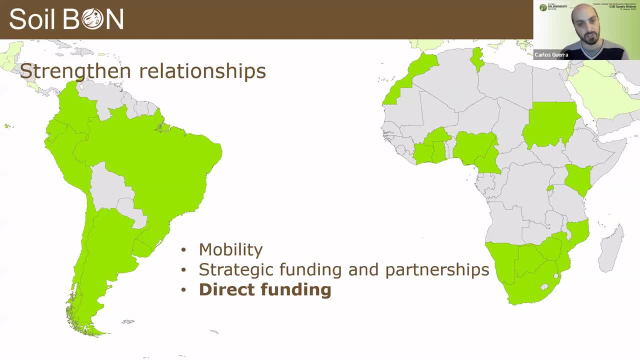 globe look at their participation into these networks in quite different ways, or they have different needs that actually block or stop completely their capacity to participate in these networks. In the case of South America, one thing that is clear to us is that issues about 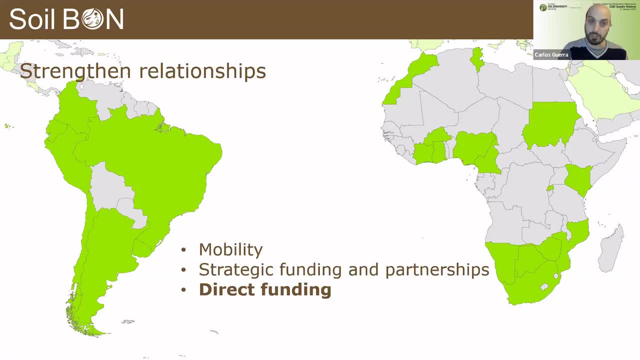 researcher mobility, for so the capacity of researchers to go outside of their country to either do other types of research or to extend the scope of their research is something that is quite important for them, And the other thing is about strategic funding and partnerships, So institutional level types of partnerships that can strengthen their local 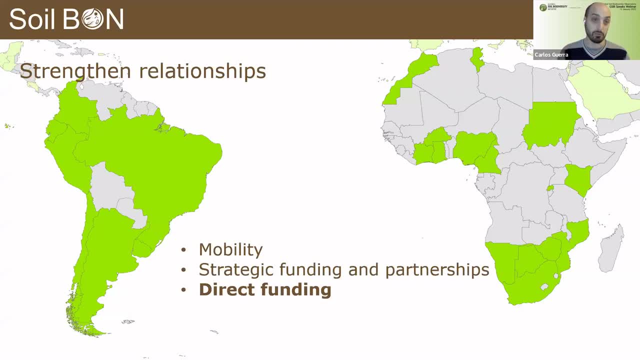 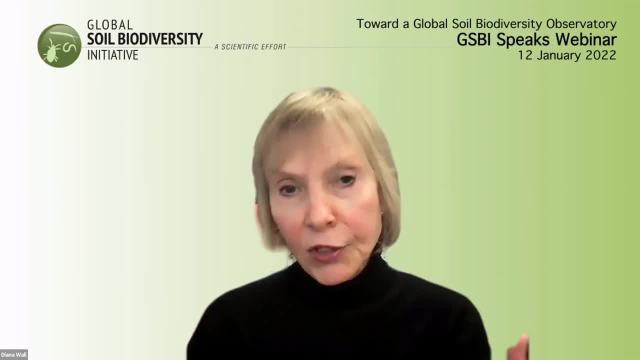 work, say in molecular analysis, and whether businesses will start up analysis and whether businesses will start up to do the DNA analysis. so businesses will start up to do the DNA analysis so that they can pick the suite to do the DNA analysis, so that they can pick the suite of indicators to tell the 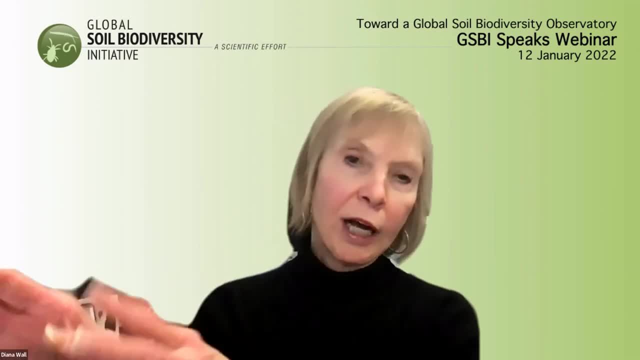 that they can pick the suite of indicators to tell the farmer- oh yeah, I. of indicators to tell the farmer- oh yeah, I know that you're going to build farmer. oh yeah, I know that you're going to build your soil here and your. 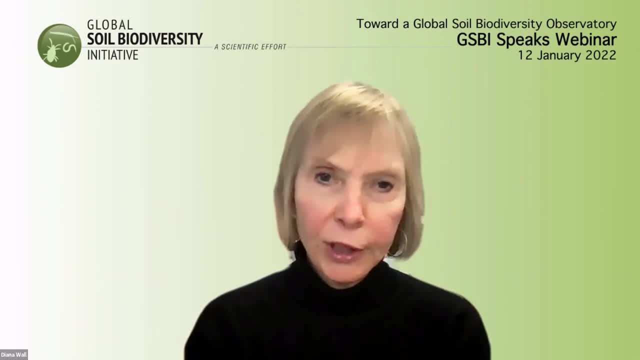 you're going to build your soil here and your soil carbon and get your soil here and your soil carbon and get your ecosystem services. So I think your soil carbon and get your ecosystem services. So I think there's a lot of ecosystem services, So I think there's a lot of targets of ecosystem services. 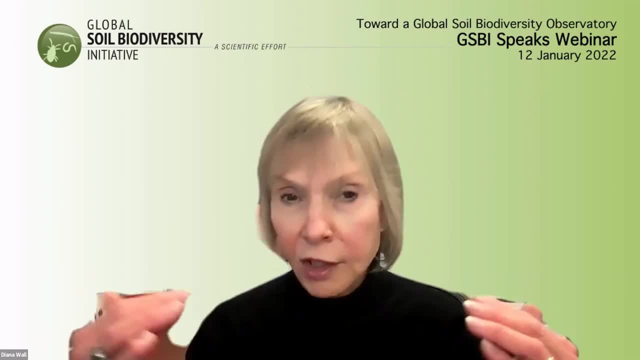 there's a lot of targets of ecosystem services. There's the economics of it. targets of ecosystem services. There's the economics of it, whether a small-scale- There's the economics of it whether a small-scale farmer can pay to get the. whether a small-scale farmer can pay to get the indicators that a larger-scale 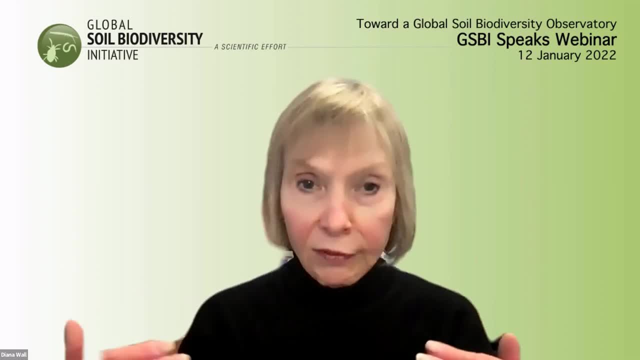 farmer can pay to get the indicators that a larger-scale farmer can and has farmer can and has the funding for. So I think there are a lot of issues the funding for. So I think there are a lot of issues embedded in indicators. embedded in indicators that people are looking at And so they may have it. that people are looking at, And so they may have it for a region or for a for a region or for a climate or for a changing climate, But I don't know climate or for a changing climate, But I don't know if they're going to have 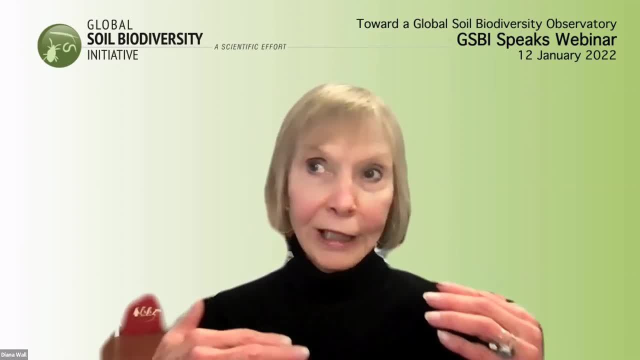 climate or for a changing climate, But I don't know if they're going to have a specific global climate or if they're going to have a global climate, a specific global climate. But I don't know if they're going to have a specific global climate, But I don't know if they're going to have a 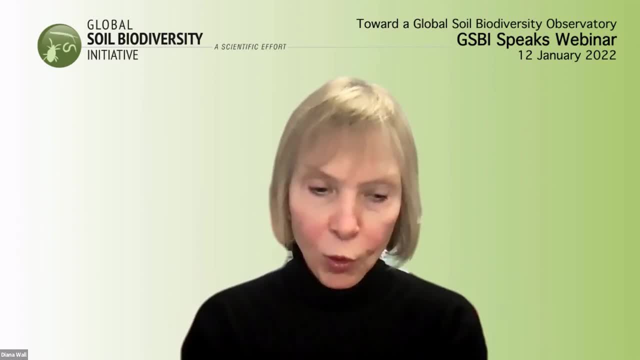 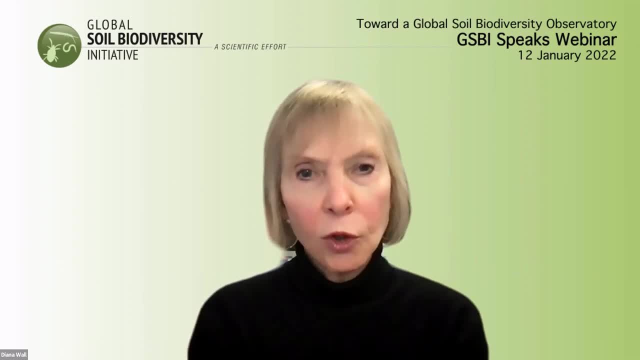 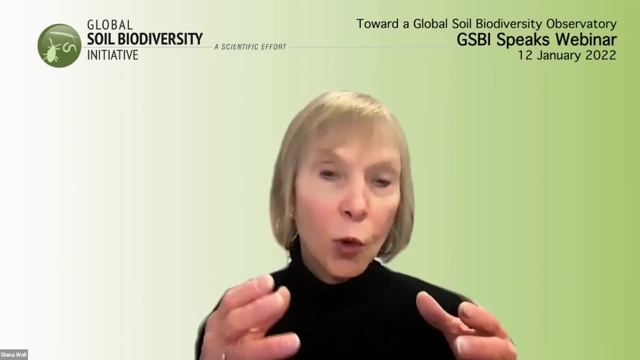 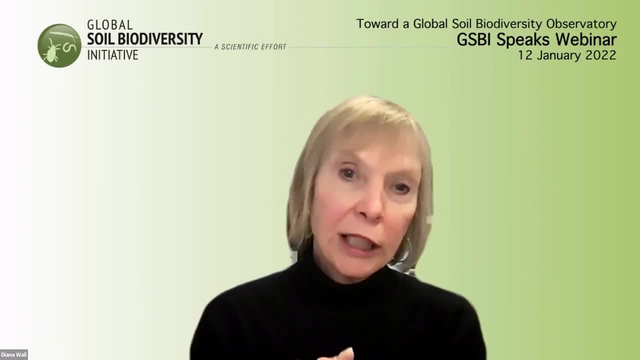 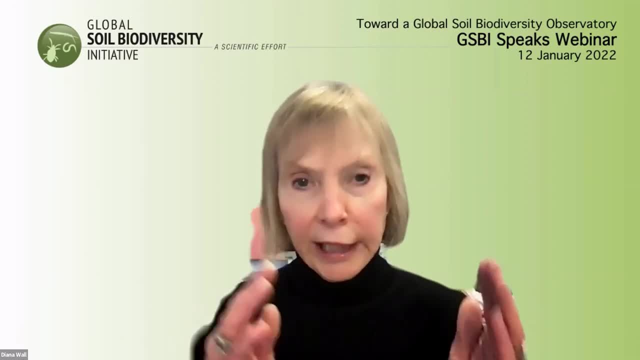 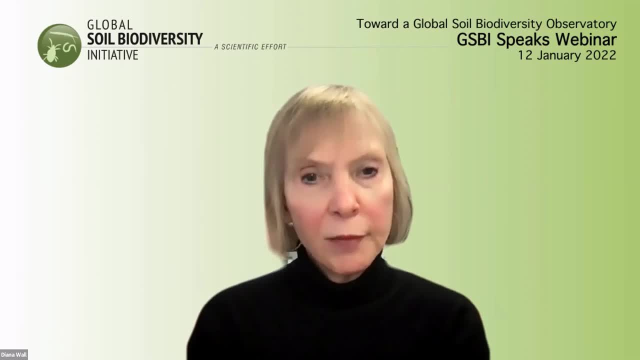 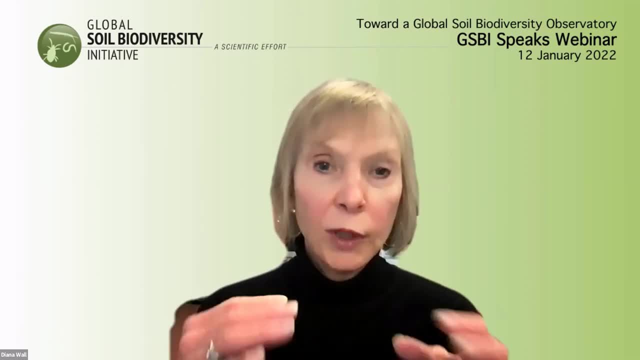 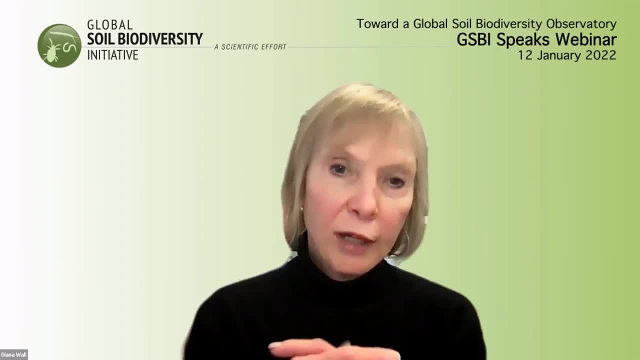 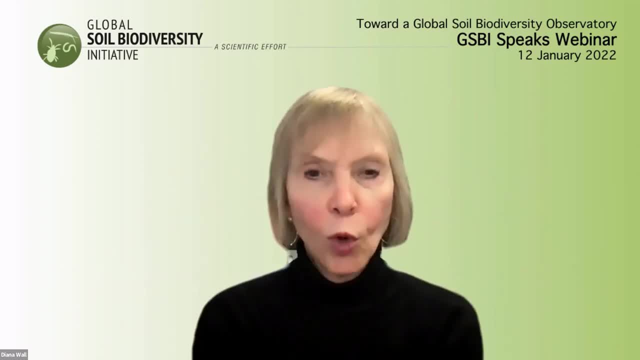 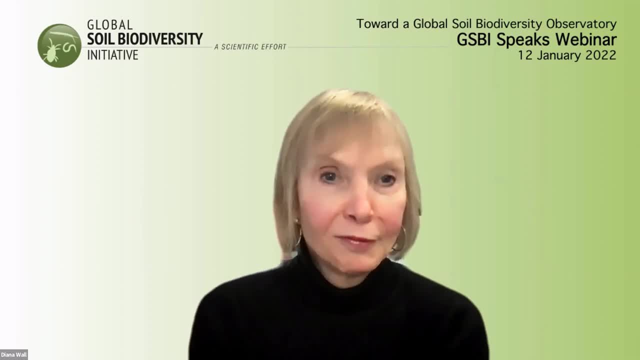 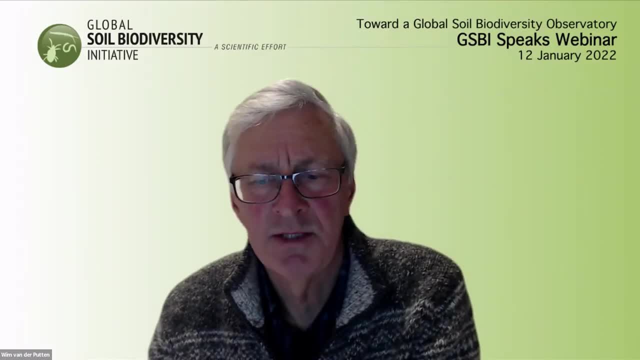 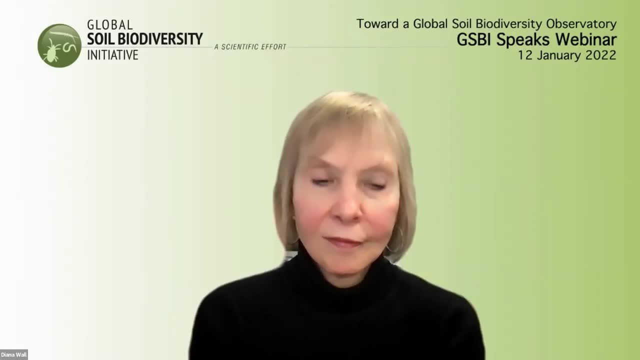 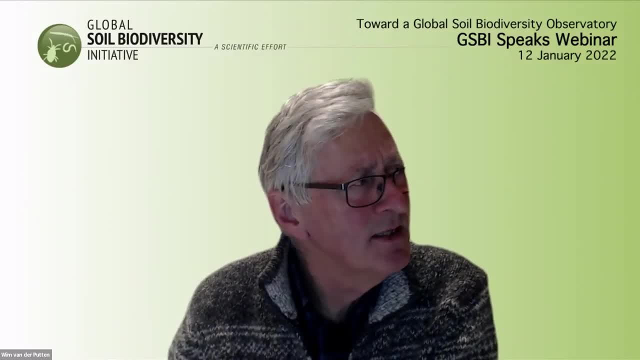 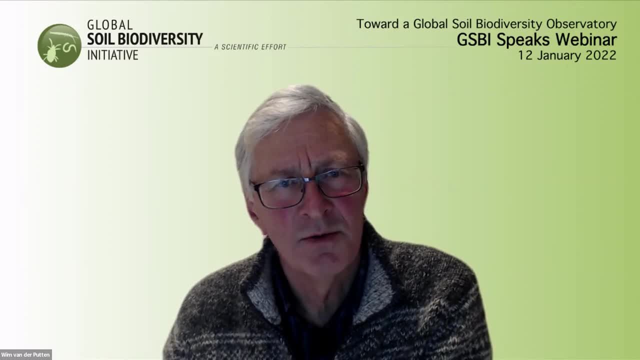 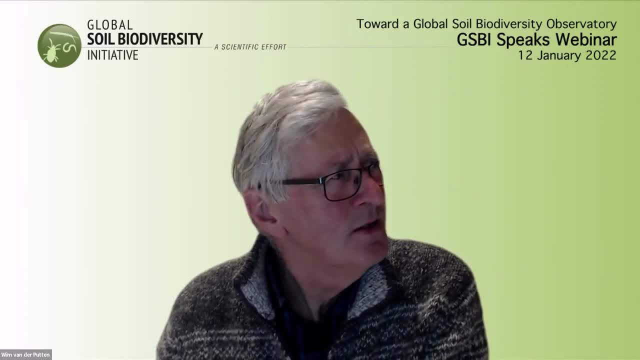 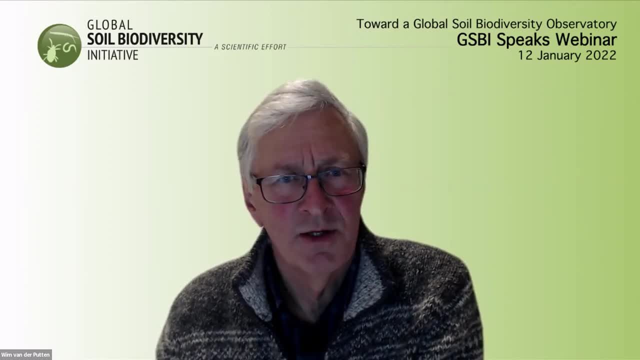 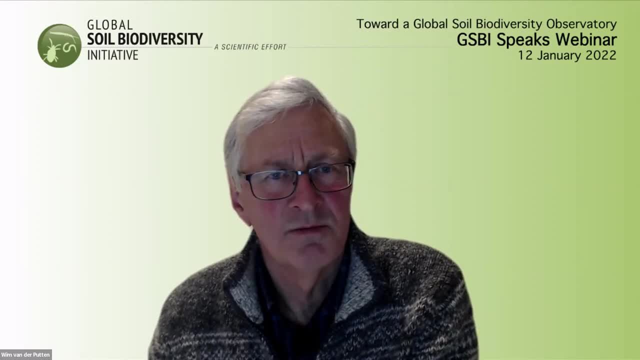 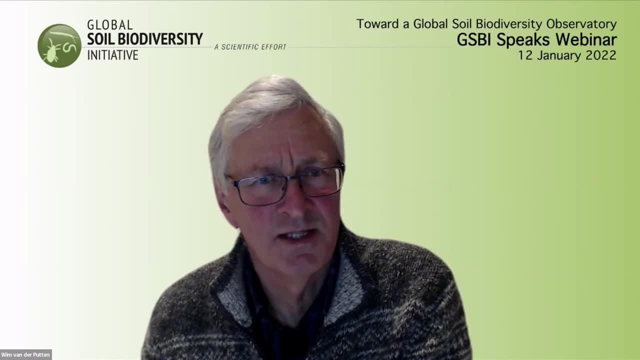 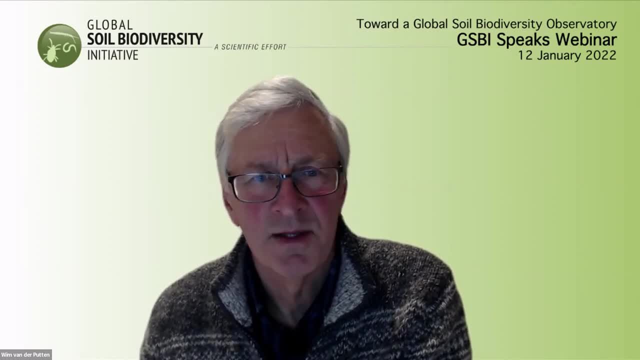 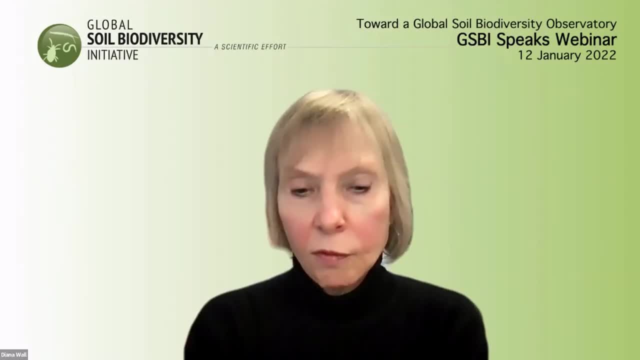 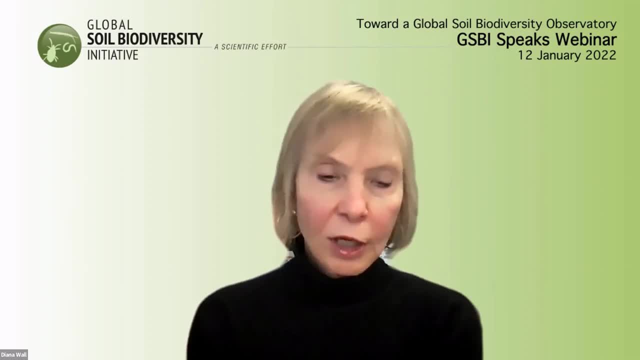 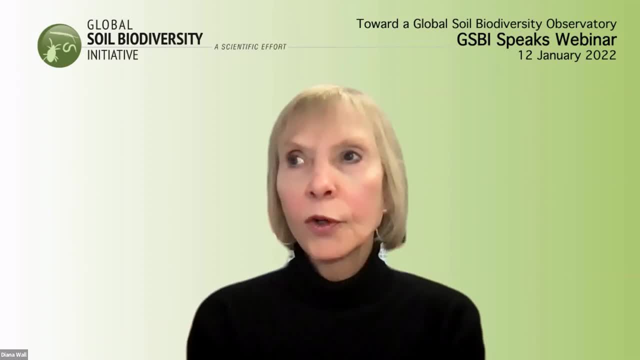 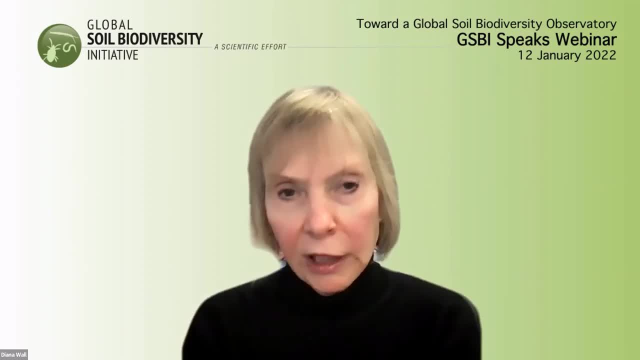 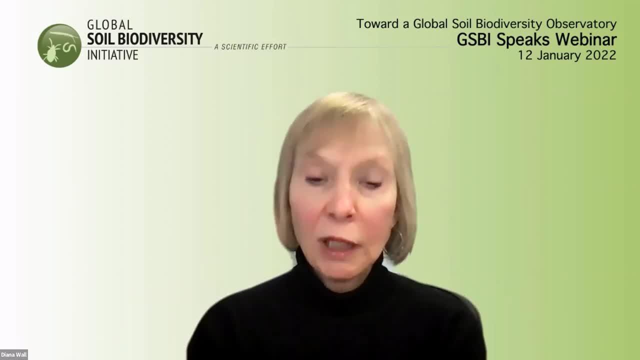 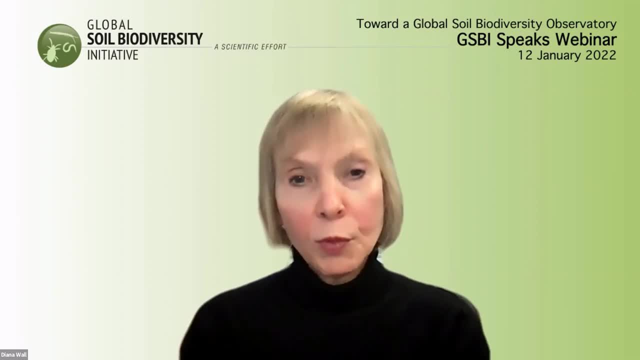 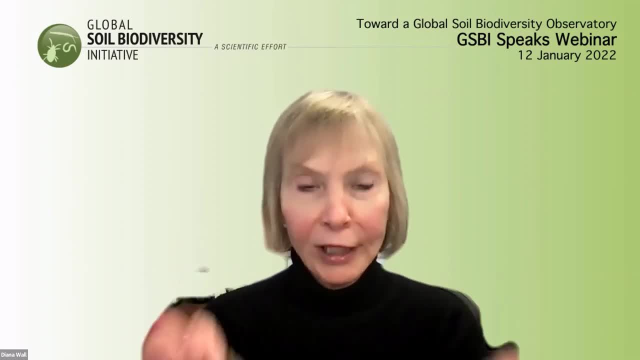 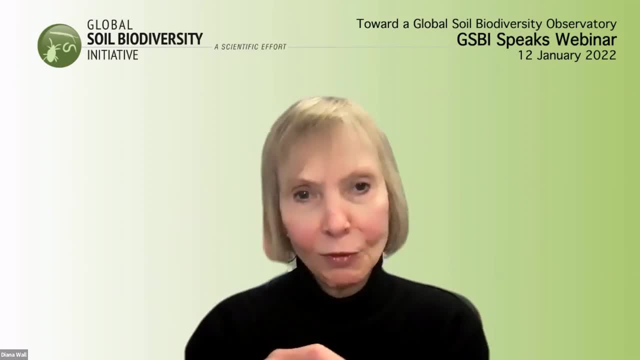 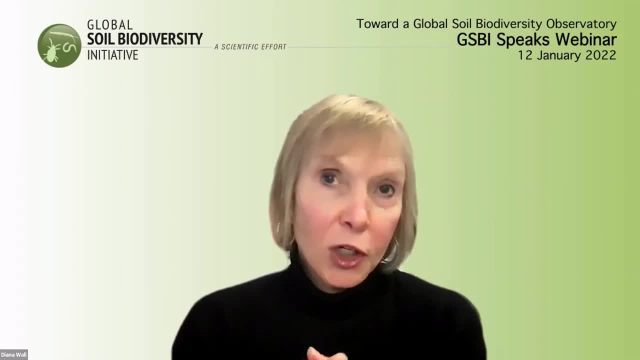 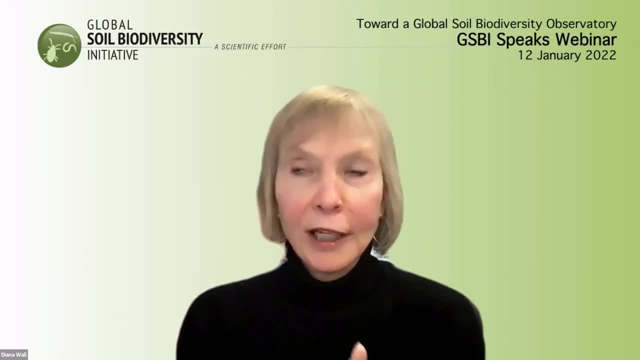 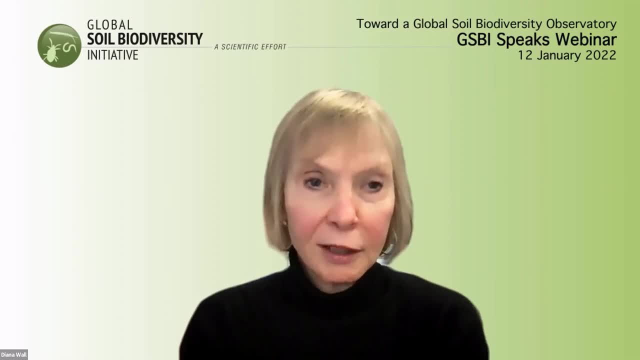 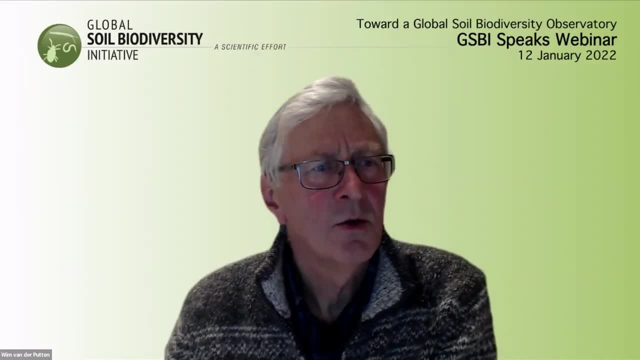 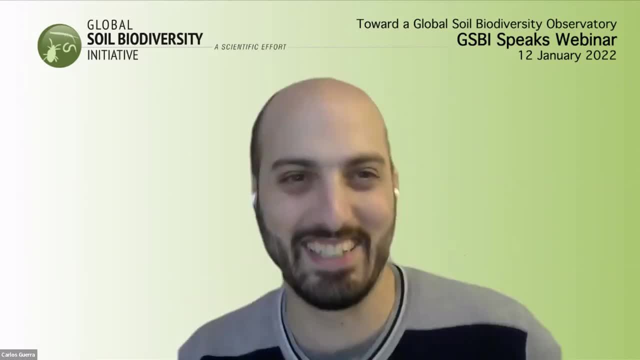 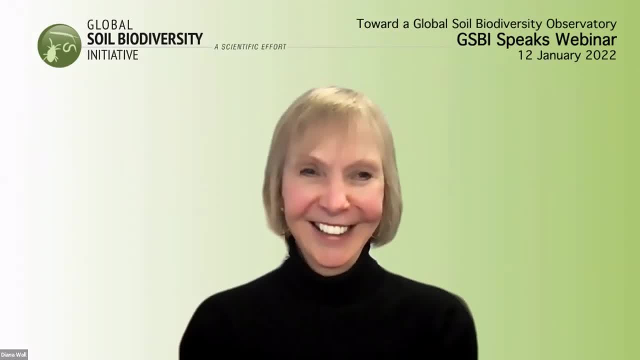 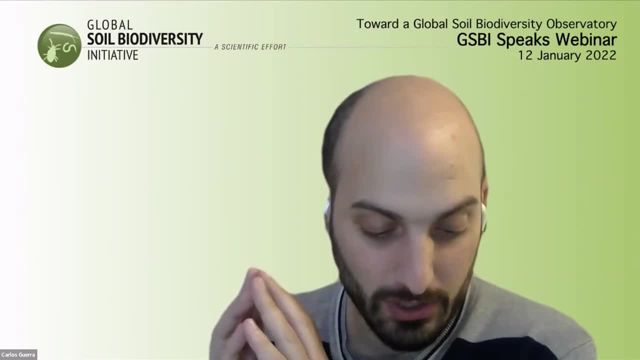 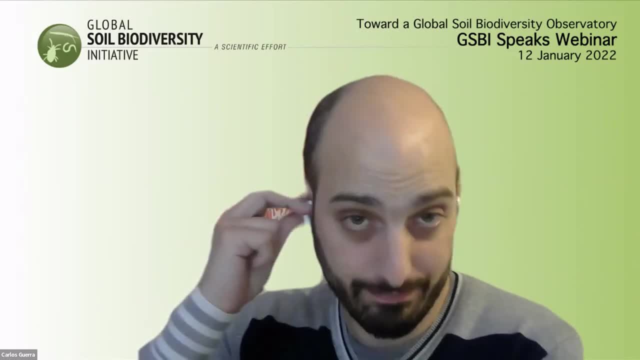 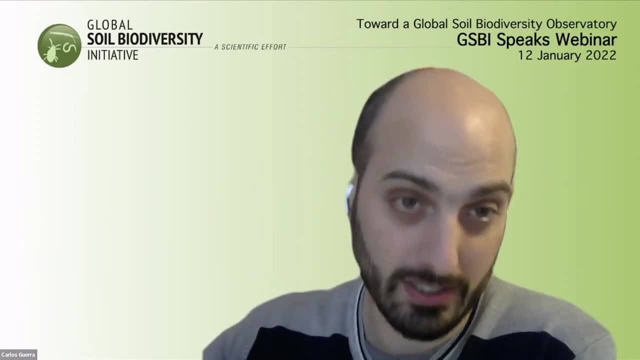 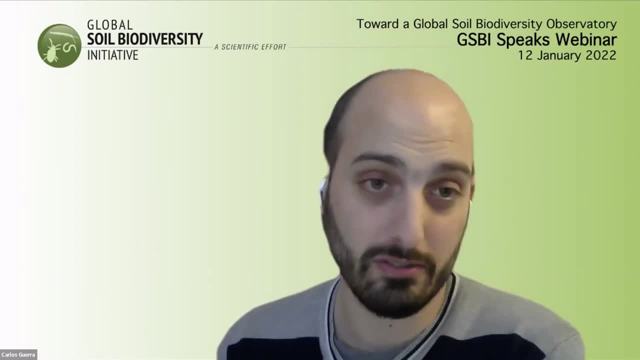 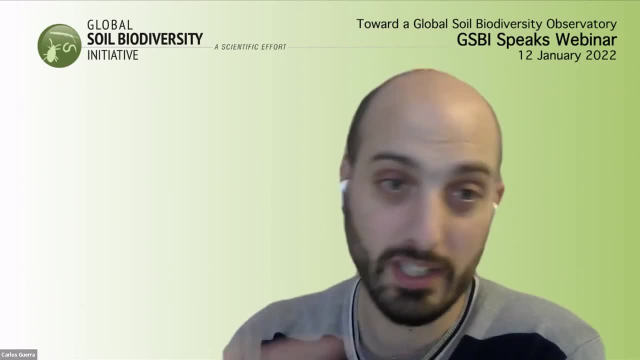 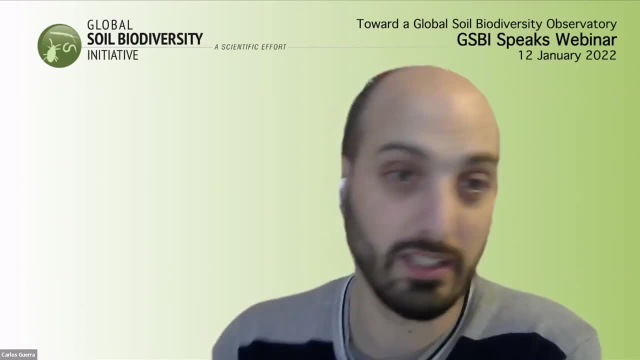 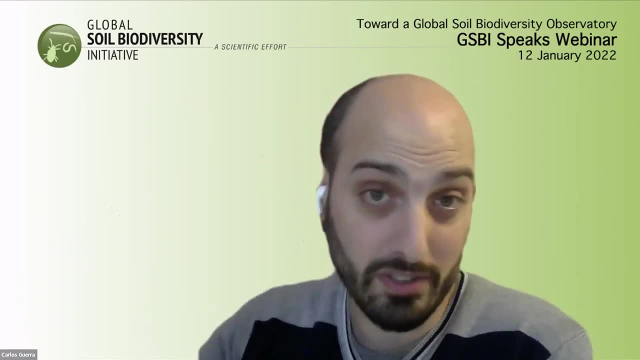 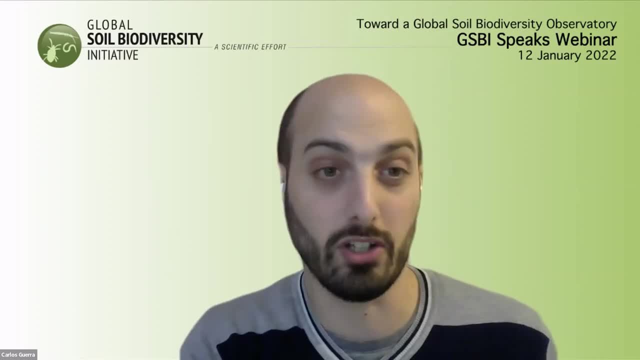 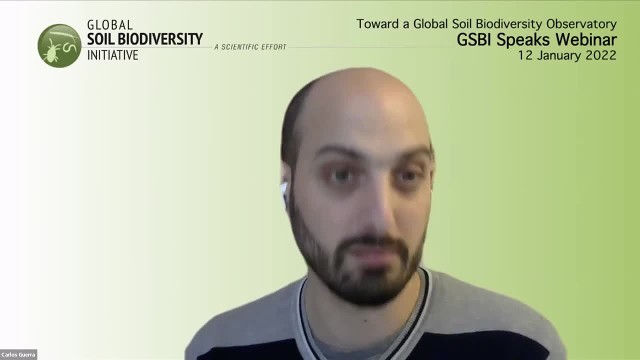 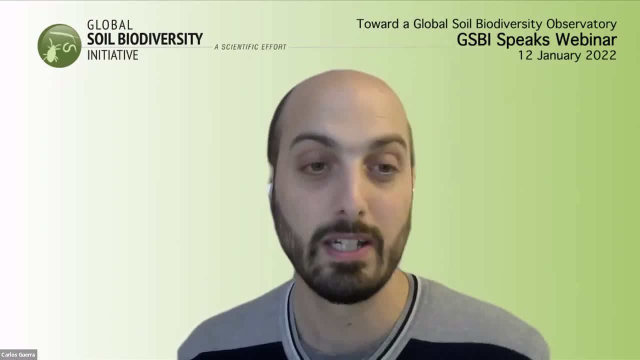 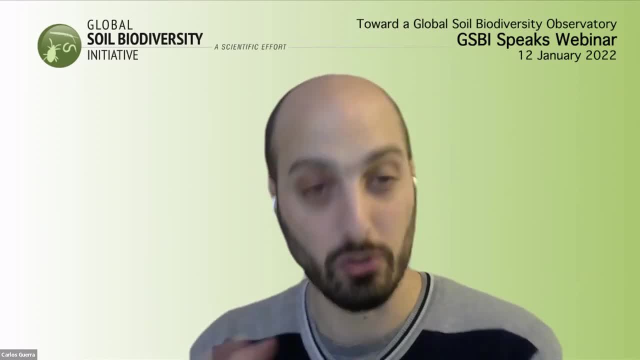 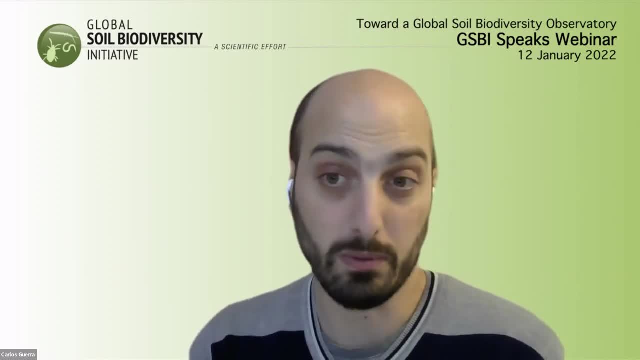 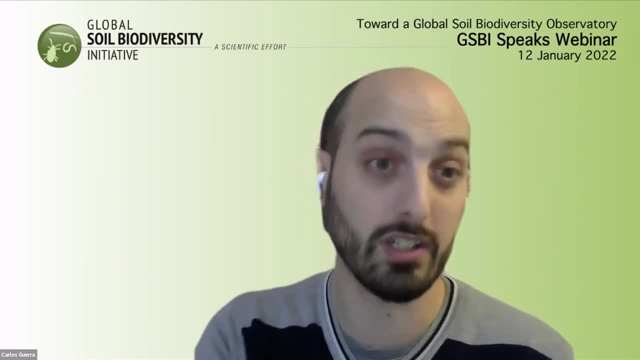 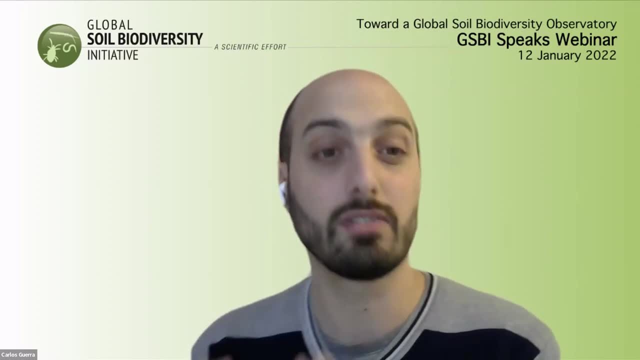 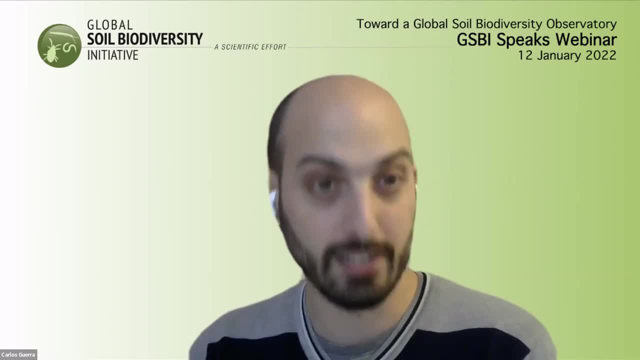 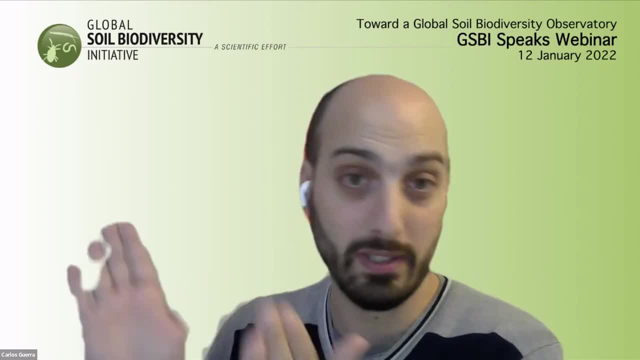 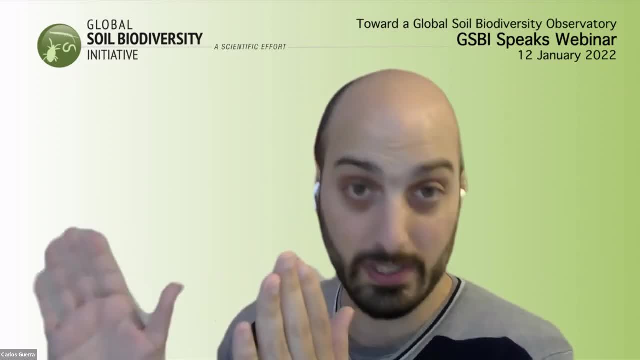 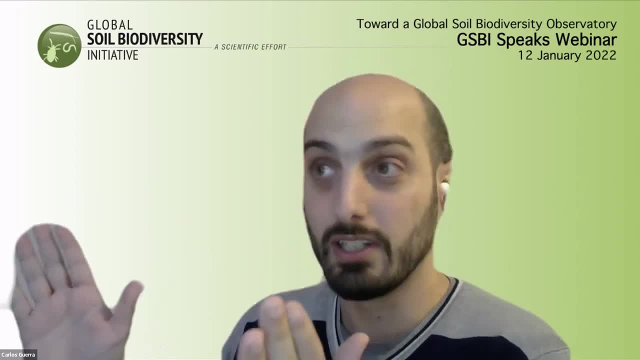 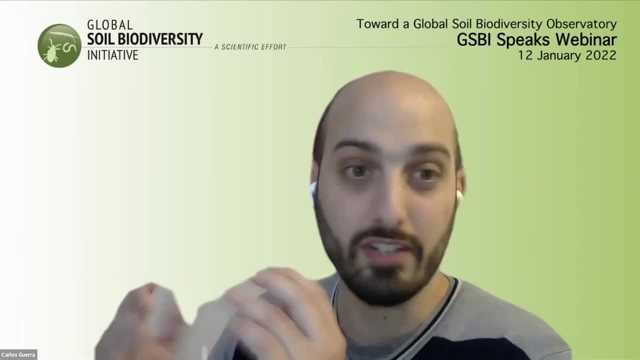 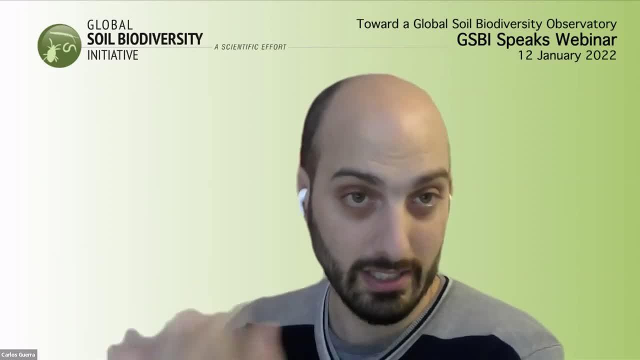 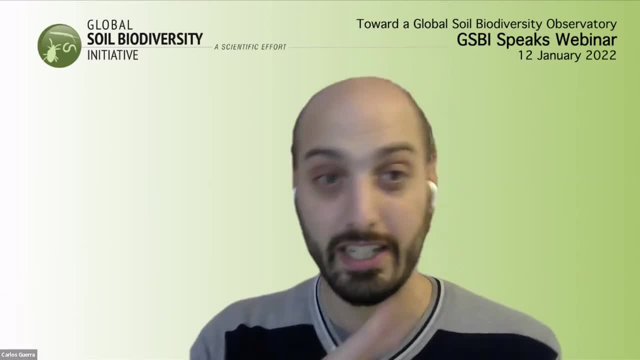 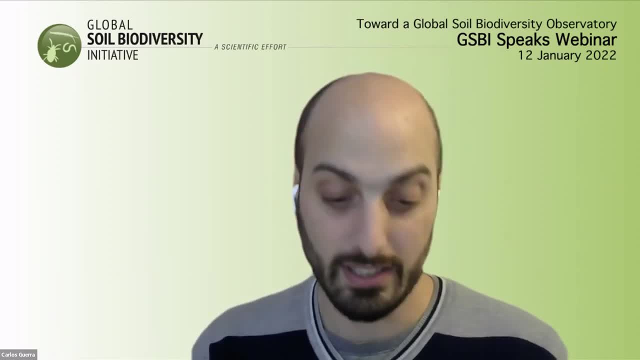 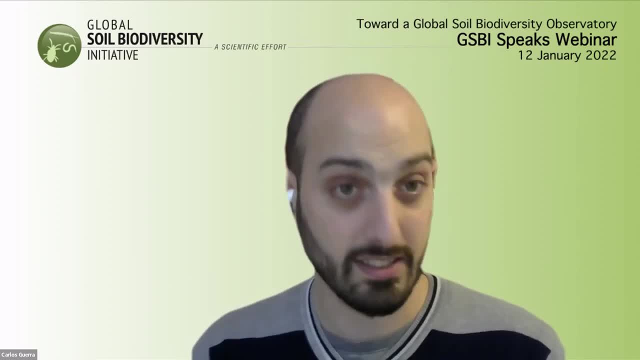 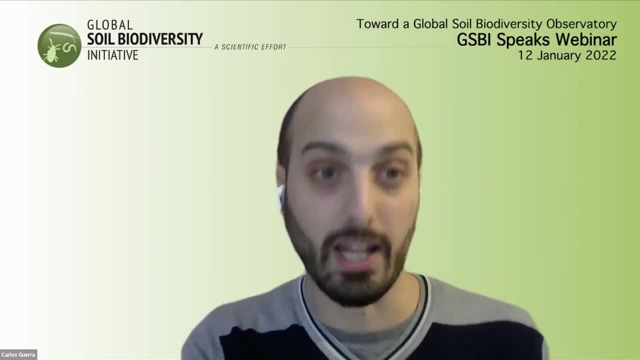 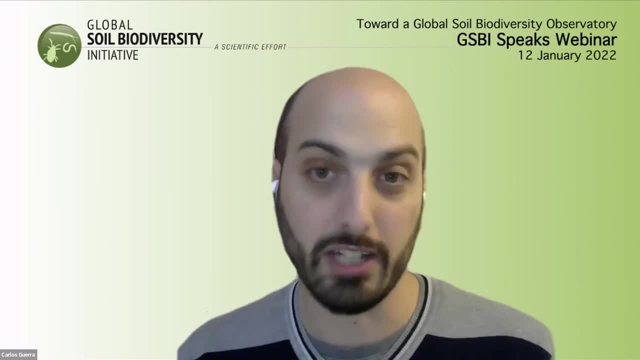 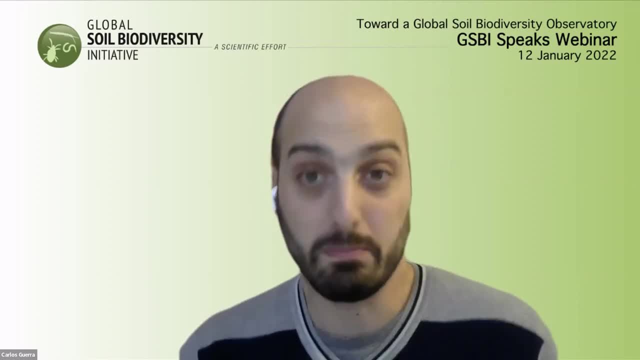 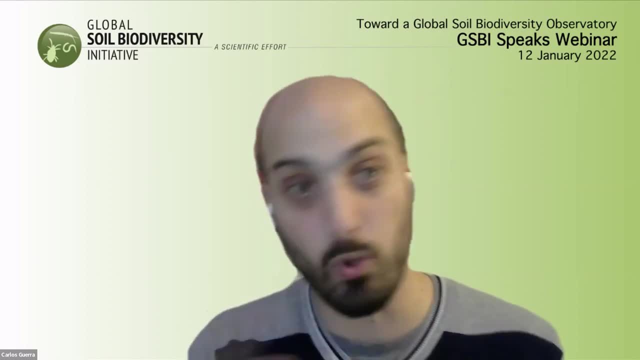 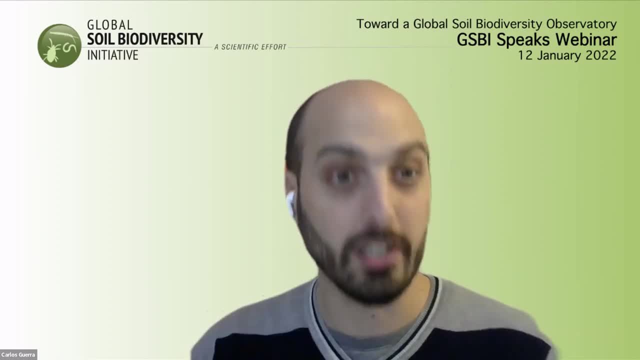 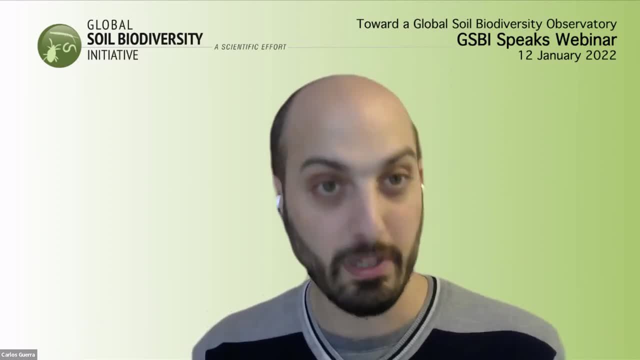 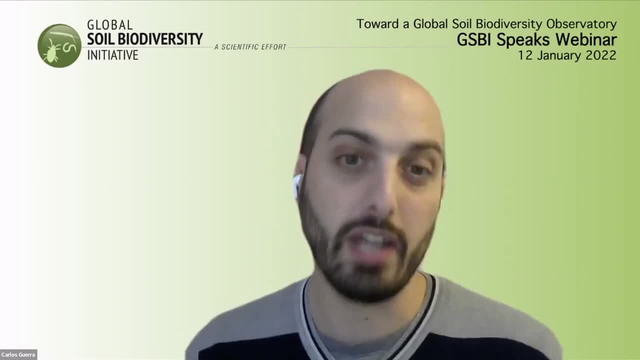 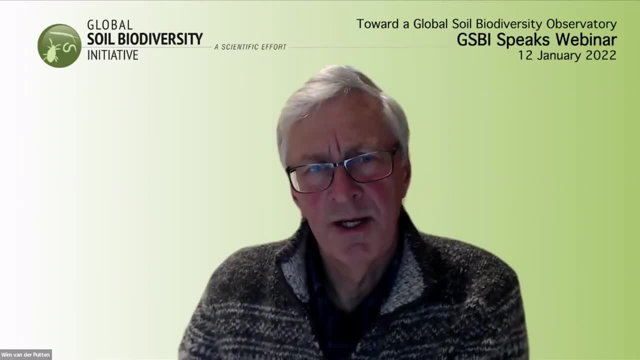 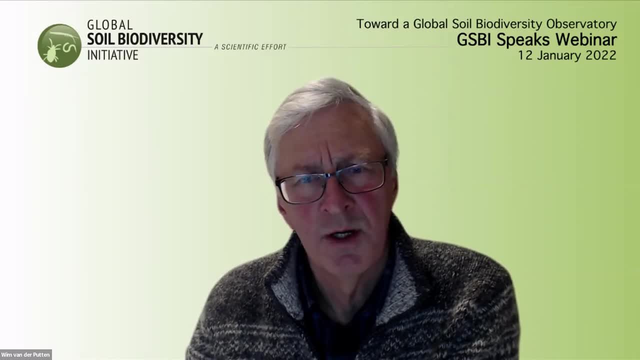 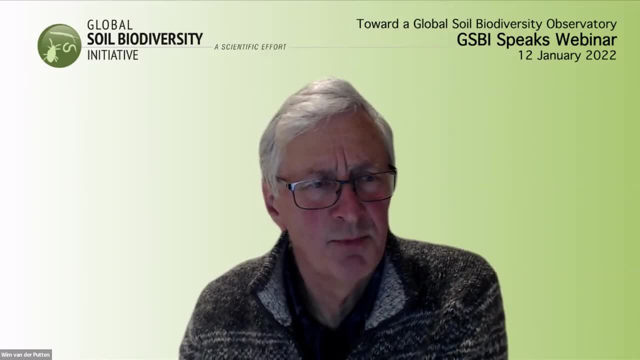 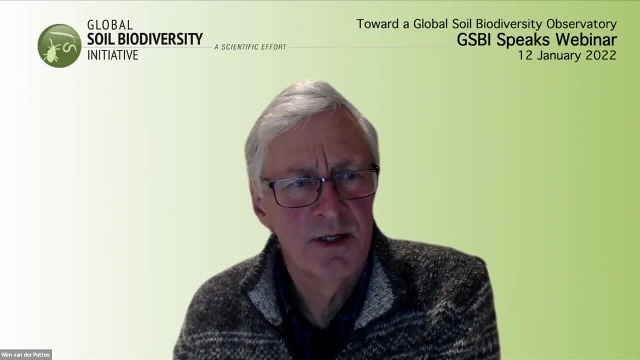 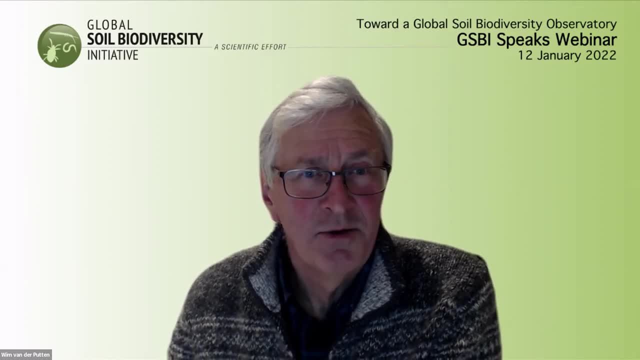 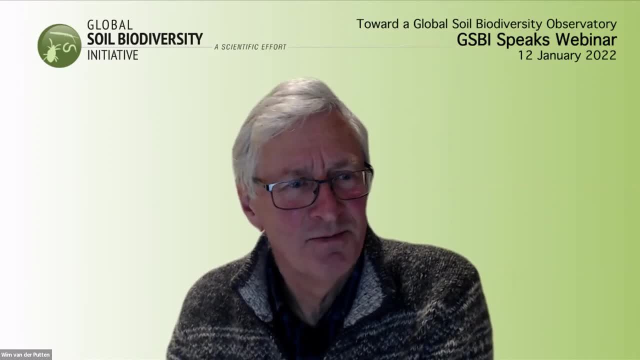 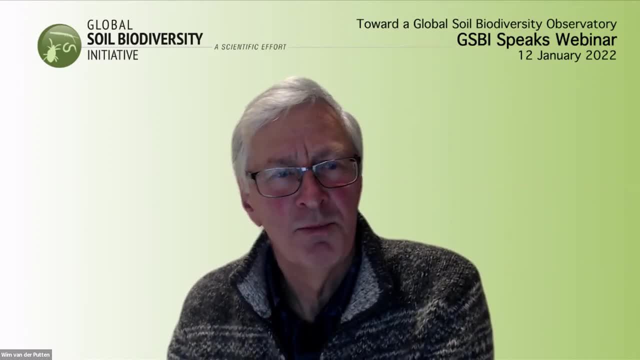 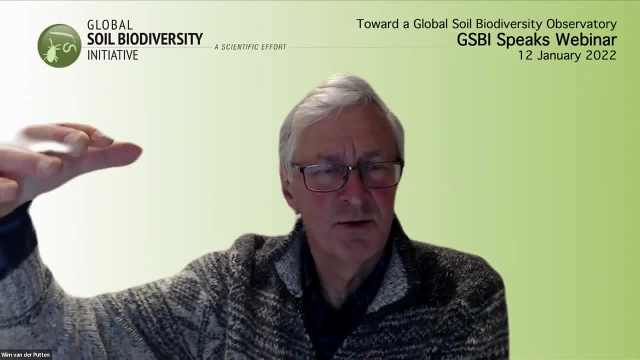 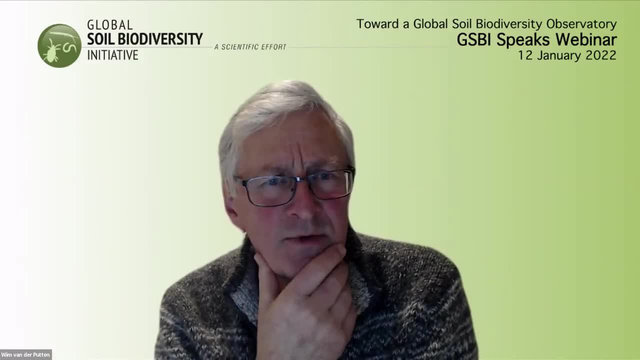 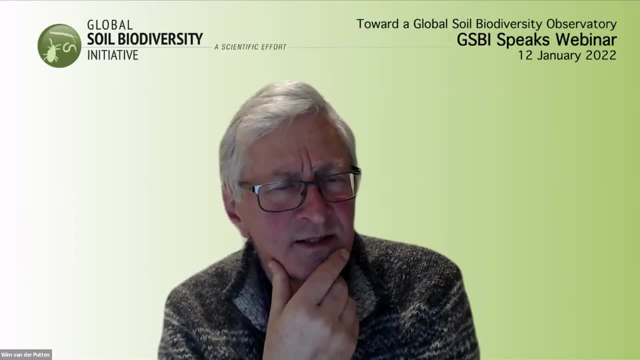 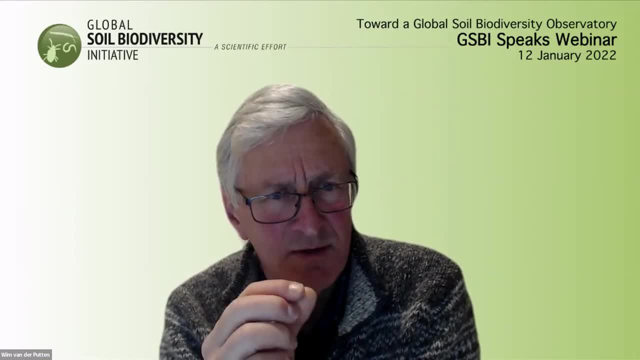 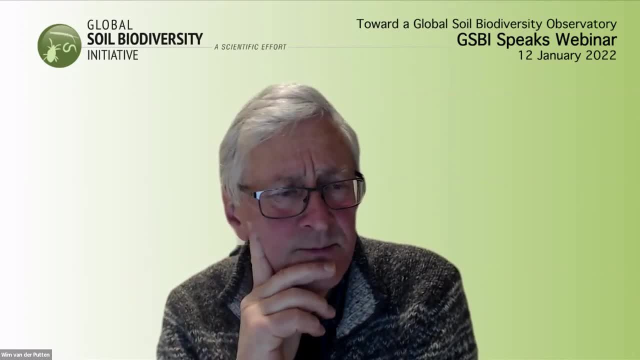 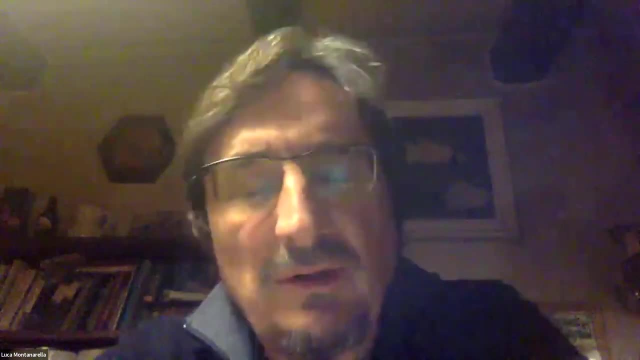 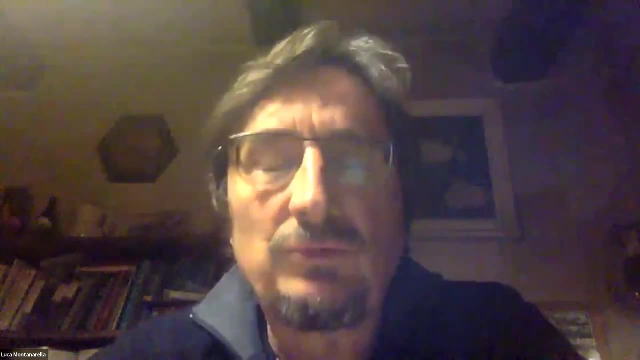 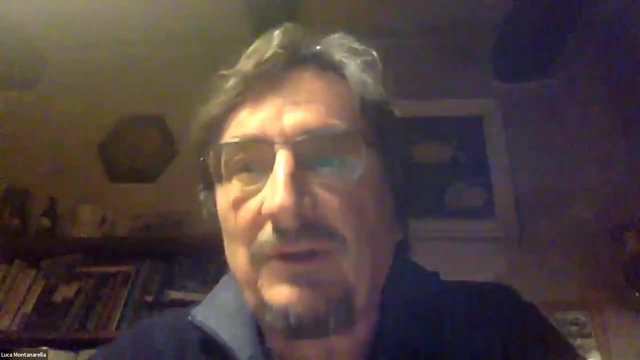 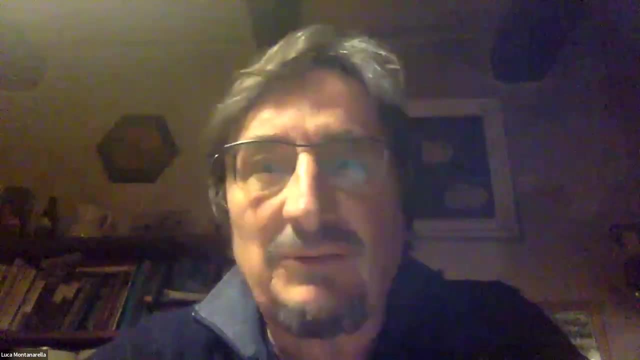 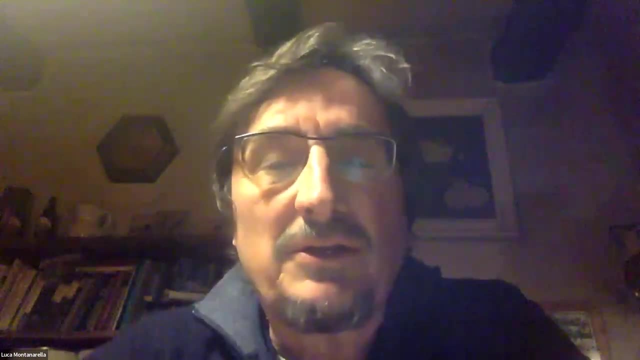 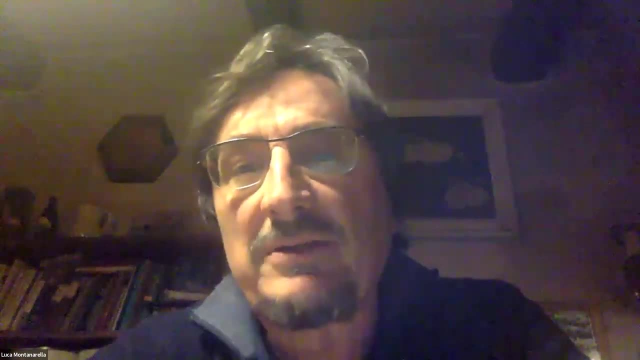 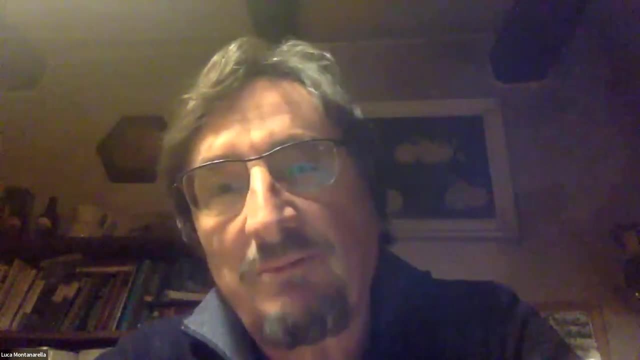 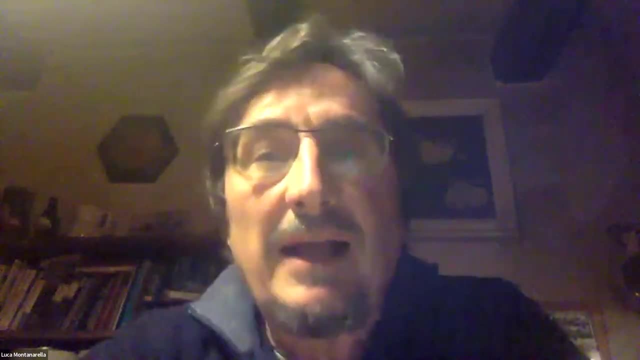 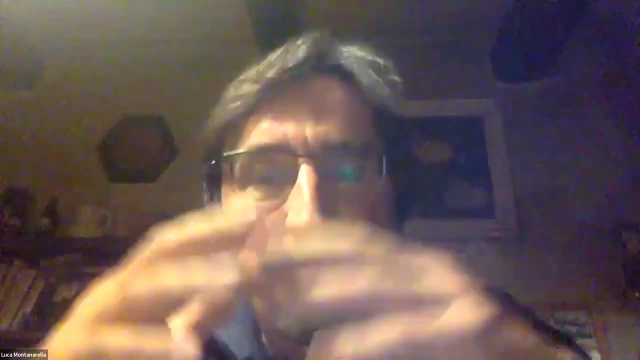 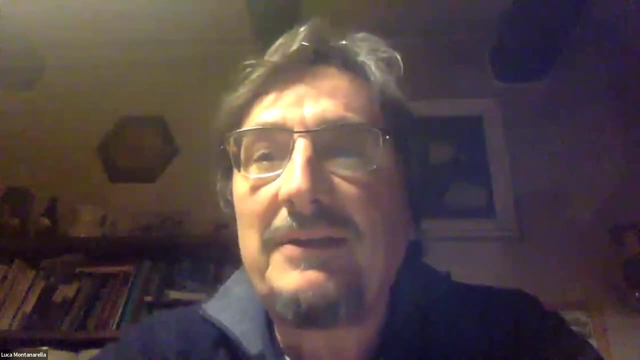 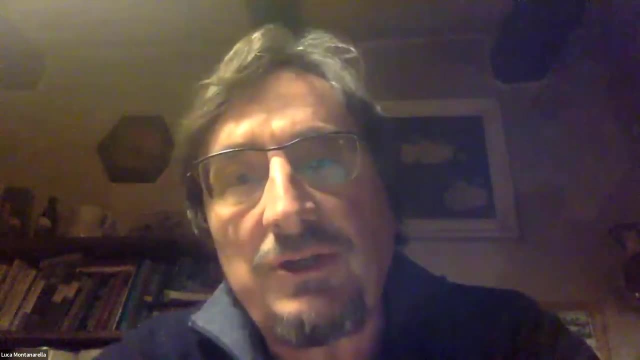 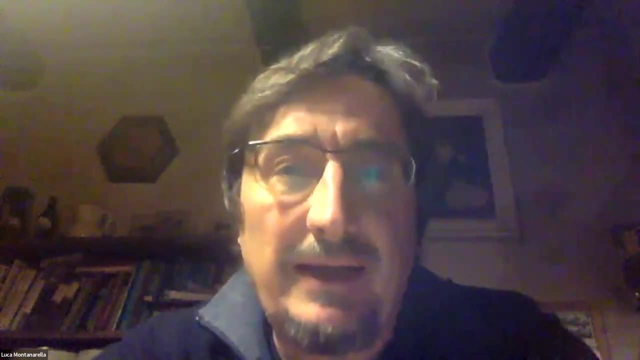 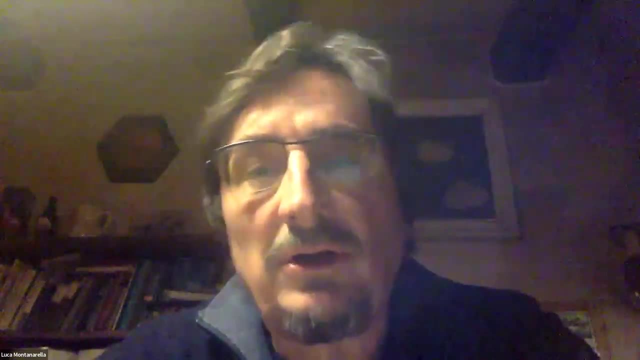 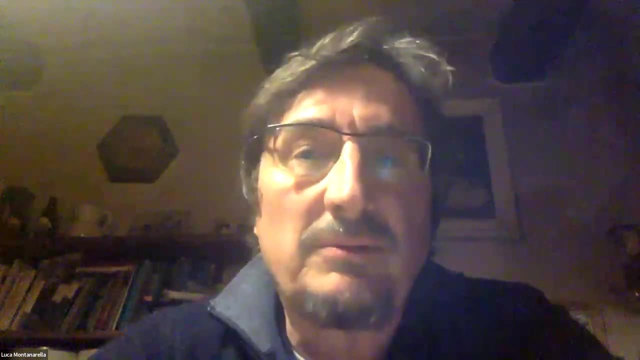 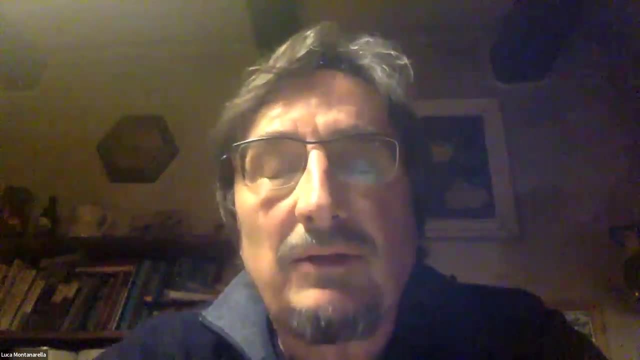 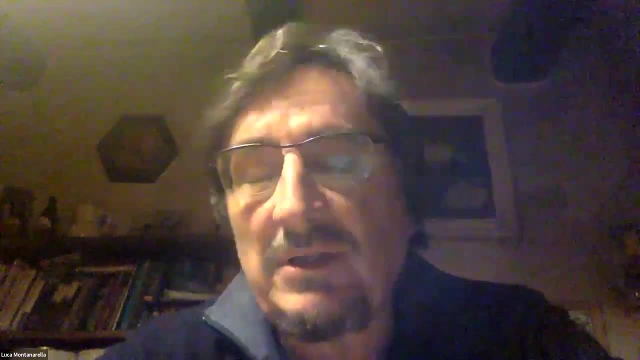 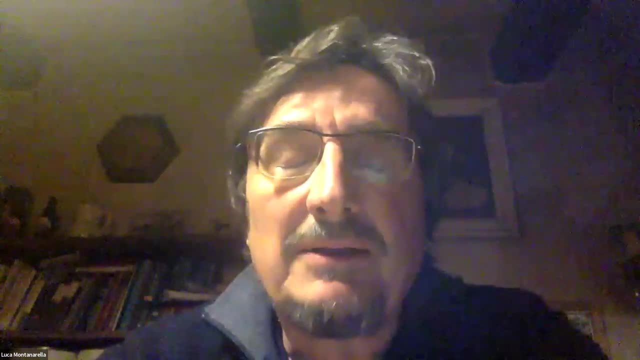 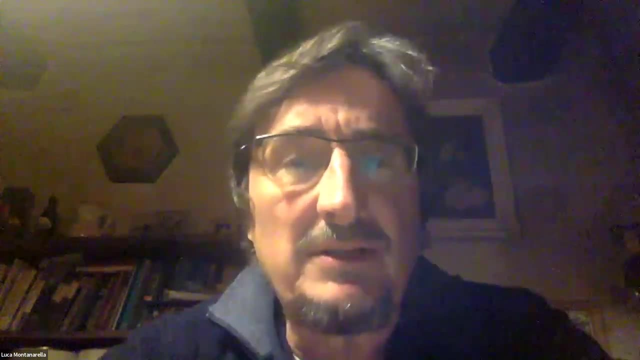 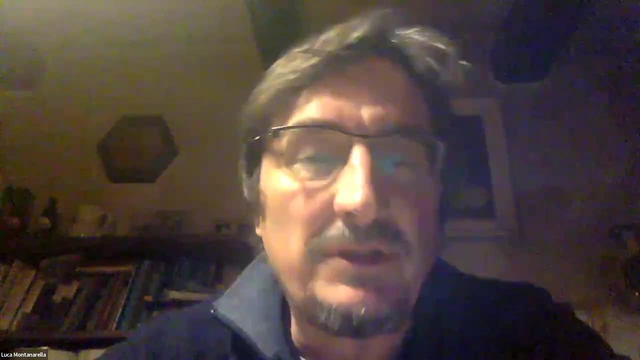 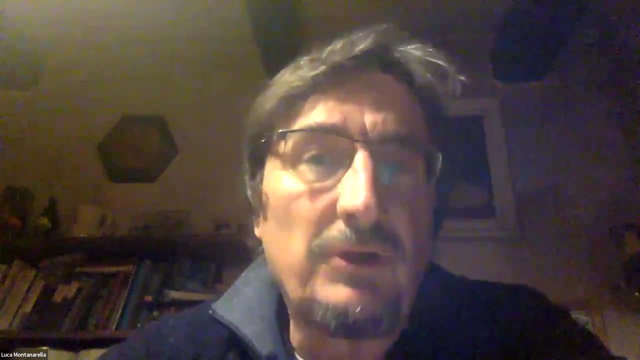 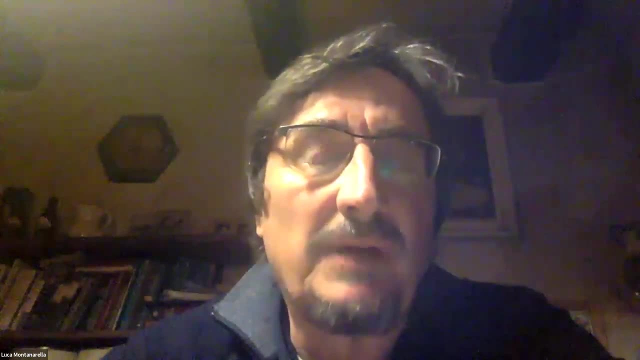 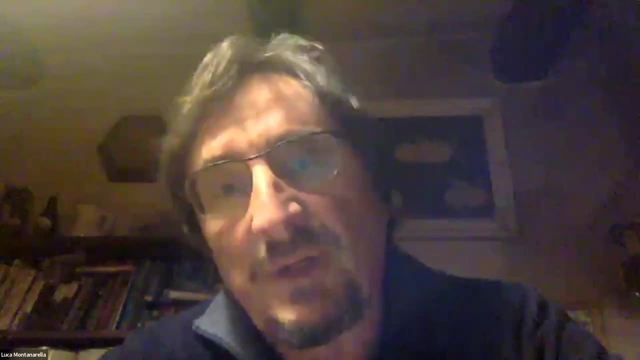 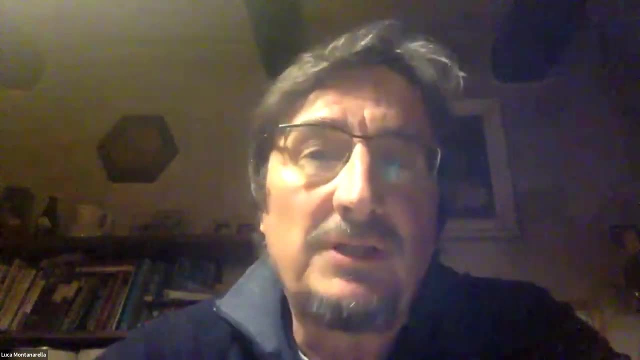 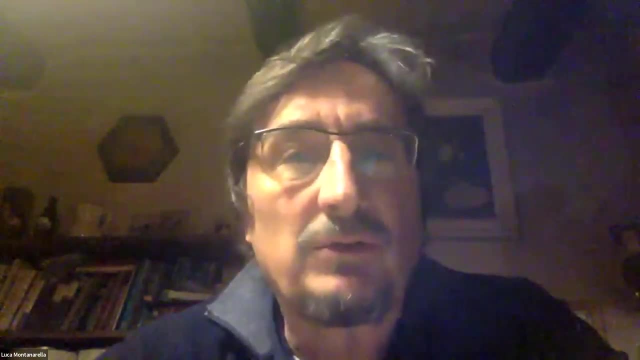 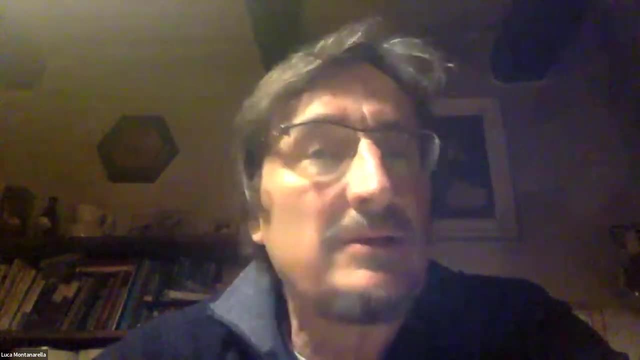 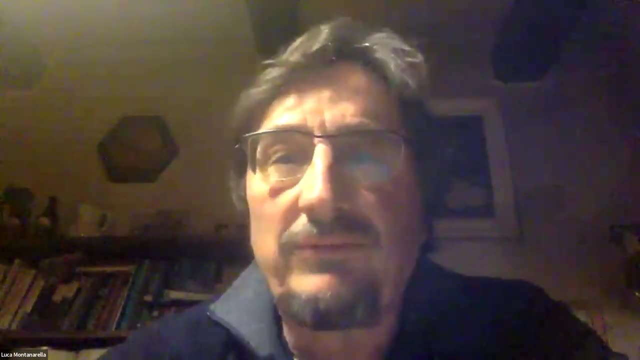 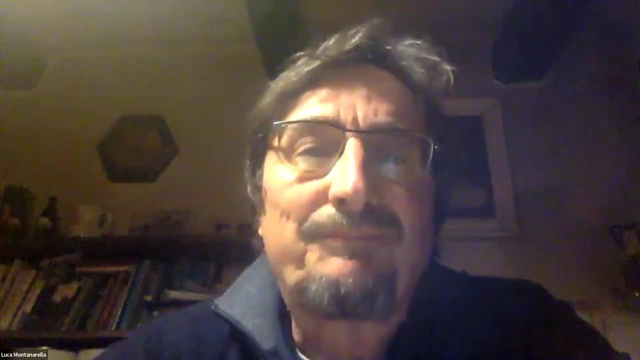 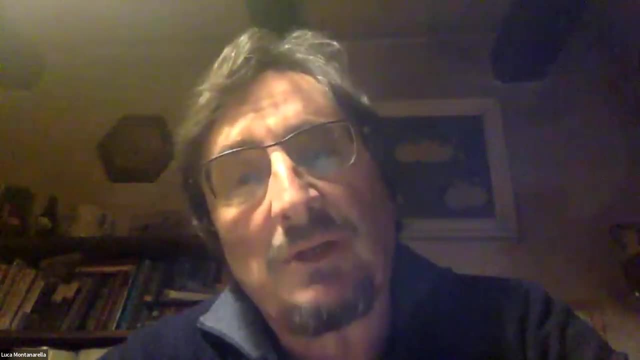 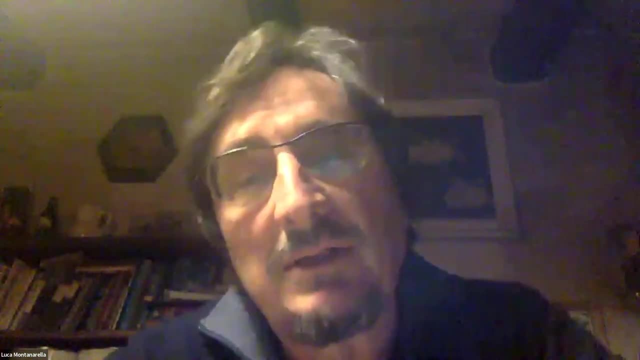 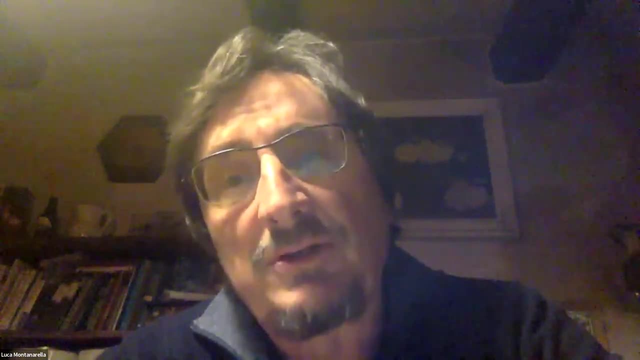 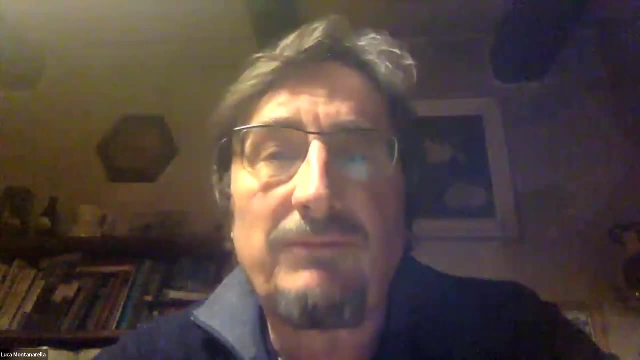 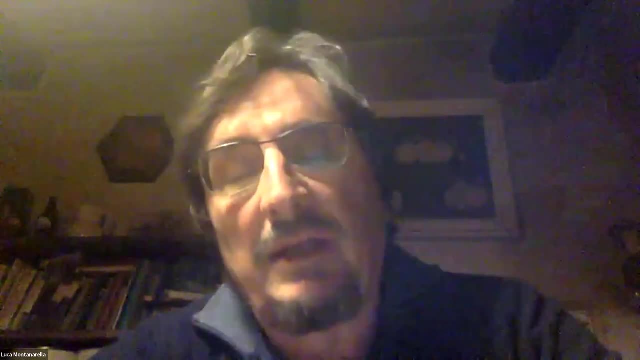 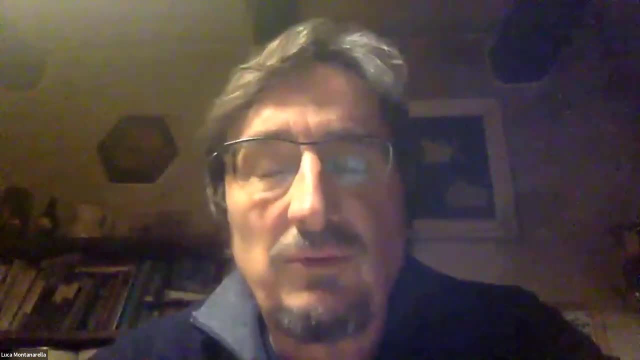 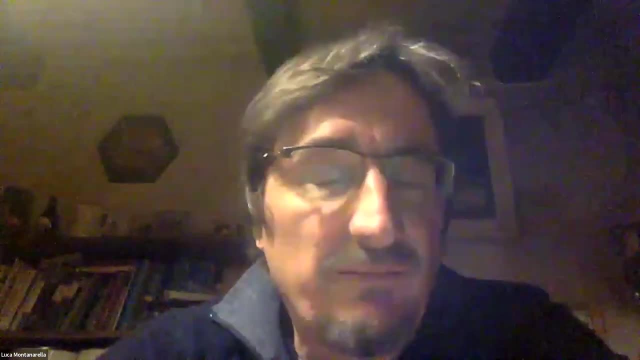 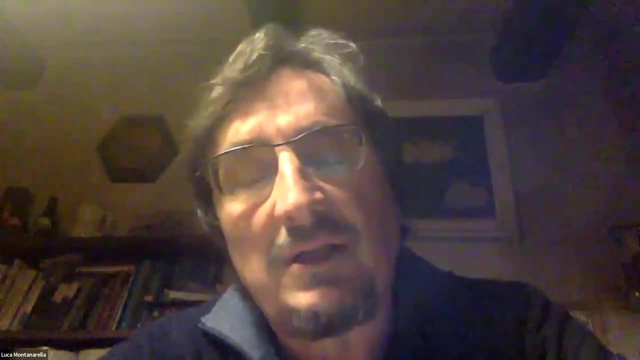 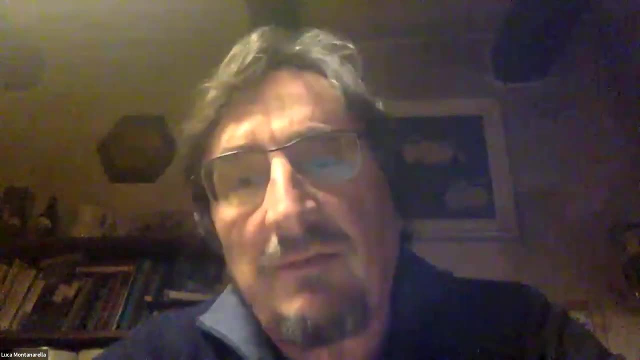 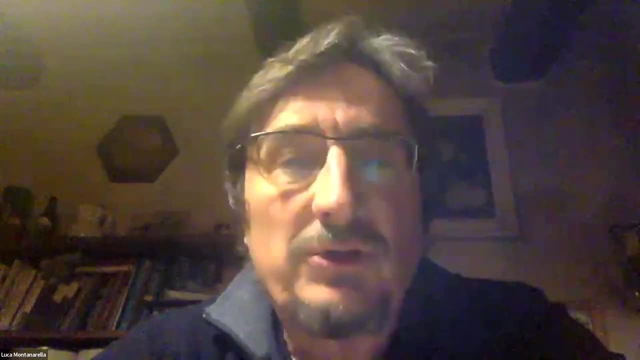 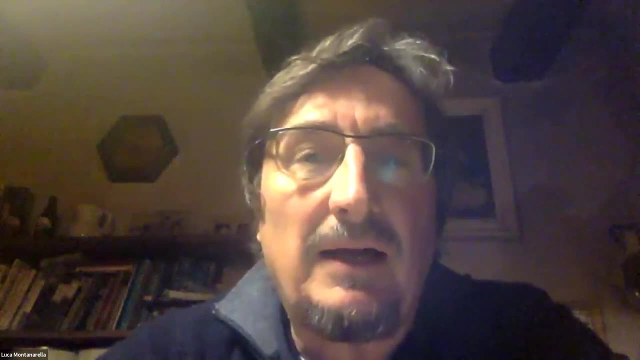 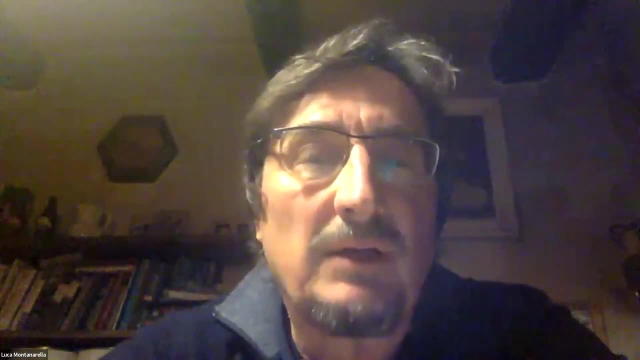 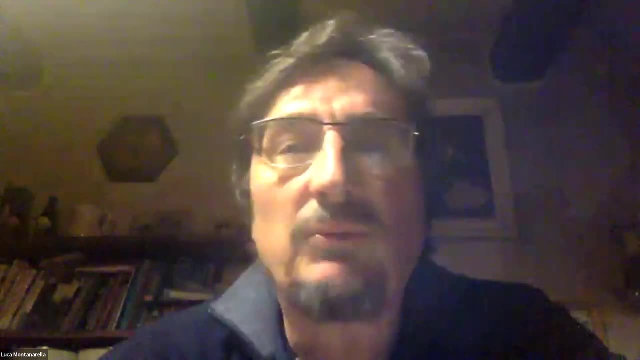 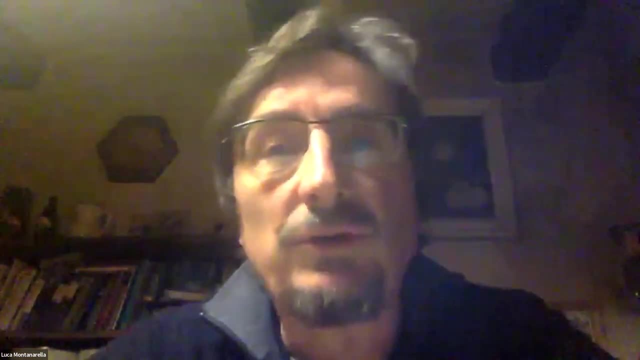 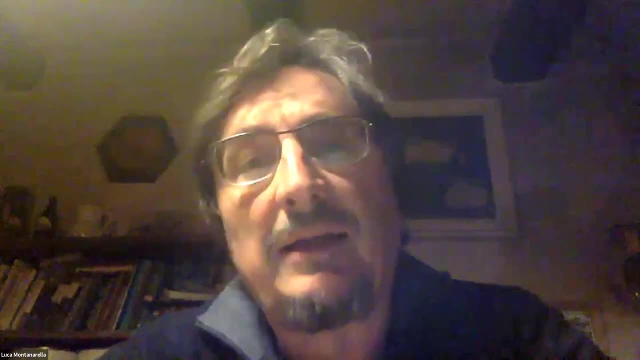 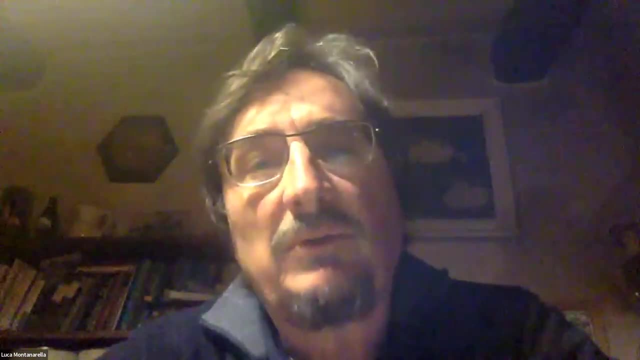 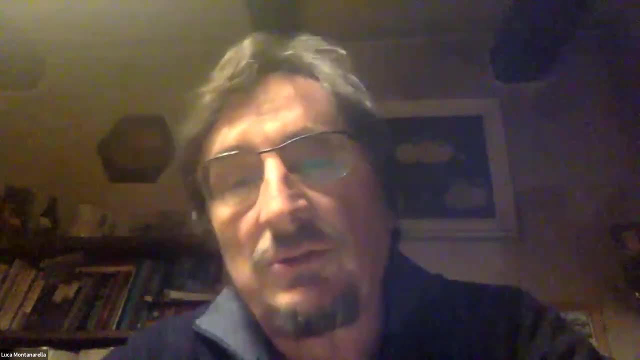 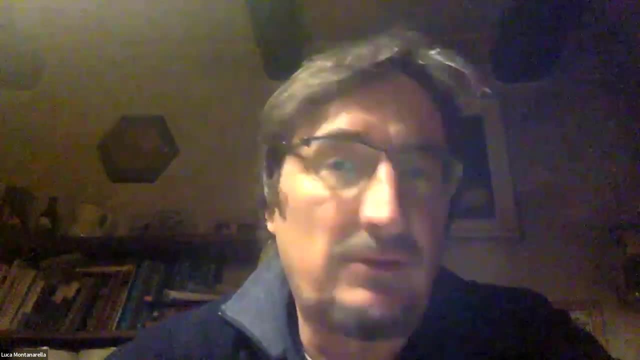 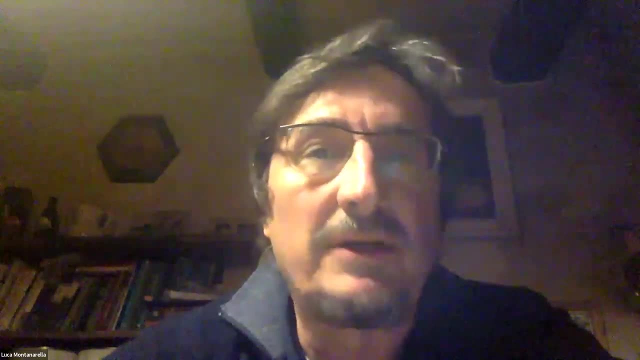 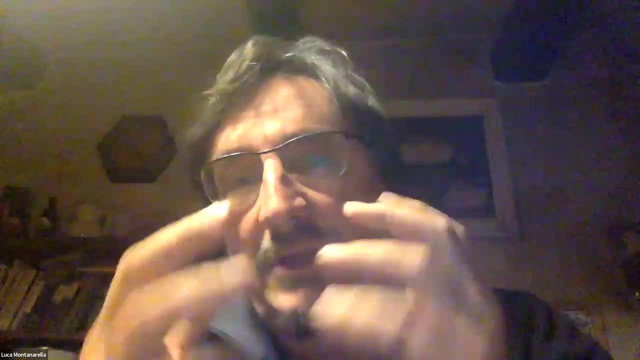 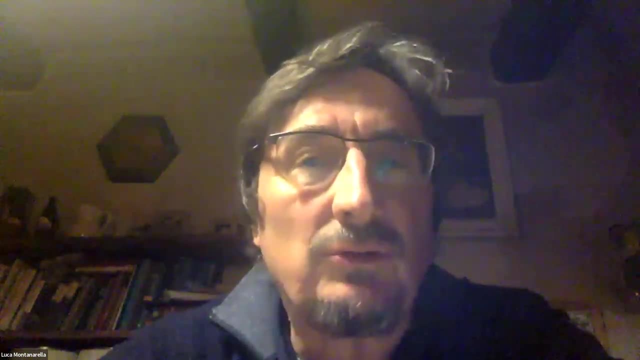 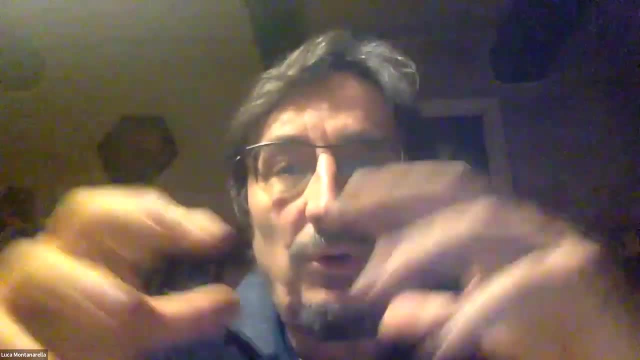 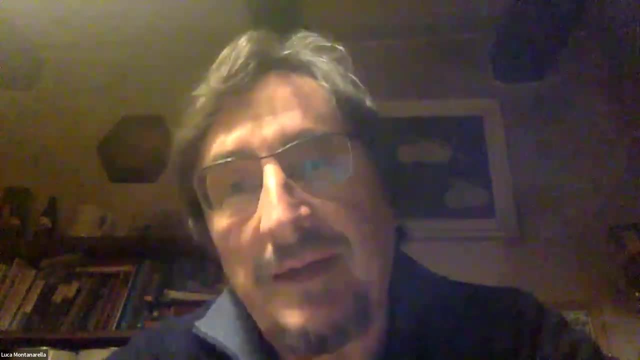 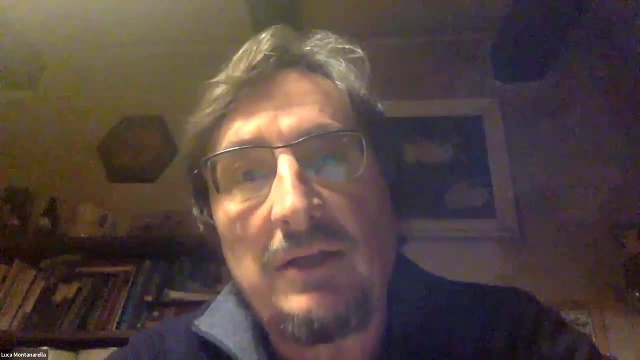 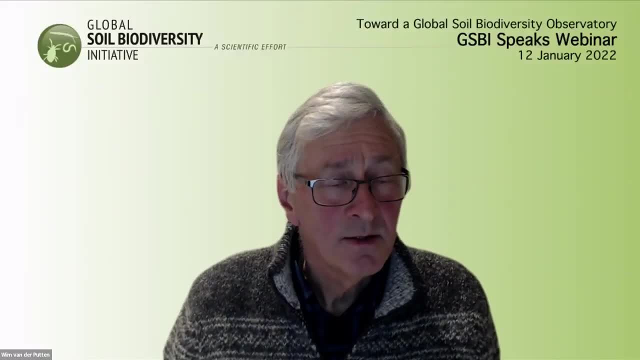 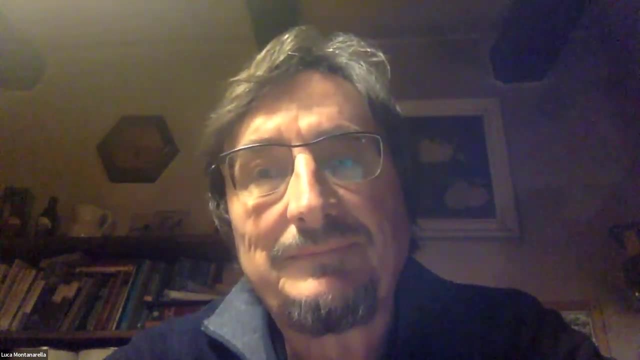 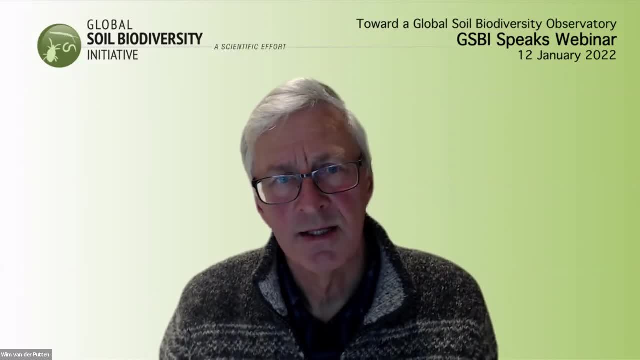 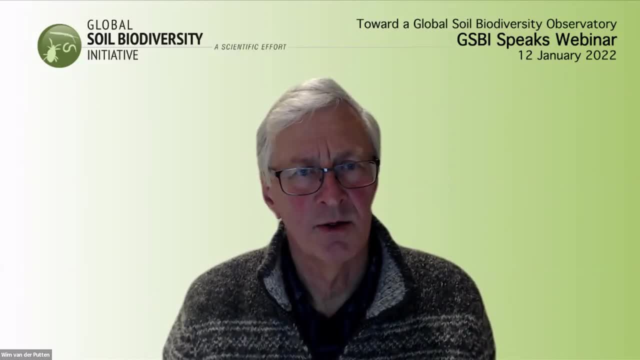 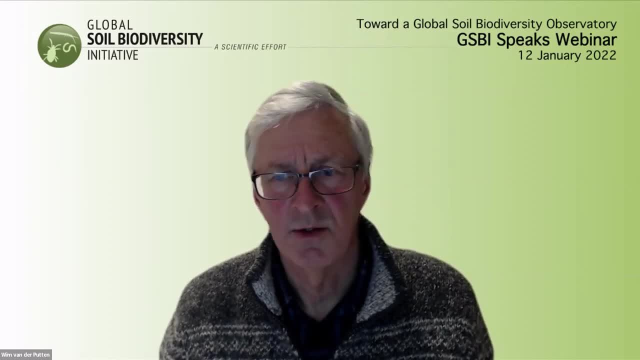 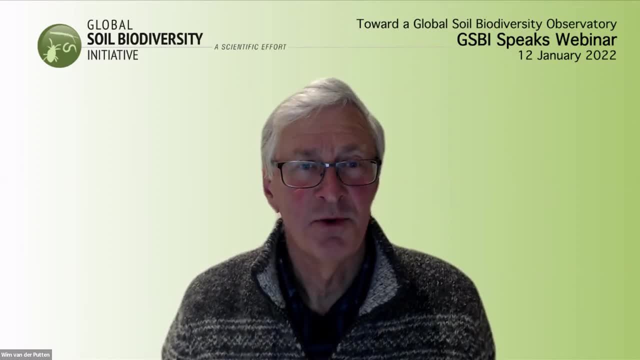 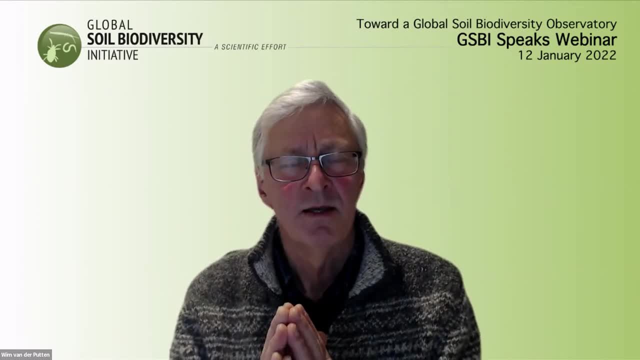 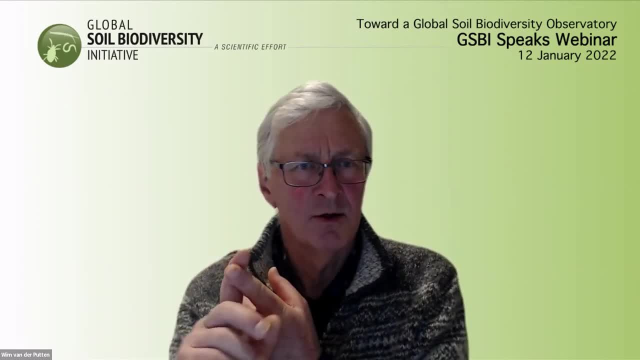 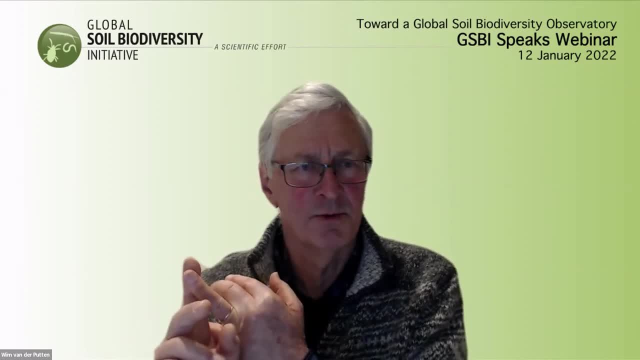 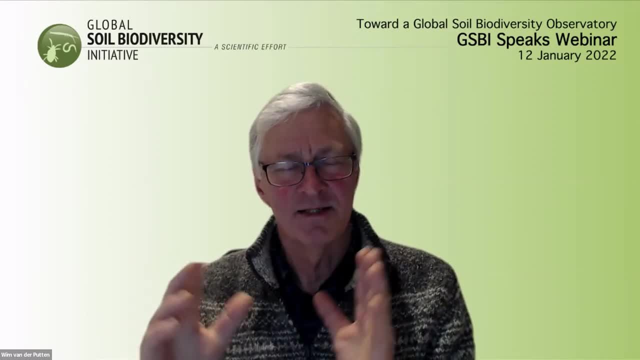 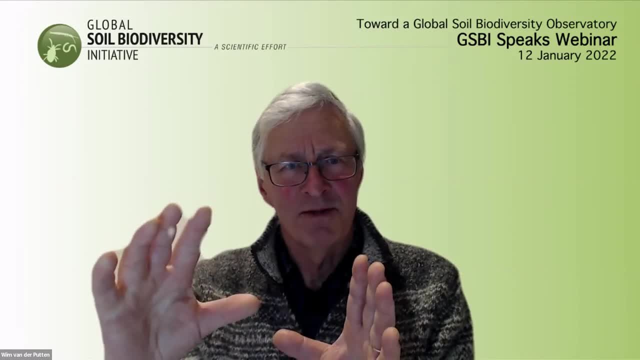 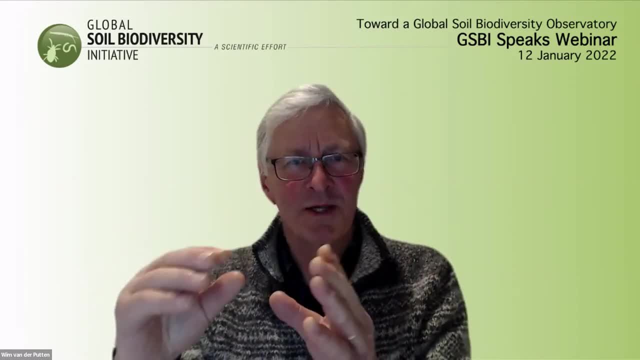 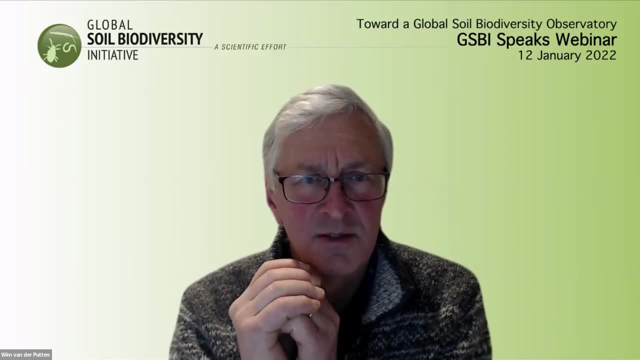 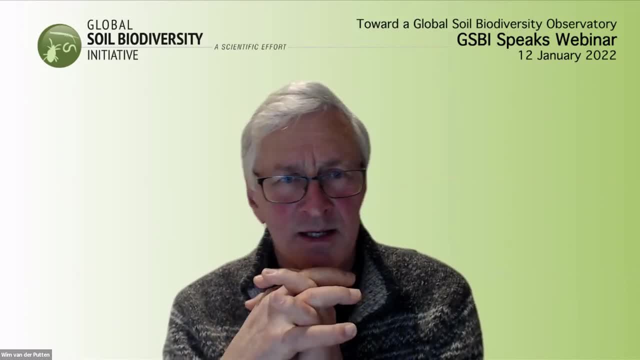 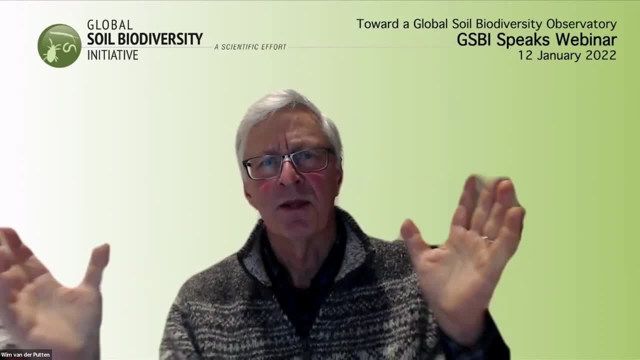 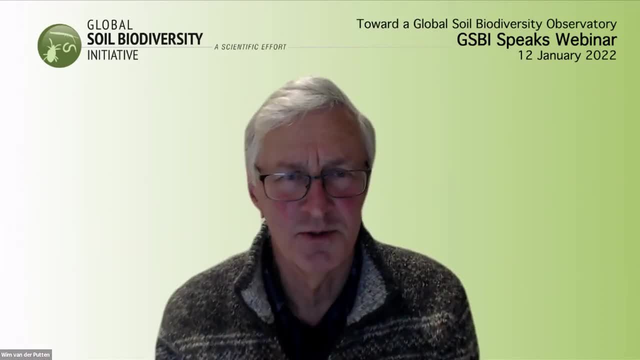 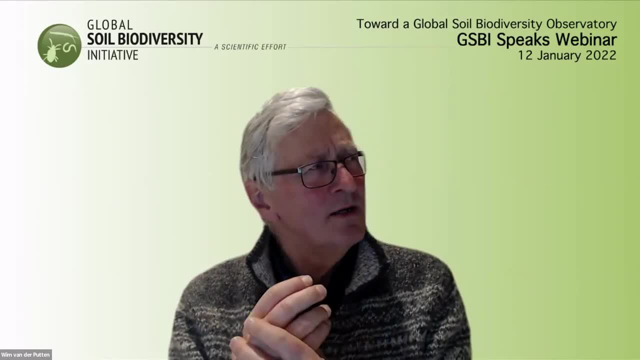 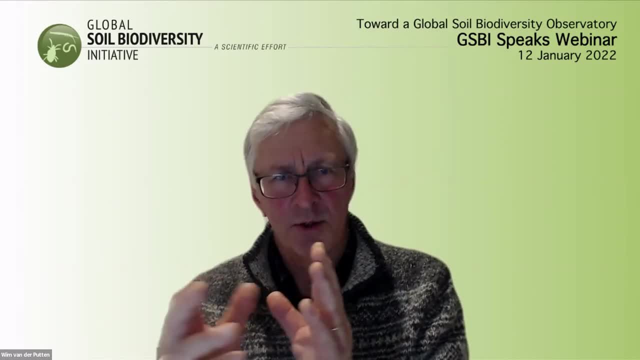 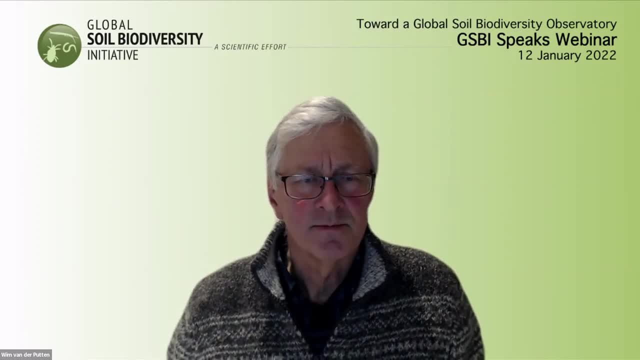 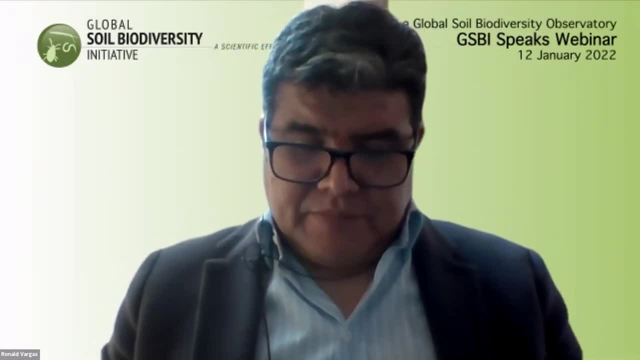 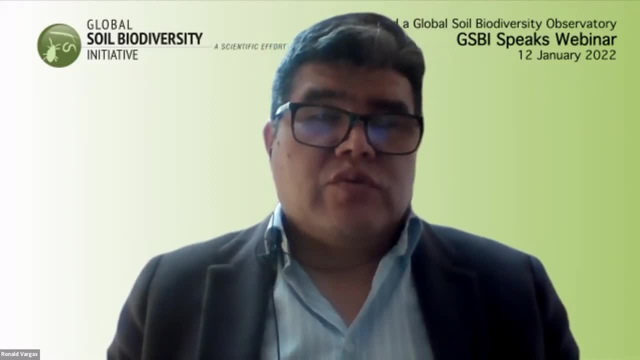 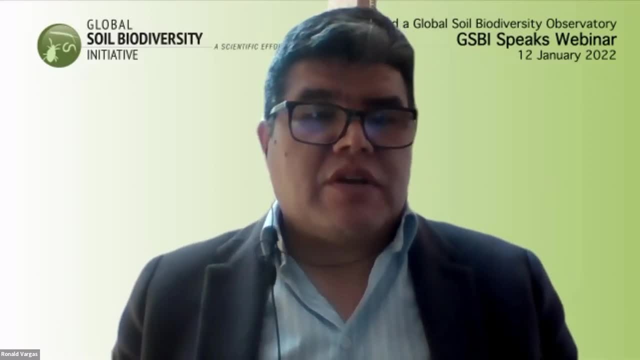 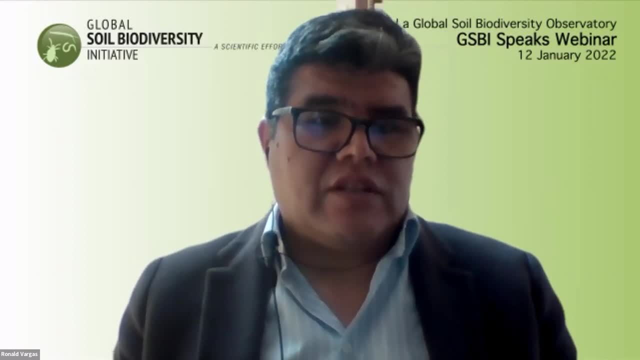 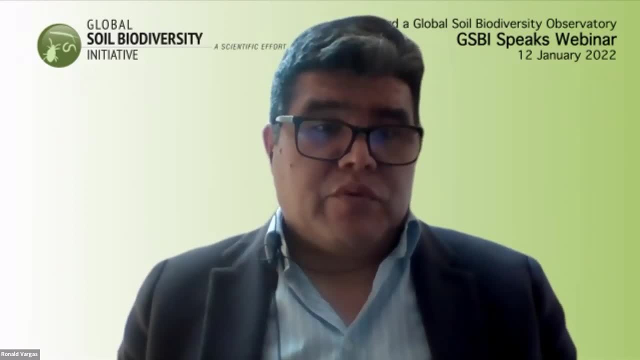 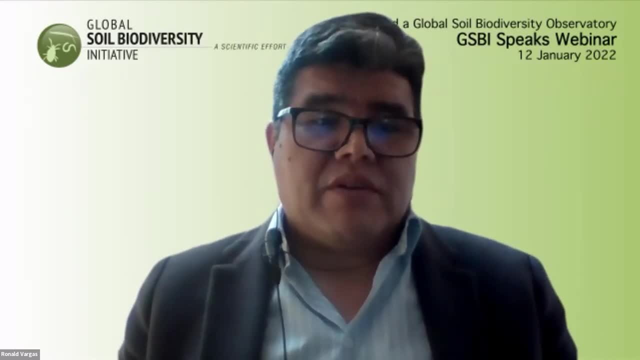 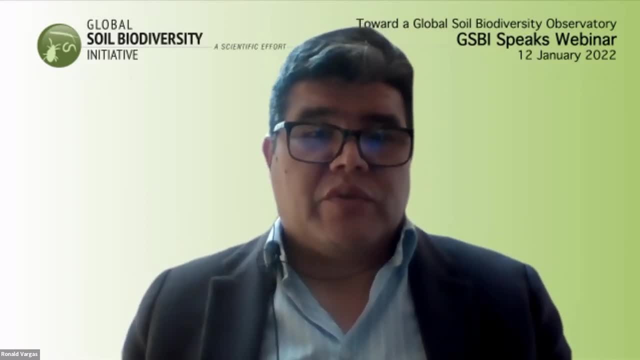 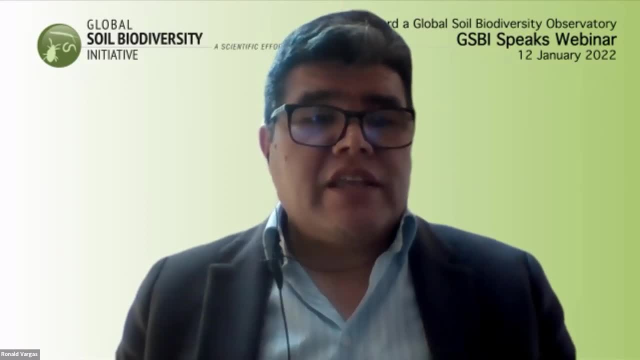 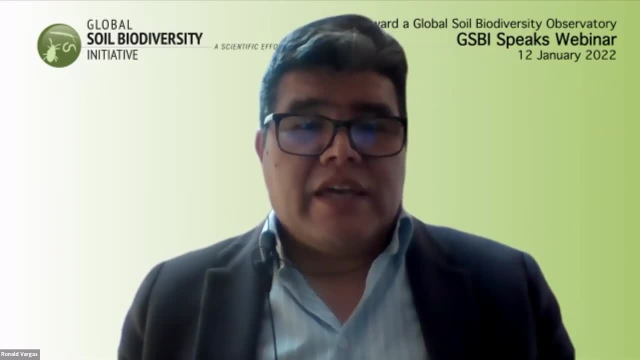 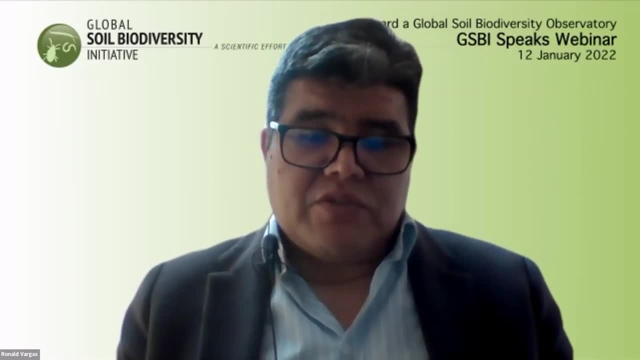 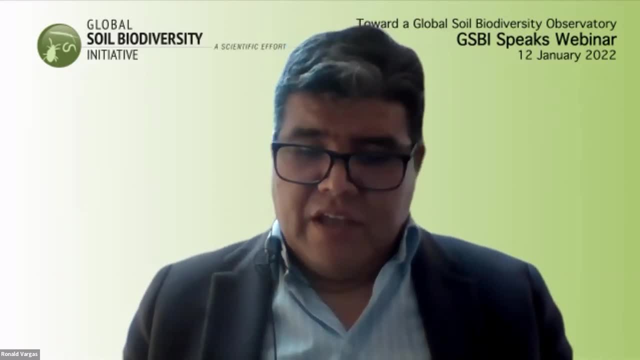 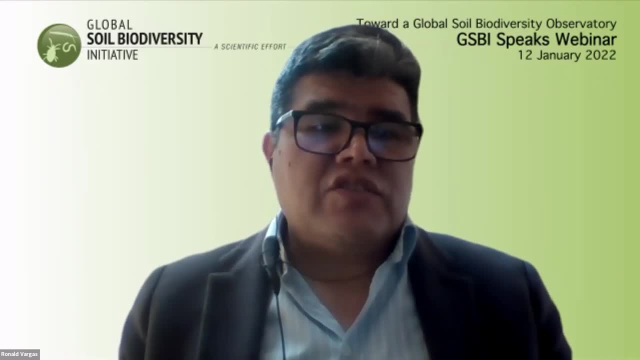 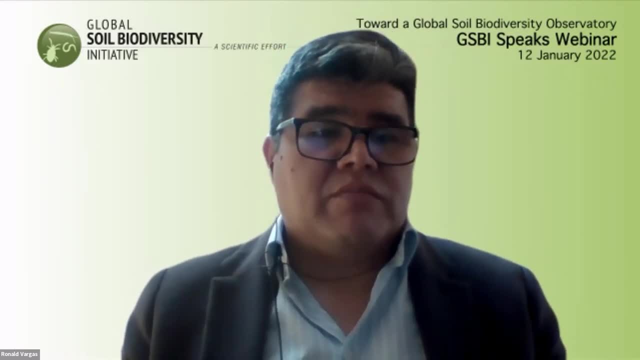 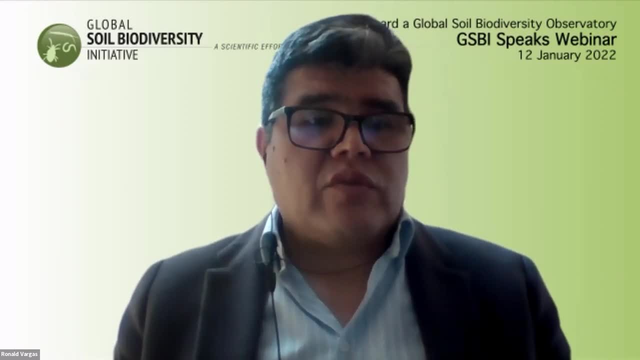 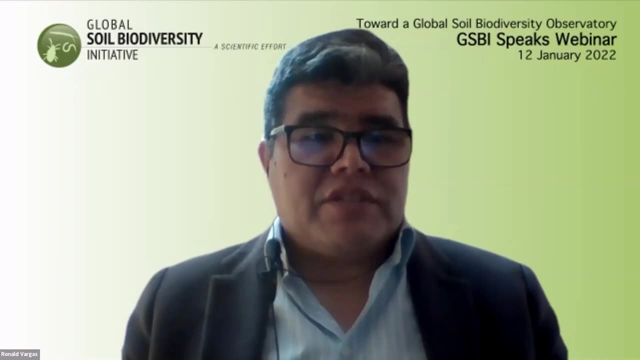 And for this we will try to get hotspots where we would like to have these measurements taking place. But in the long run, of course, we would like that countries get the ownership of that process and measurement, so that then they will be populating the key places with the most biodiversity. 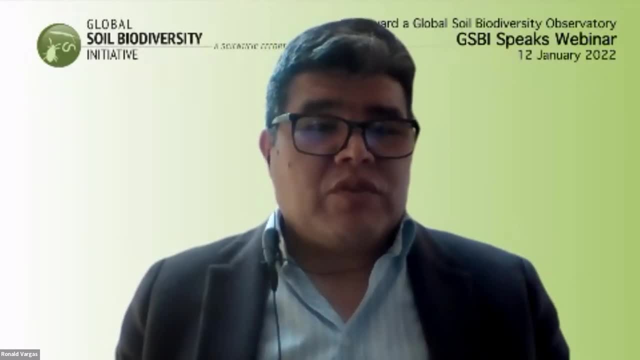 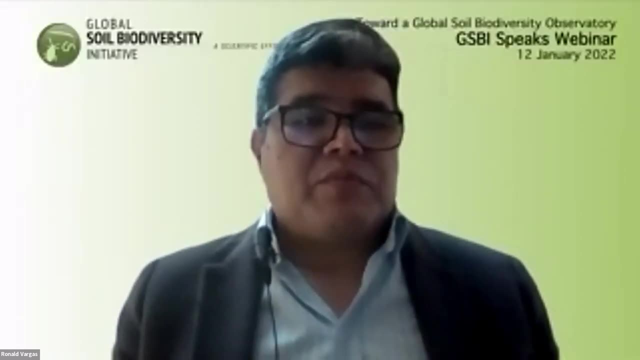 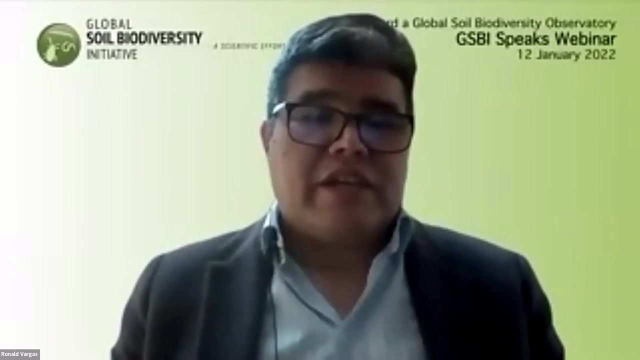 Now it is. look, the soil science community, of course, is a very important player in all this, But when talking about them, with them in different perspectives, it's quite difficult to get some agreement And the indicator thing can take you for years and I'm sure many will never reach agreement. 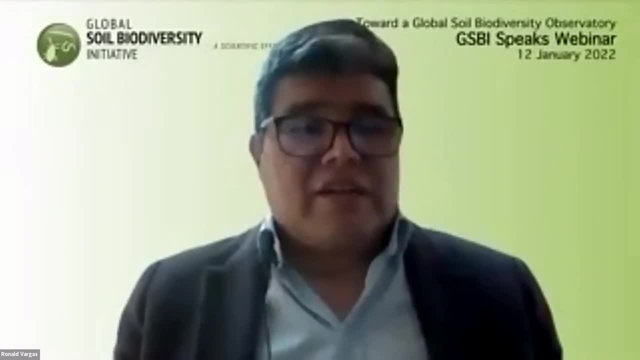 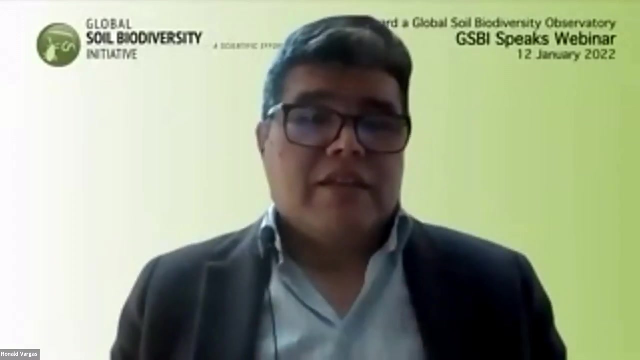 We reach agreement in FAO with three indicators to start with, But still I can tell you that when you talk about laboratories, the only thing that all agreed is that the pH- when soil pH is seven, is neutral. All the rest is very difficult that you get any agreement, even reference values to guide us, like you get some reference values when you do the blood test for humans, right? 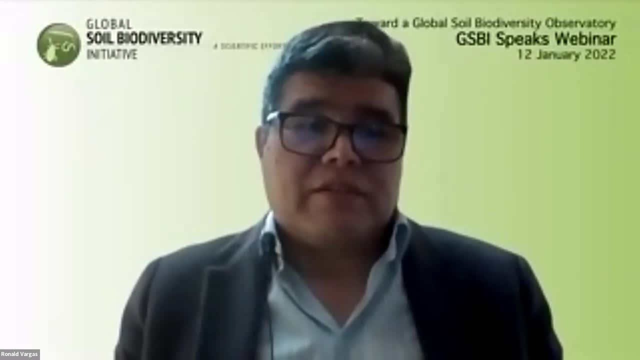 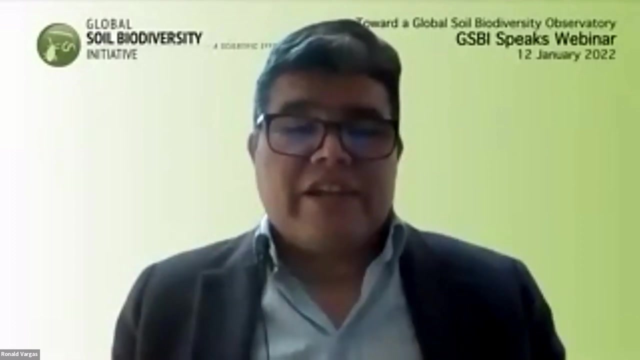 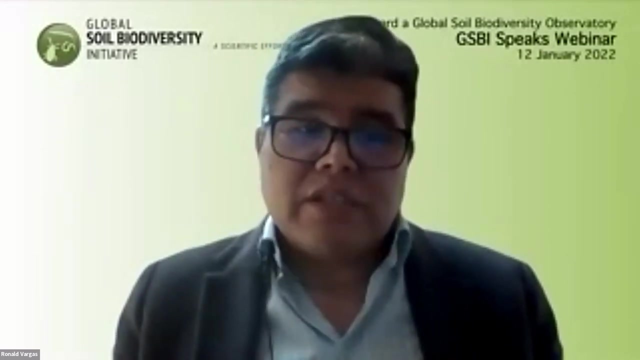 Some indications, But from soil science it's quite difficult because you always have the local variability in place. So sooner or later we need to come with some indication. We need to come up with some indicators that will help us to enter into this global definition of policies, because otherwise we are out. 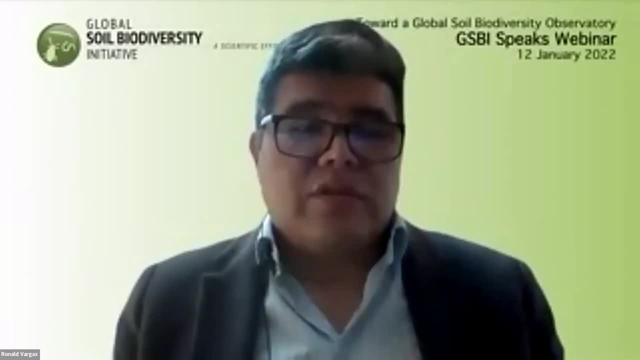 One example is the sustainable development goals. We fight a lot of time and we advocate for having soils more reflected, And the usual question was: that the statistics, national statistics systems? we're not having almost anything on soils, meaning that we were out. 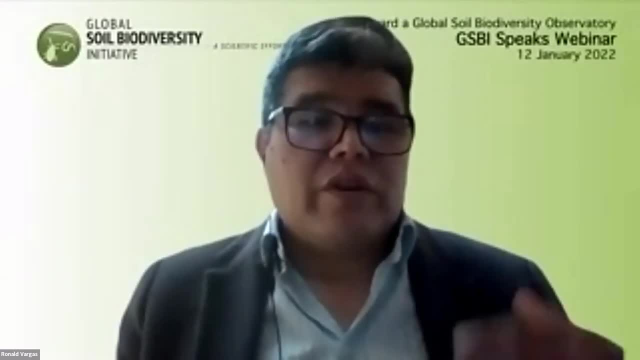 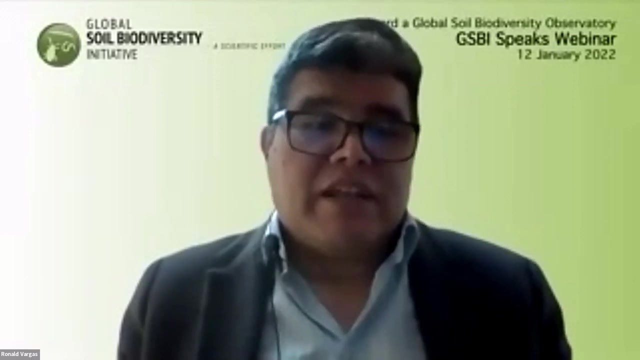 So we were not able to put policies or, let's say, any goal there, because we don't have the tools to measure and show progress. So sooner or later, we need to take a commitment, a compromise, and have something reflecting how soils can be considered. 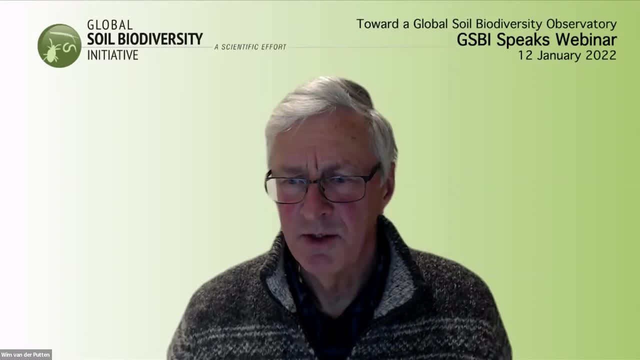 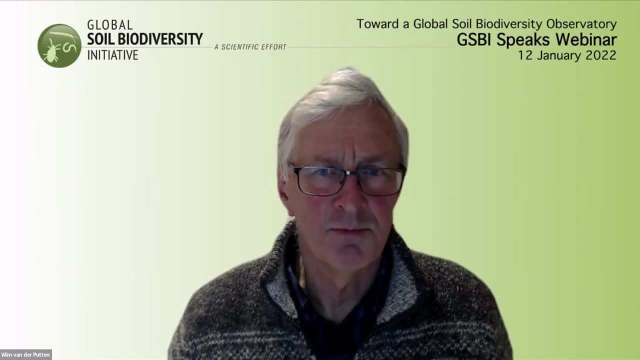 So sooner or later, we need to take a commitment, a compromise, and have something reflecting how soils can be considered Exactly. And Ed Bush also mentioned that there are five principles of soil health. Yeah, I think that the group here is quite aware of the principles. 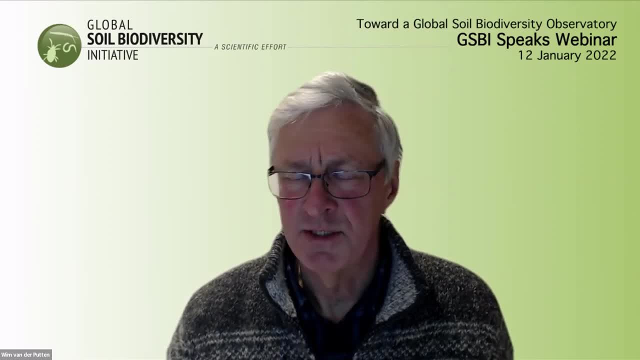 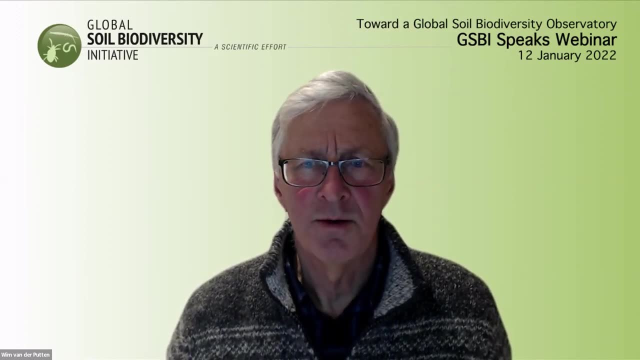 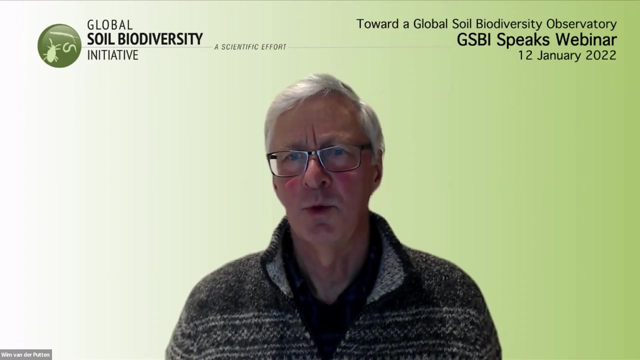 Ultimately, it comes down to how to apply the principles in policy and in management. So we have 12 minutes left, So I would like to ask each of you: where are we in five years from now? I will start with Diana. Where are we in five years from now? 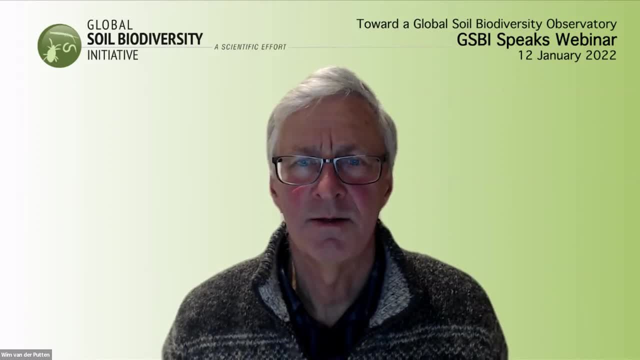 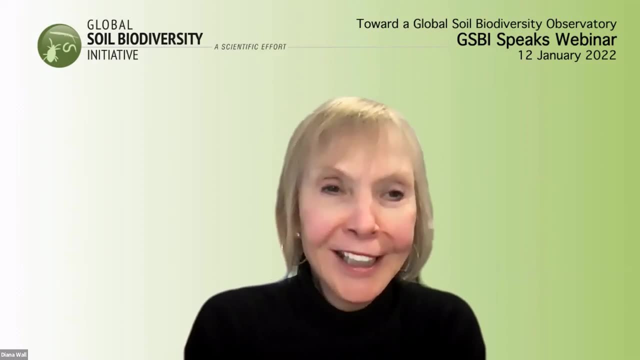 You have to unmute, Sorry. I think this has been absolutely fascinating because I'd like to you know. I'm optimistic at heart And I'd like to say that I would hope that we do have some resolution on a global observatory. 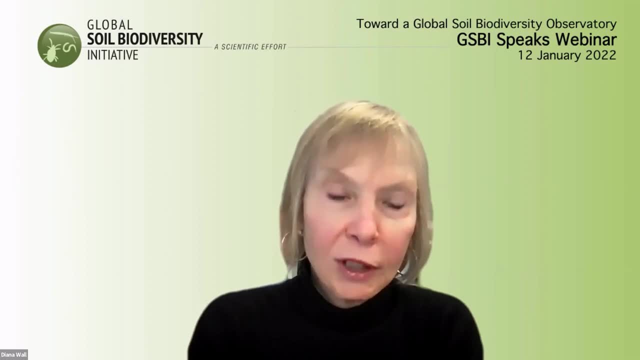 and perhaps the different types of laboratories in countries that would give us the information to include biodiversity and soils as part of overall biodiversity, Because I think to meet these global challenges, we need some measures that we can use very much like we use birds or snakes or bumblebees. 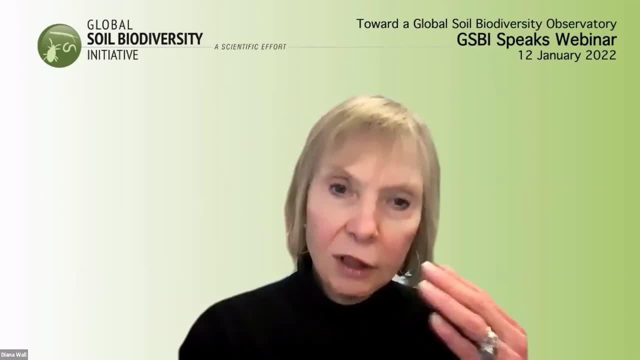 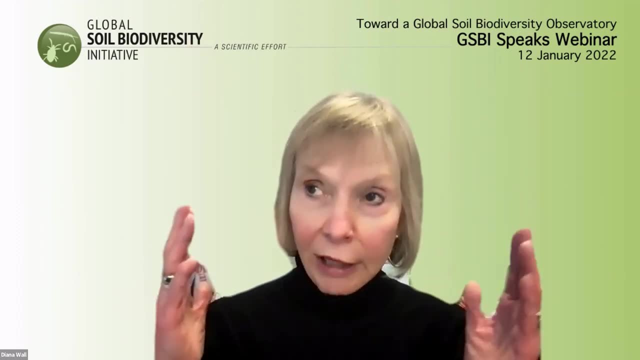 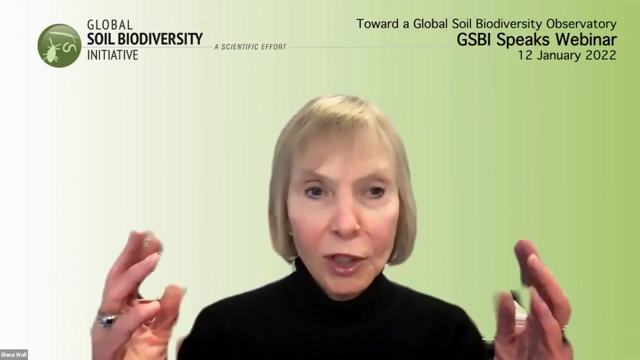 We need the same kind of indicators below ground, because it's not a blocked off piece of concrete, It's living and it interacts above ground. And if we're seeing all these global problems above ground, We as a community of scientists have to do the- as somebody mentioned, the magic word of 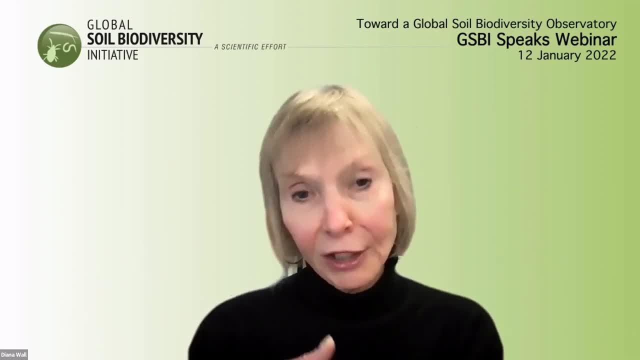 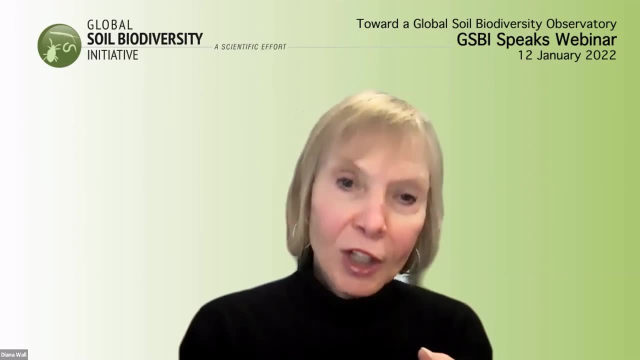 compromise, which in policy, can take years, but I think we have to be more urgent. So I would add: five years from now. we should be. we scientists should come to an agreement with stakeholders about what some of these markers are that we need. I think the other thing that's really important is: 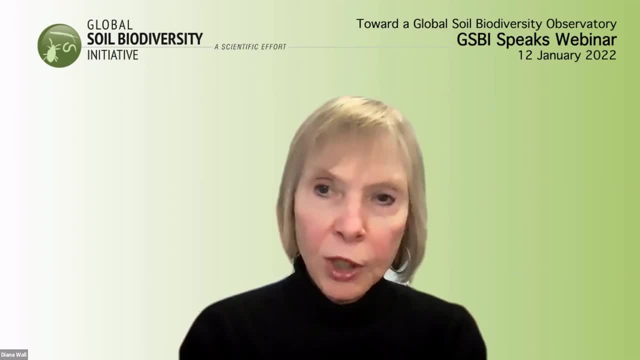 to go back to this topic that we talked about in building capacity in various areas of soil biodiversity, Again I want to say we have lots of disciplines involved. people who are entomologists, nematologists, you know, work only in the Arctic or work only in the desert. Many they're not aware. 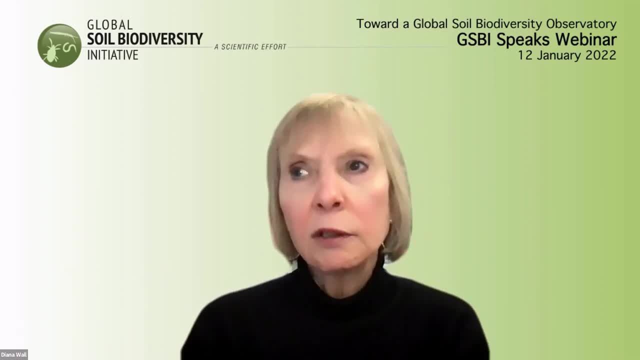 of necessarily all the policies that have to do with soil, but those disciplines need to talk and come together on where they think our contributions will help in training the future people working in biodiversity. that the soil biodiversity becomes more noted, I think that's really important, a long-term thing, And then I think, more interaction of the scientists. 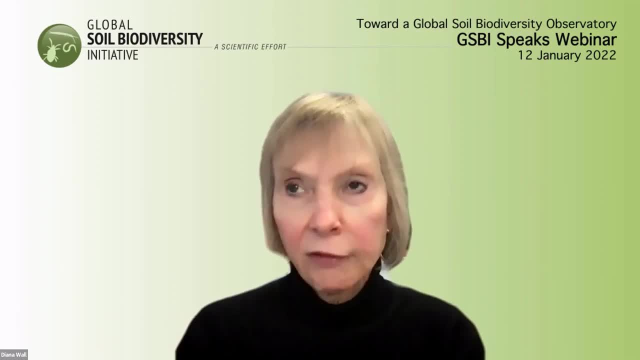 with the policymakers is really where it's all at. If the scientists sit back and say, oh, they can argue about this, I don't want to contribute, then we're dead. Okay, Luca, where are we in five years from now? 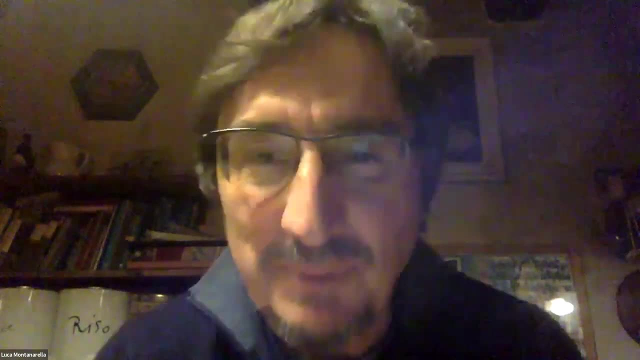 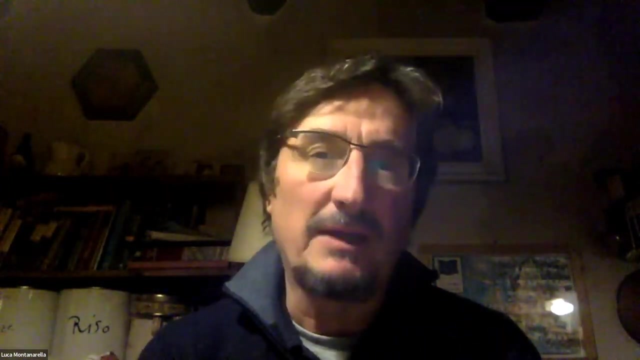 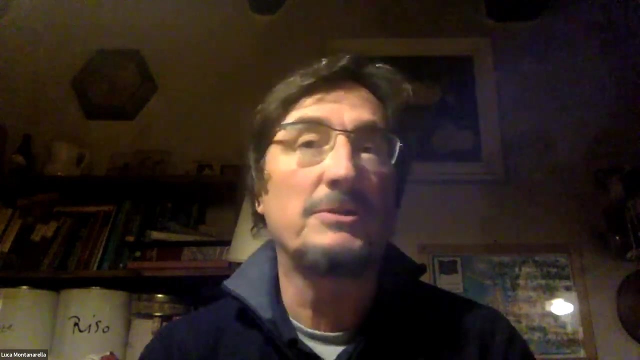 That's difficult to say. I can tell you what I hope we will be in five years from now, And I can tell you- I'm pretty confident- that in five years from now in the EU we will have a binding legal agreement which will be the soil health law. That, for me, would be a major breakthrough. 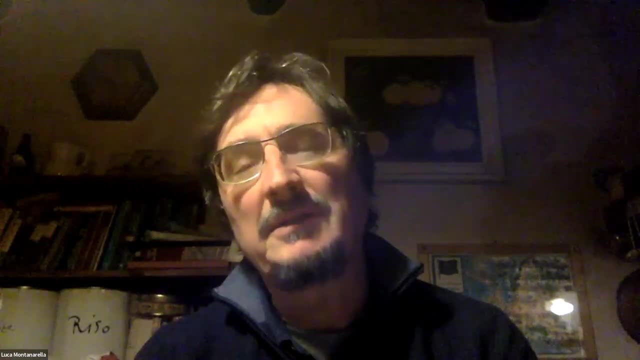 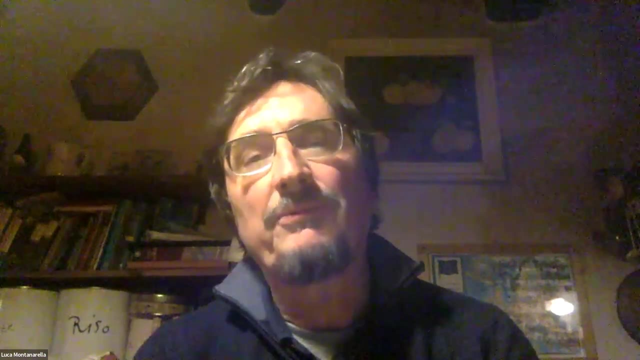 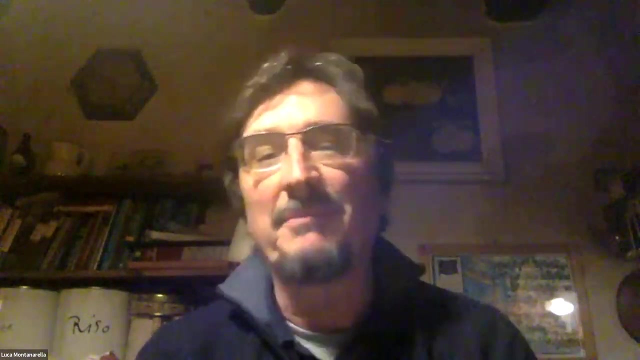 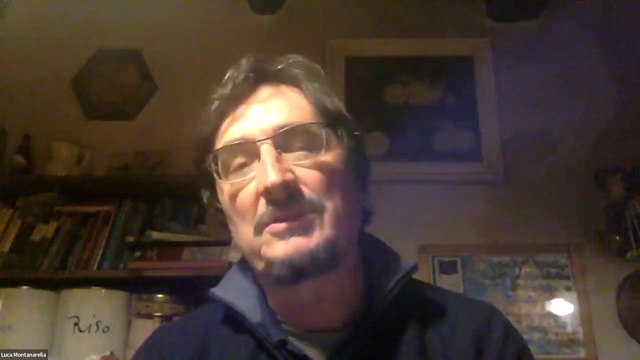 For the simple reason, as Ronald was saying, that the EU is somehow setting the example, And if we achieve that for other countries, we can achieve that maybe also for the hundred and more countries that are members of FAO. So because advocating that soil health is something that goes beyond the national. 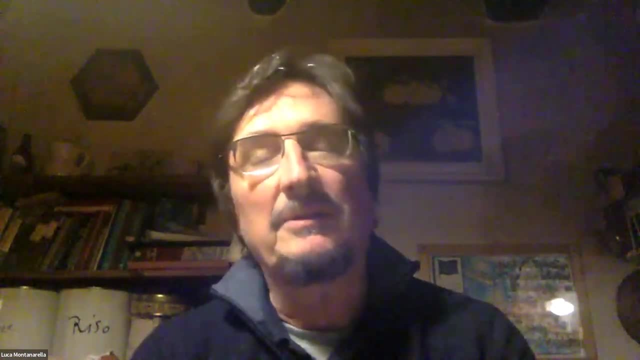 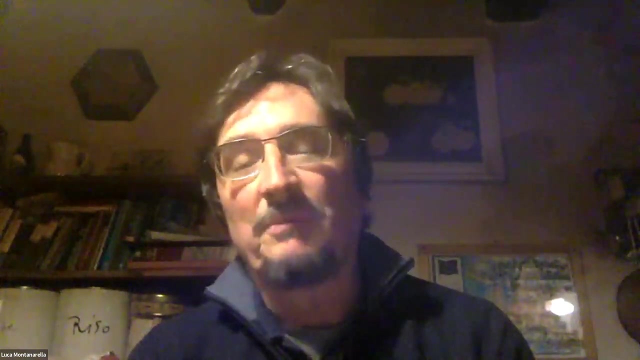 borders is something that is very difficult to explain to policymakers, But if we succeed in that, that will be a major breakthrough And I'm confident this time it could go better than the last time At global scale. I can only hope that this global observatory will. 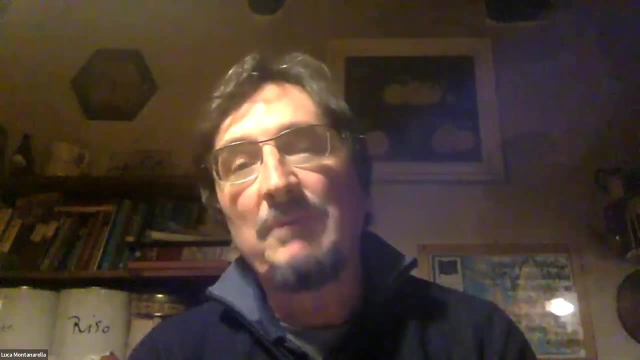 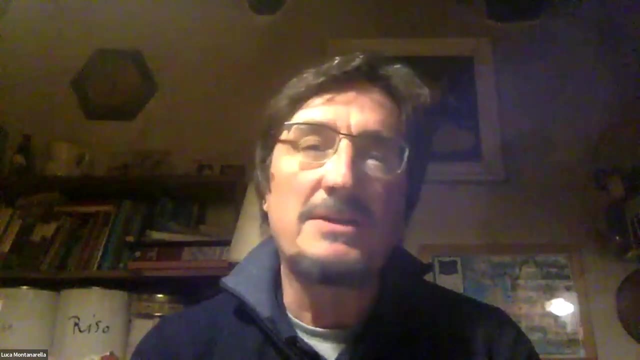 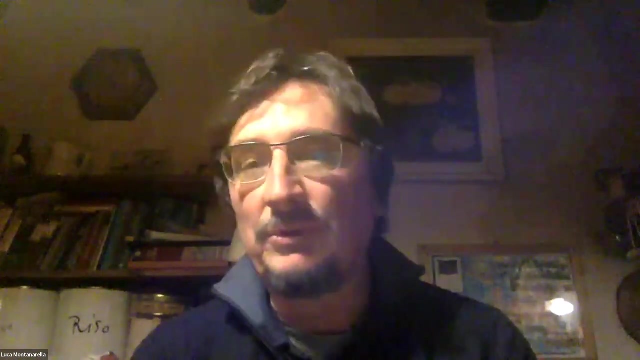 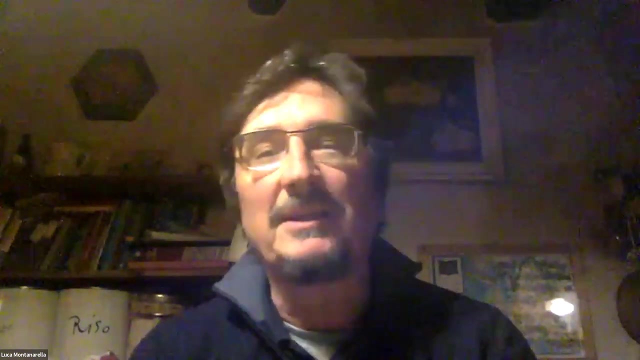 be operational in five years' time and that it will be participatory. I mean, that's what I think. it's really what I think is crucial. And participatory means not doing metagenomics and high-tech, super fancy Observations like we do in the EU. Participatory means what to me? for example, something like 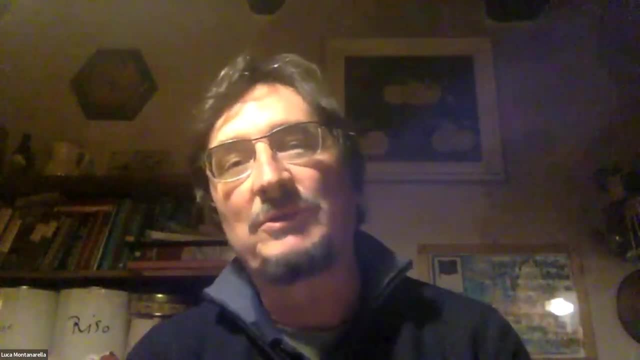 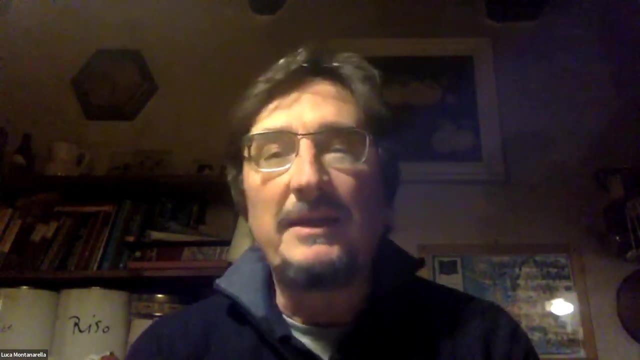 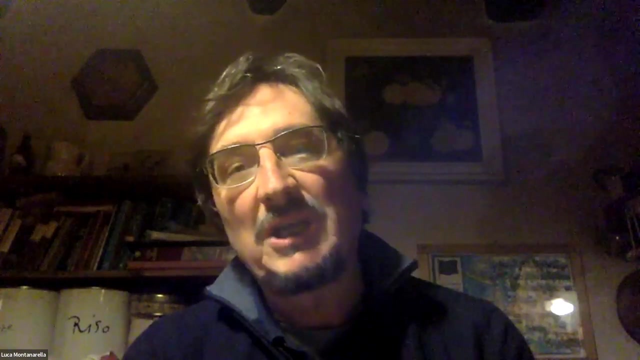 the warm watch program in Canada. I don't know if you're familiar with that. To me that was fascinating. A school kids-based program across all Canada where school kids were going out in the field and counting earthworms- This type of things which seem maybe not so scientific and a 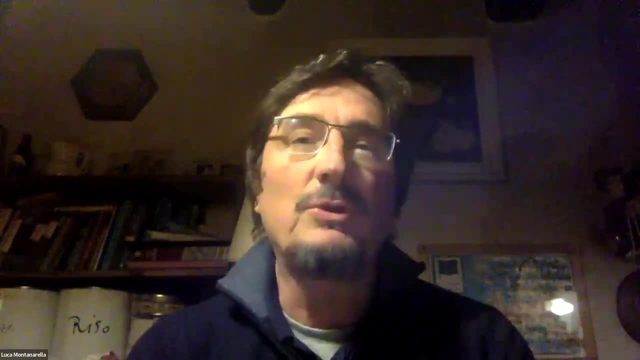 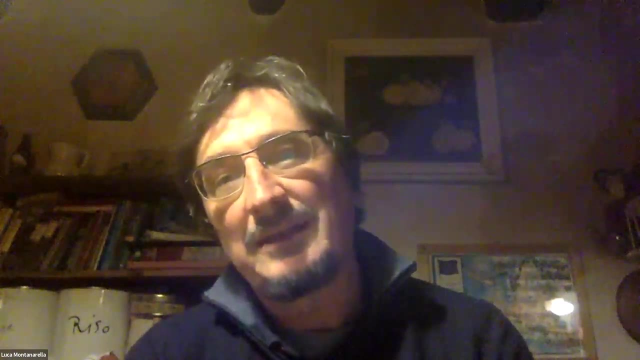 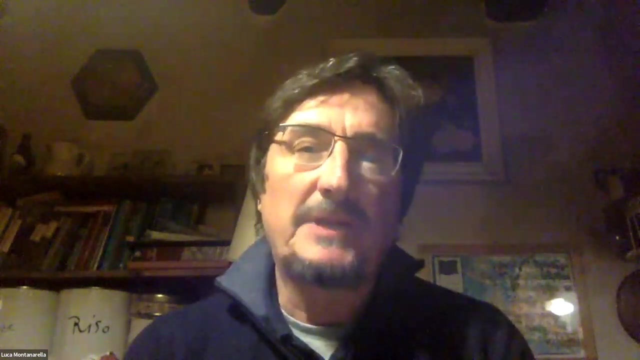 bit trivial to many of us, I think would make a difference, Because doing that type of things when you are a kid brings you close to soil, brings you close to soil biodiversity, And these are the things I would advocate the Global Soil Biodiversity Observatory should strive for: So simple testing that can be done by everybody. 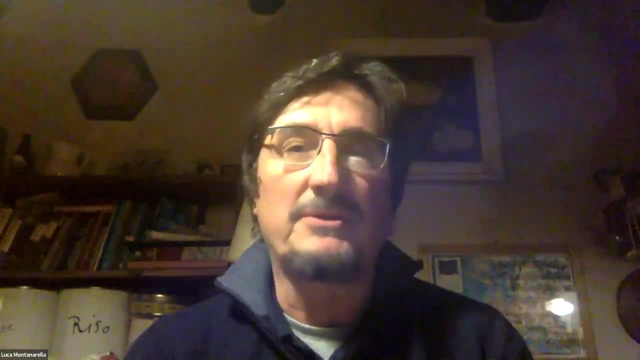 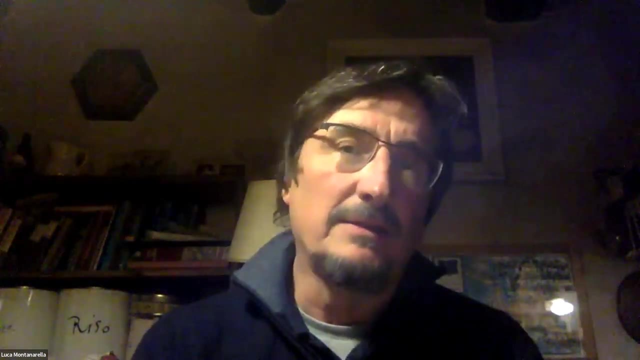 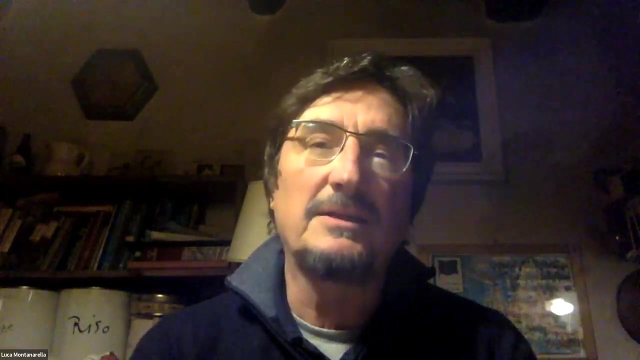 in the field at global scale, That would be a major breakthrough. Very simple things- Counting earthworms or whatever That thing FAO can do- because it doesn't require huge financial efforts. And I think there, I think, we are counting. 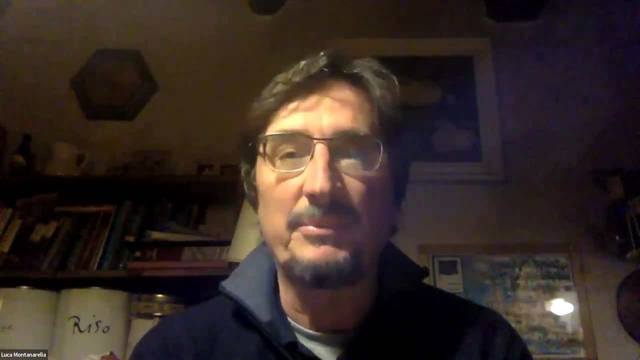 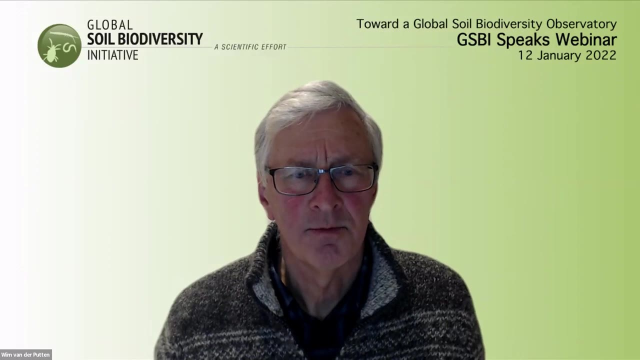 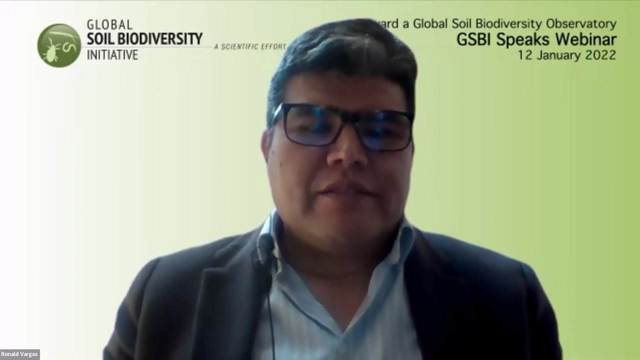 very much on the Global Soil Partnership to take this up and take the lead on that. Thank you Nice, Ronald. Well, I'm very optimistic because, well, I believe that soils didn't get much attention as they are currently getting. So this is the basis And I'm confident that all colleagues 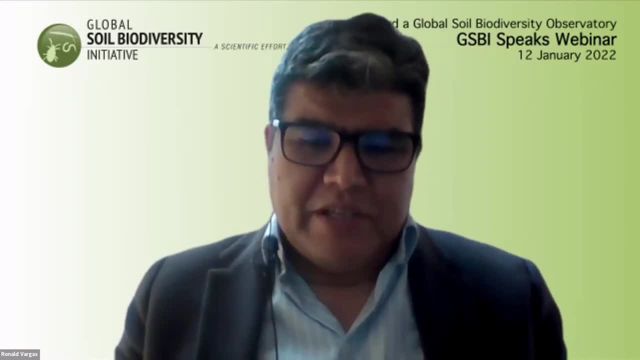 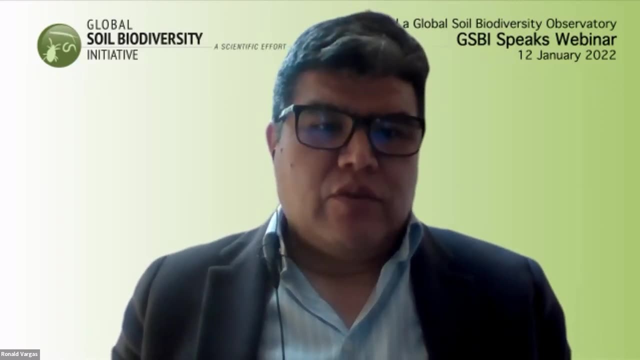 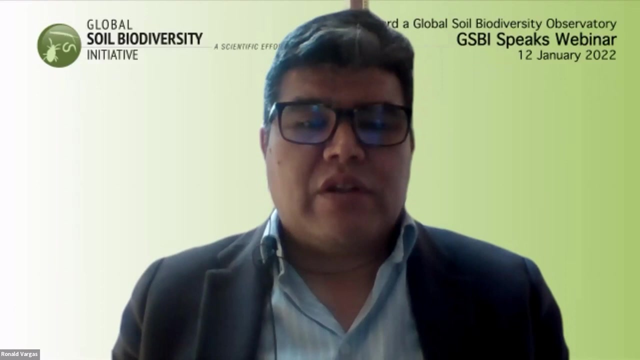 working on soils like all of that are present here today, are working hard in order to really materialize all this soil fashion that we have now. So in five years, I see and I can tell you that we will have the Global Soil Observatory, Soil Biodiversity Observatory. 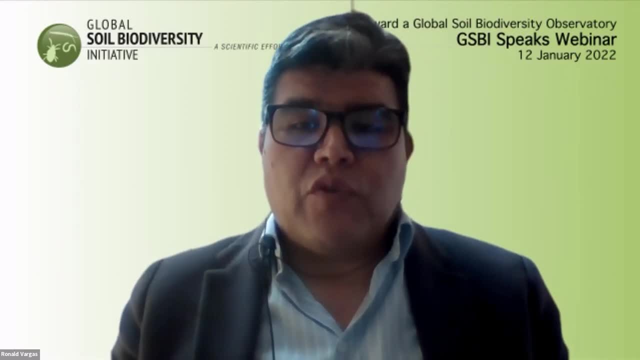 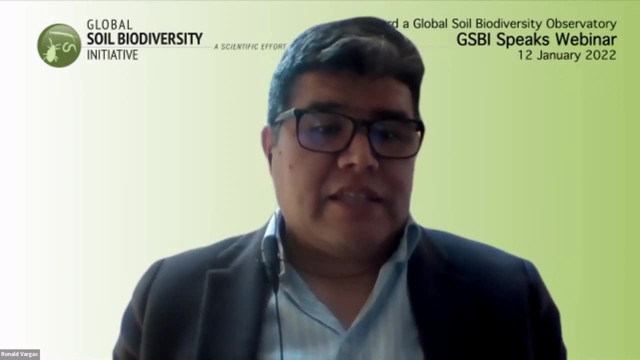 Observatory running And, of course, as Luca said, the participatory approach is fundamental And that's why we are really facilitating this And we want to have ideas from all of you, like this one that Luca mentioned, in order to really have this observatory running and, let's say, having 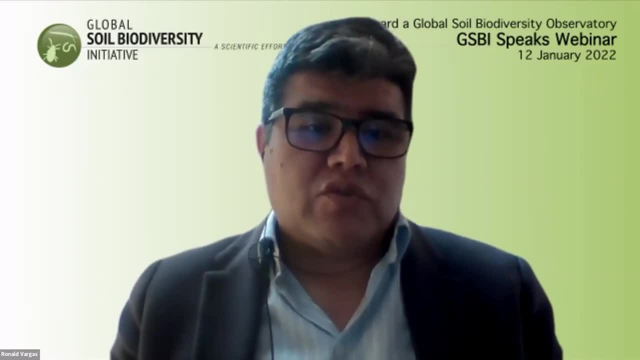 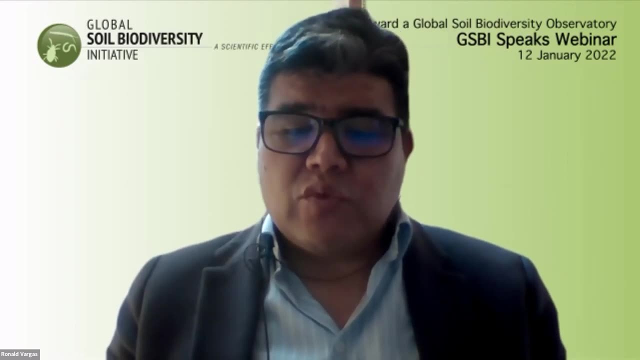 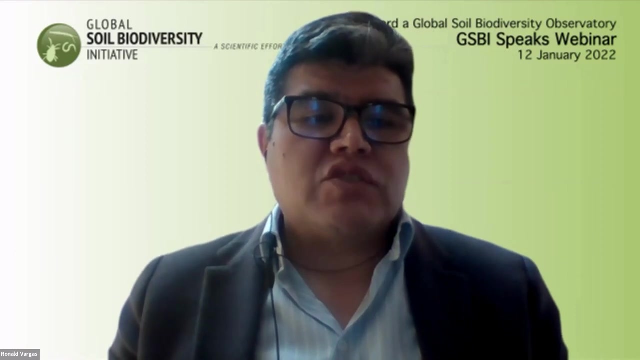 ownership by all. That is something very important because otherwise an observatory by few will not work. I also see that in five years' time we are working towards something to have some soil binding mechanism. So we are working towards the institutionalization of the Global Soil. 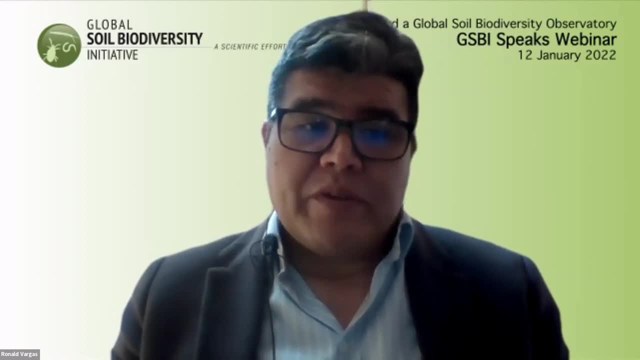 Partnership so that it becomes something binding. I hope it will fly. I think there is quite good support, But also we are building our own framework, action framework for the next 10 years, And in there you will see that this is quite ambitious And I'm sure that in 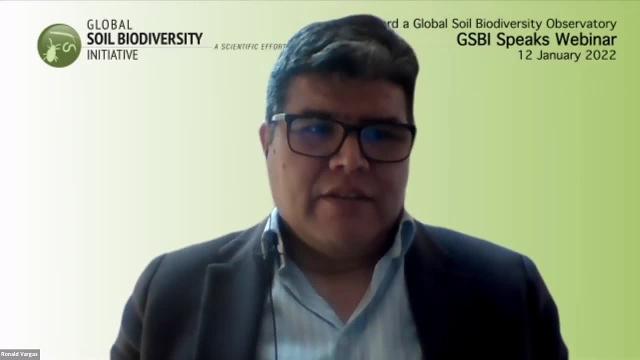 five years' time we will have at least half of the policymakers on board in supporting something like this commitment. So I see that in five years, soils will be having this attention materialized in concrete commitments. So I really hope that we will have this commitment. 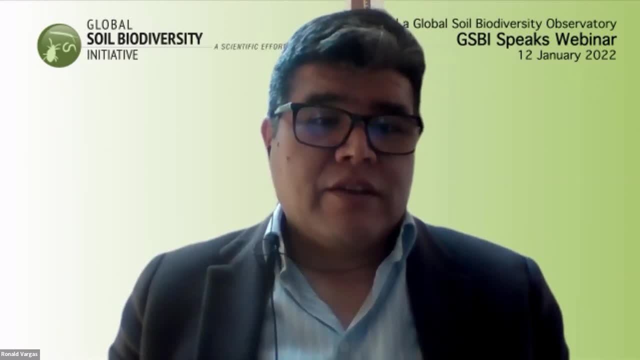 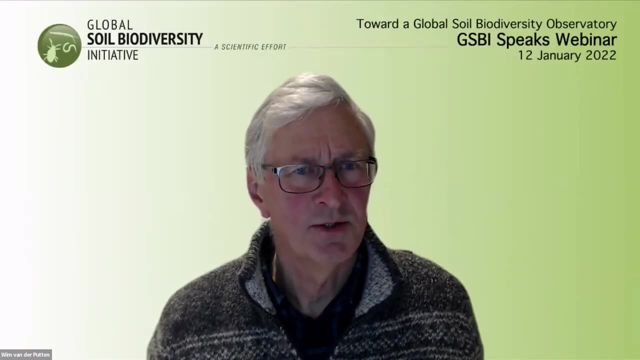 I will not be mistaken, but let's see, in five years, hopefully, if we all are here. Thank you, And the last word is for Carlos. You're the younger one here, Carlos. So what is? Yeah, You may say 10 years, but five years is longer. 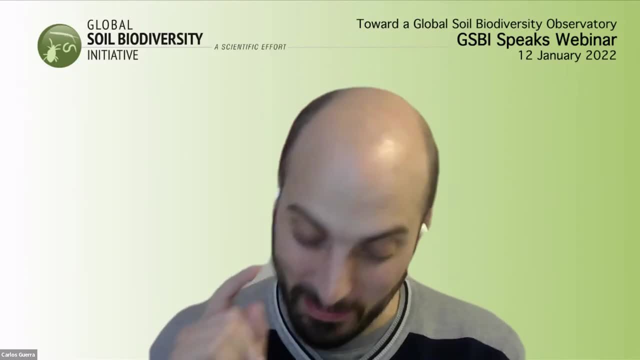 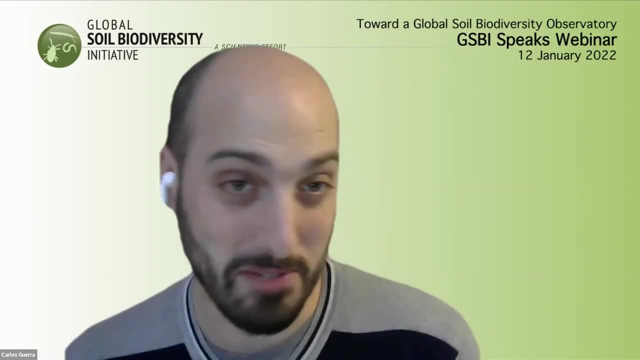 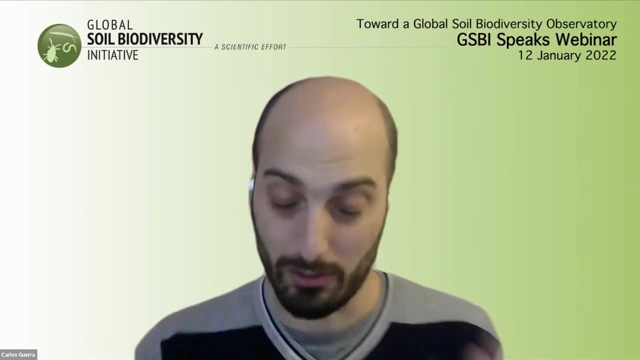 I can say all those five years, And I want to start by saying that Honnold was saying that the dream was. And then he said something, Maybe because I'm younger, because I'm more naive, but I believe in the dream And I really believe in the capacity of people and of us here. 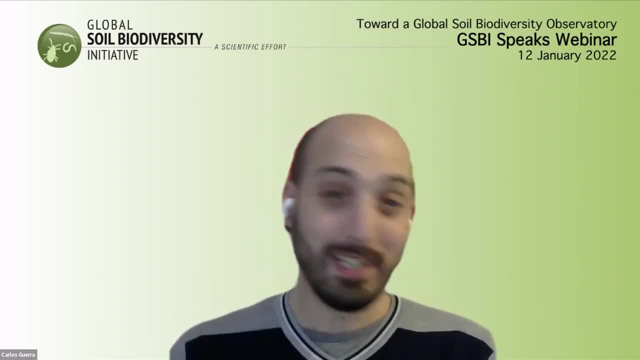 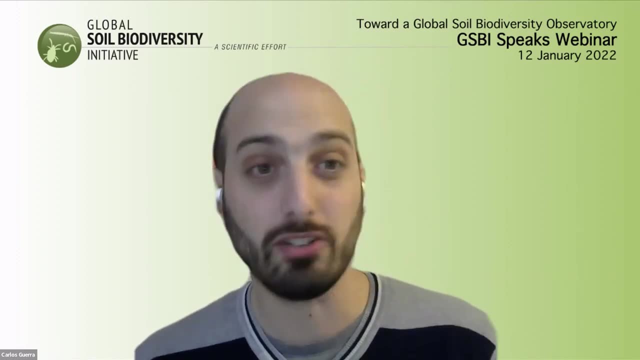 and other people across the world to implement this in a real way. So for me, in five years' time, I would like to have temporal analysis of soil biodiversity. We will get that already in the EU, but this would be an achievement, for example, for SoilOne. Within SoilOne. we aim also for that. 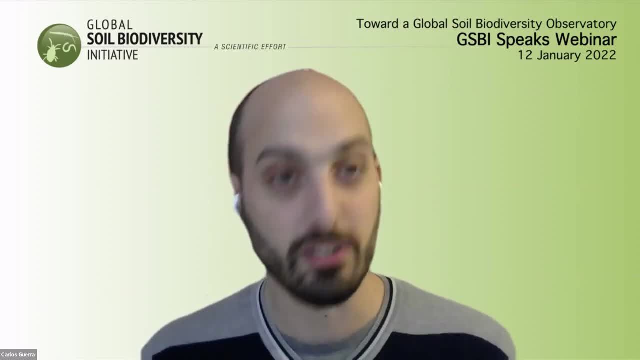 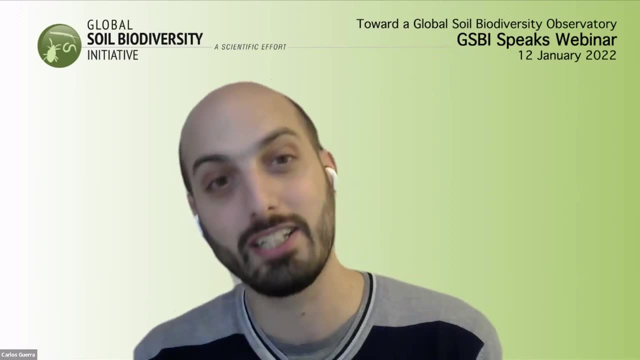 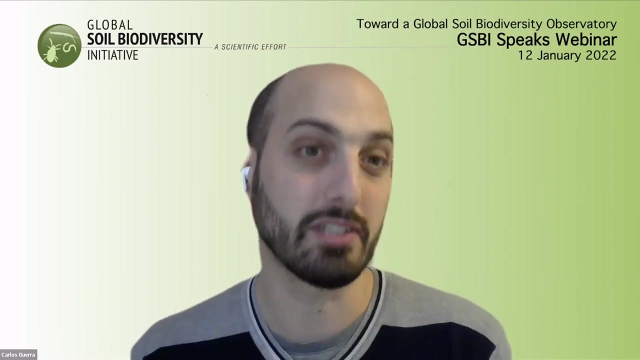 and this would be something to consider. This would be a very important outcome for me in five years, Then I would honestly would like to have more and better representation of the developing world, to overcome some of the barriers that we have at the moment to for. 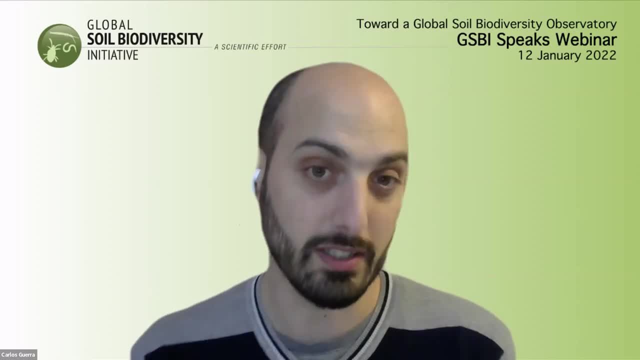 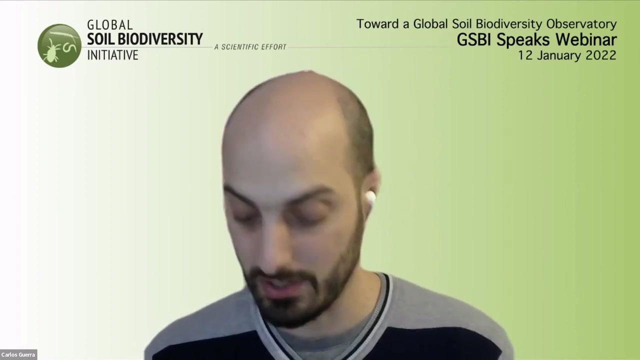 example with the support of the JRC or from FAO, to provide, for example, direct funding for developing countries, that they can also interact directly with us and provide their own contributions, their own knowledge and expertise to this type of questions. Yeah, 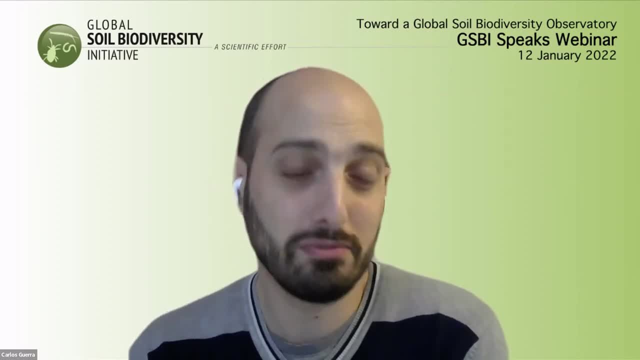 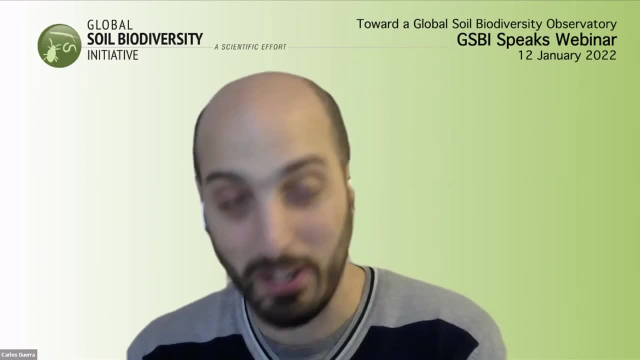 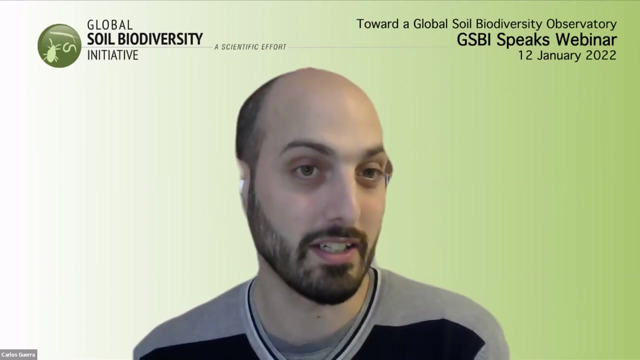 Then, a very objective thing: I would like to have five apart from the EU and the US and Canada. I would like to have five national soil biodiversity monitoring systems implemented, And if we can have that as a start-up, this would be already an achievement for me. And finally, 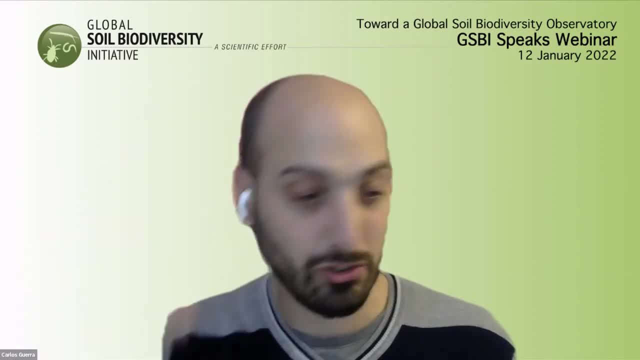 I would like to have, at least within SoilOne. SoilOne is not a project of me and Diana, it's a project of more than 500 people. Yeah, Yeah, Yeah, At least. 500 people have 500 different ideas of what they can do and what they want to do with. 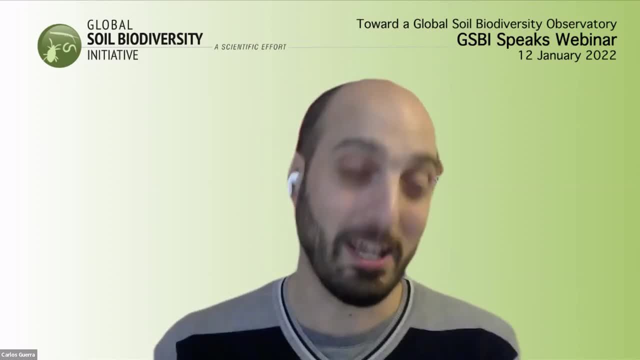 this type of information. So in five years' time, I don't want to have 500 different ideas, but I would like to have 20% of those people developing their own ideas and developing their own projects under the scope of SoilOne, And that would be me, Thank you. 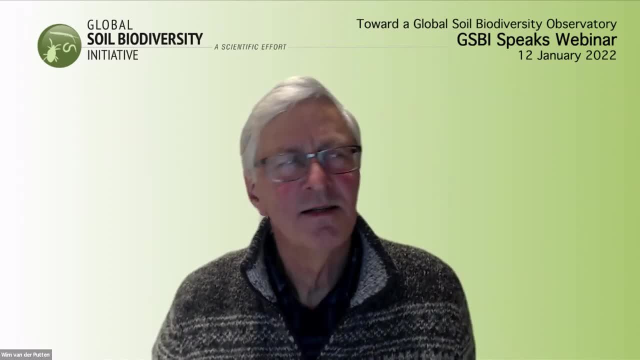 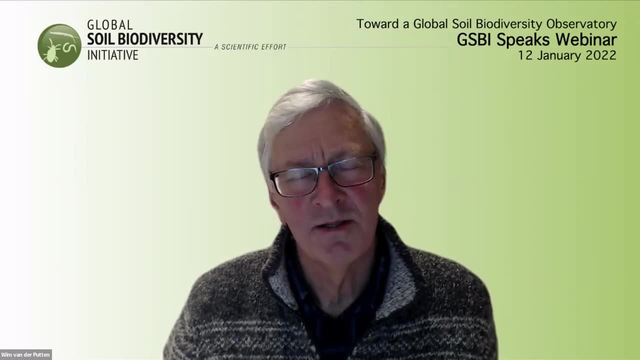 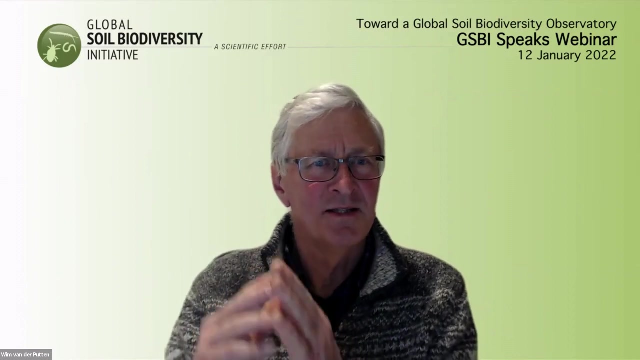 That's super, Yeah. this latter point also touches to something that I would like us to to say is we are really good in as soil ecologists or scientists in general, to show that every time we make a finding, that it is a novel finding, and that's also the way. 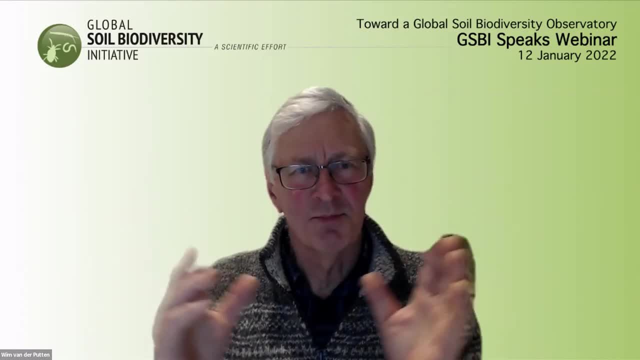 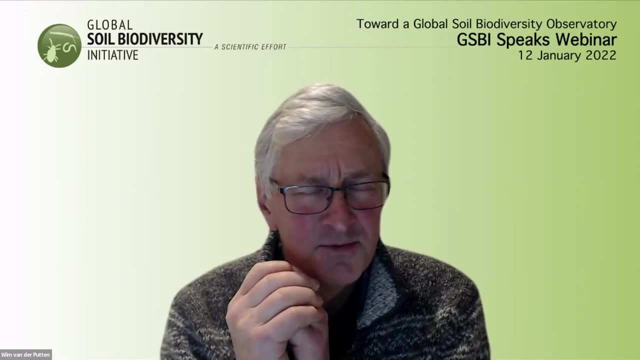 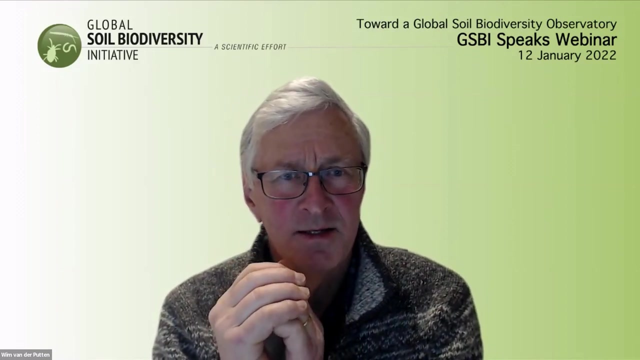 you get into the higher impact journals and so all novel things, but this gives a very scattered perspective of our work. And so what? I hope? that in five years from now, that we sort of, towards the outer world, show that we agree on certain things, and uh. 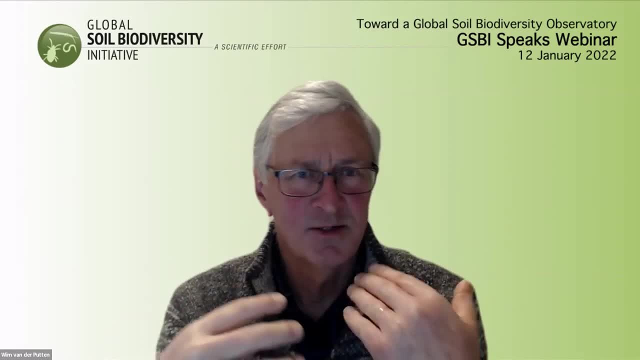 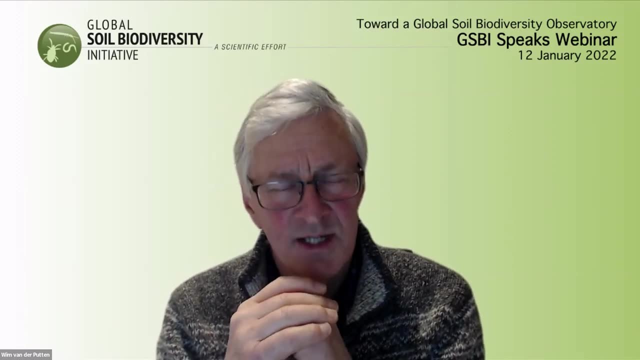 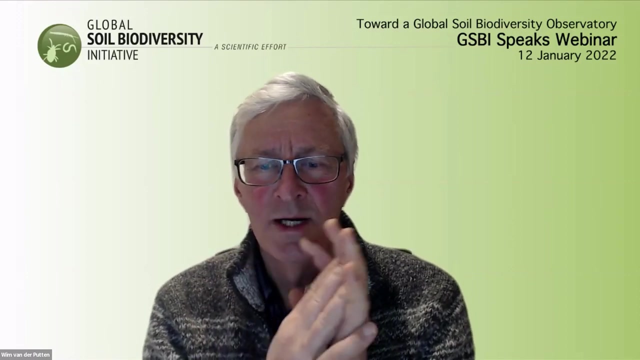 So within the field, we might say, OK, we disagree, or so, but towards the outer world, we should come up with a message which is understandable and which is coherent, And I think we have that. but we are very much trained to show the differences and not to show the convergences. 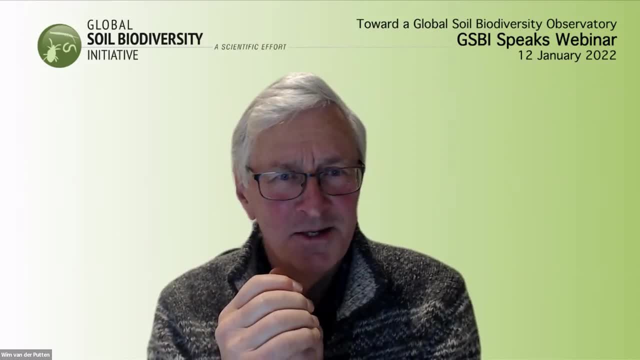 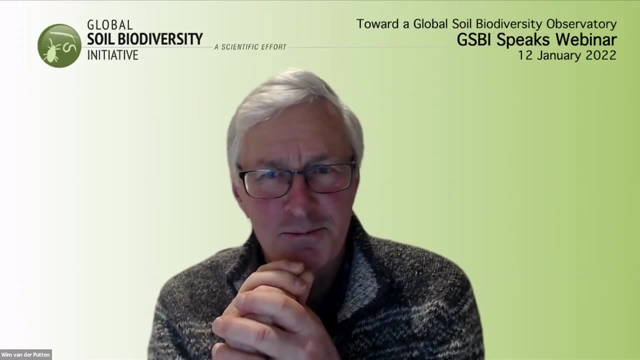 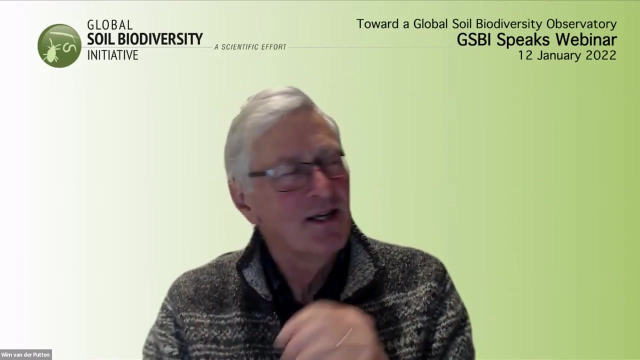 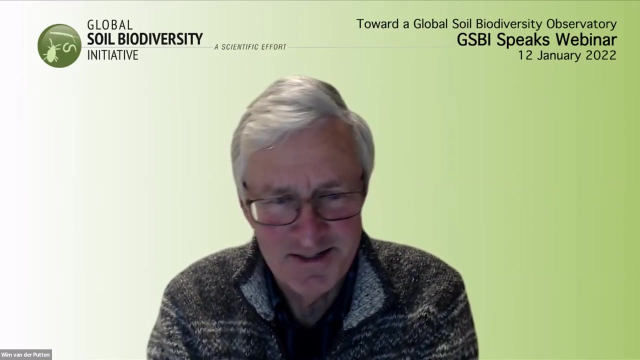 The other thing is that I hope that my country is not a country voting against a soil directive or a soil law in Europe, So we have lost one European country voting against this law. But if I can do something to motivate the people in the Netherlands to vote for and not against, I will do that, Luca. 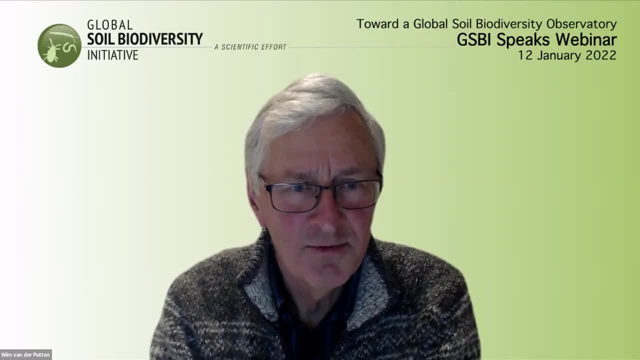 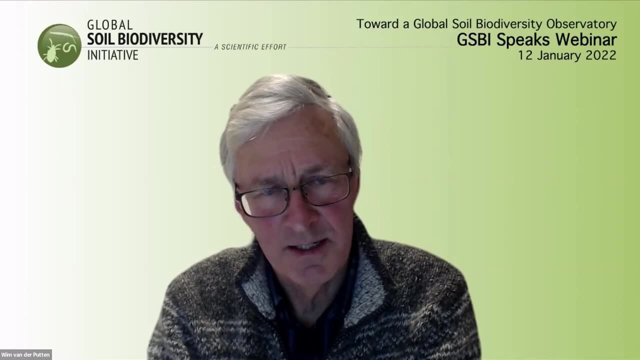 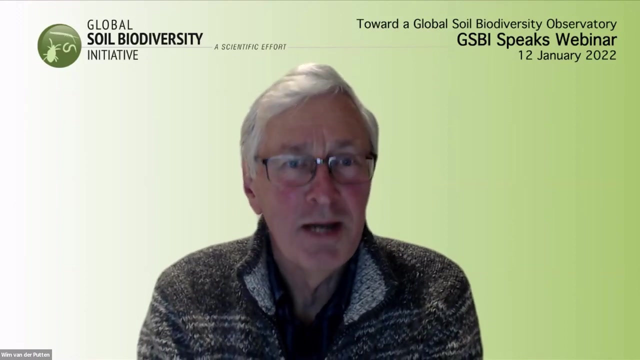 And, for the rest, I hope that in five years from now, we have this Soil observatory network installed and this, and that this enables cross talk between scientists and and farmers and landowners, and that we will just have a more happy soils worldwide, because this is what we need.